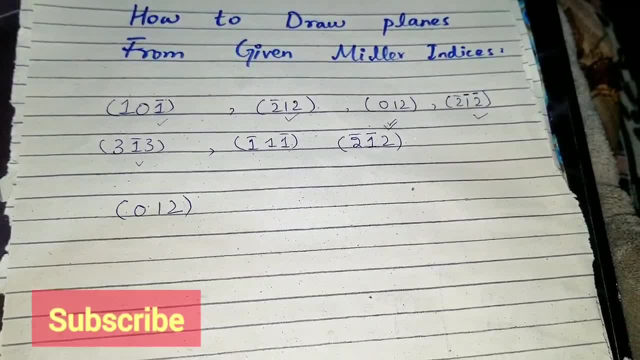 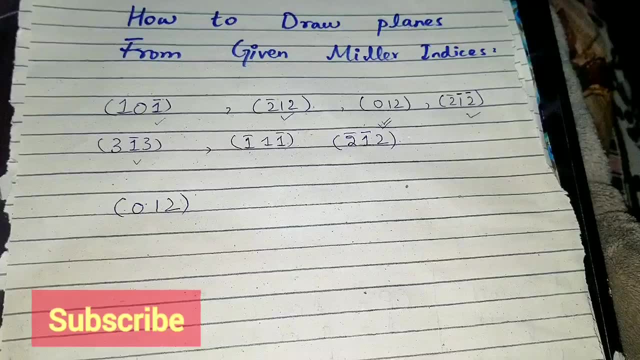 Miller indices of planes is also uploaded in English version as well as in Urdu and Hindi version, So you can check out the playlist. I have separately made the playlist for the English version videos and also for the Urdu version videos, So you can check it out in. 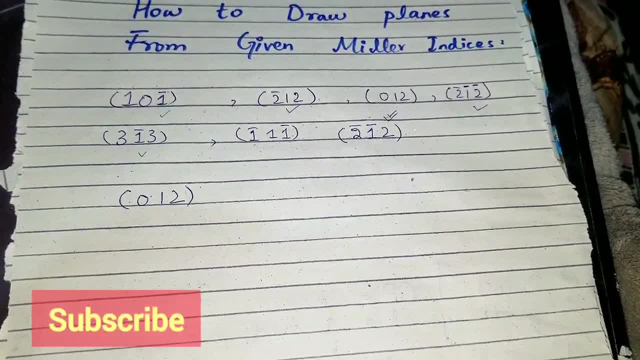 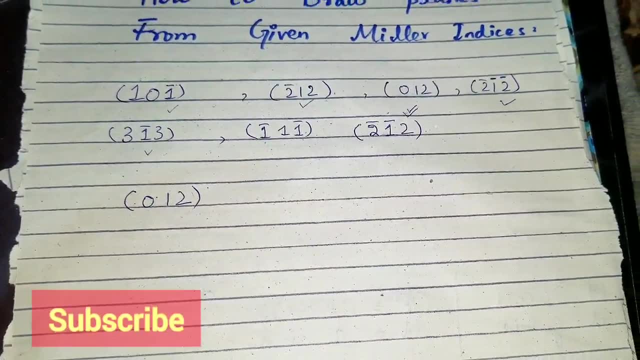 playlist section. It will be more helpful to you to go there. So do check the playlist out and myadticorg to go there and get your uh in desired video. i have also uploaded a video where we have drawn the directions from the given million indices. that includes all kind of cases and 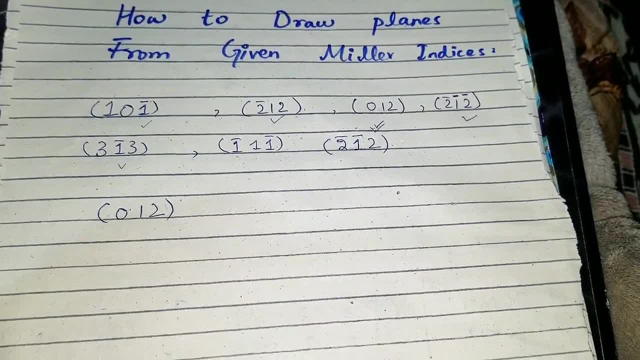 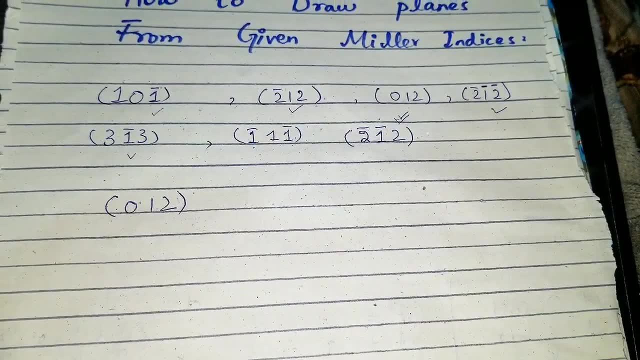 the method that i illustrated here is very simple and can be used for any kind of study. that is given to you and it will help you to have a better understanding of solving the problem. that will help you to solve the problem. so here, the first one is 0, 1, 2. okay, the million indices are given. 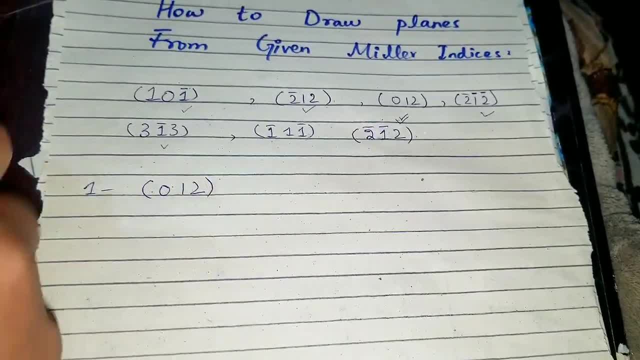 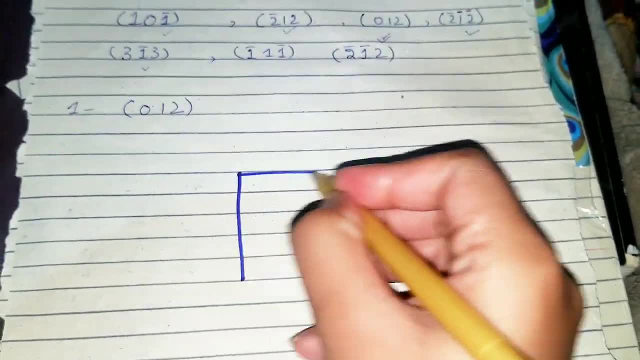 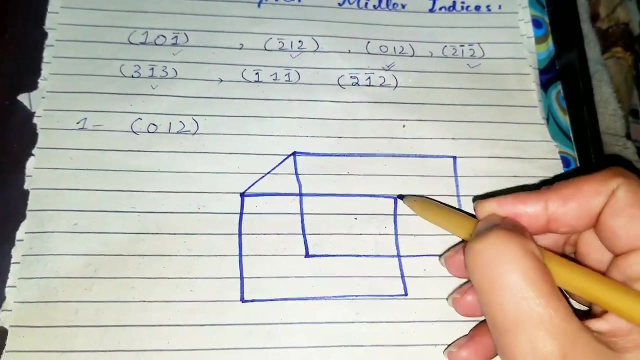 0, 1 and 2, and first of all, what you have to do is to draw a cube. if you have um pens of different colors, then it will be. it will be better because you know uh in 3d diagrams and in drawing the planes in directions, if the different colors are used to uh do different kinds of components. 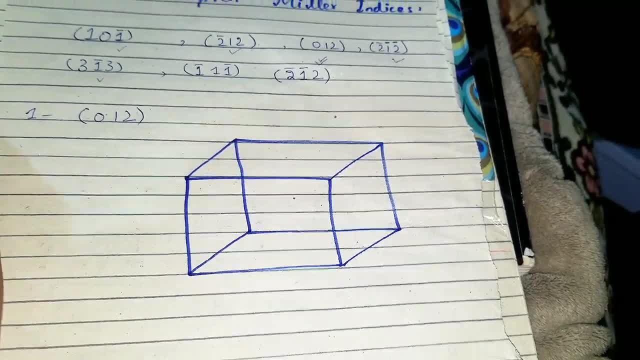 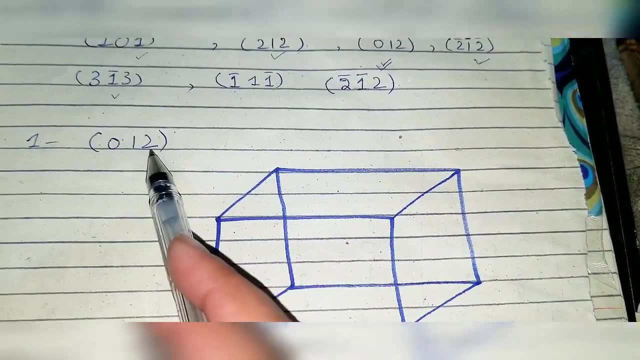 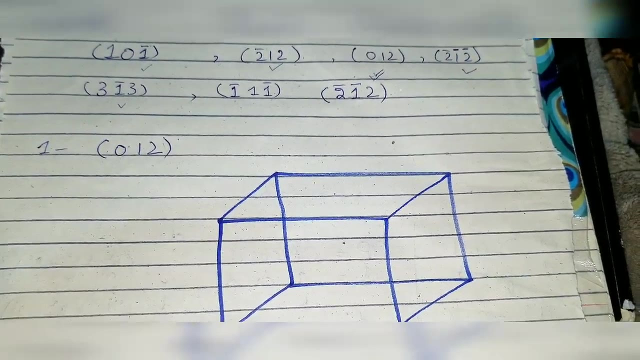 inside a diagram. then you can easily distinguish different components. otherwise you will mix all of the lines. so whenever all of the uh indices are positive, that case will be referred to as all positive case. okay, whenever i'll say all positive case, then it means a case when all of the miller indices 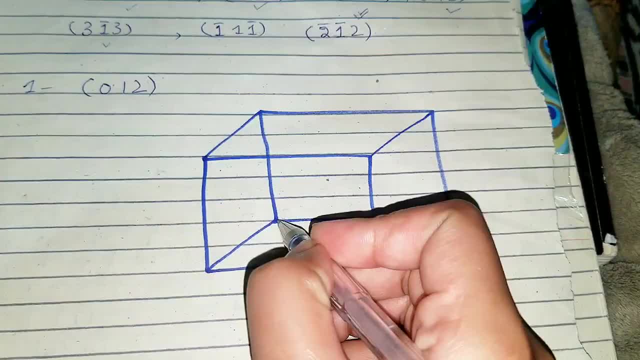 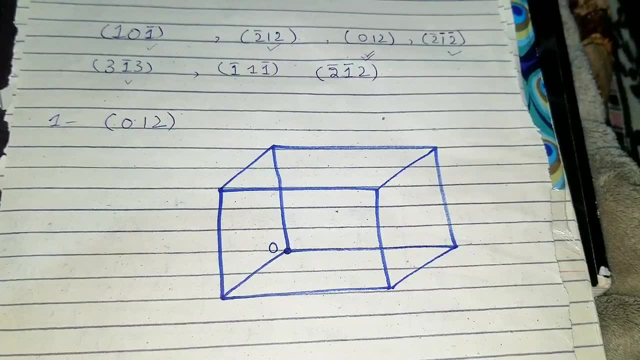 are positive. so when all of the miller indices are positive, then you will always take that one point as origin. okay, so if the one of the index is negative, or two of the index is negative, or three of the index is negative, you will have to shift the origin. the position of the origin is: 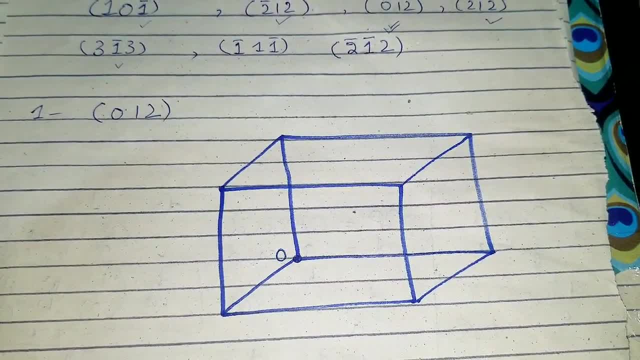 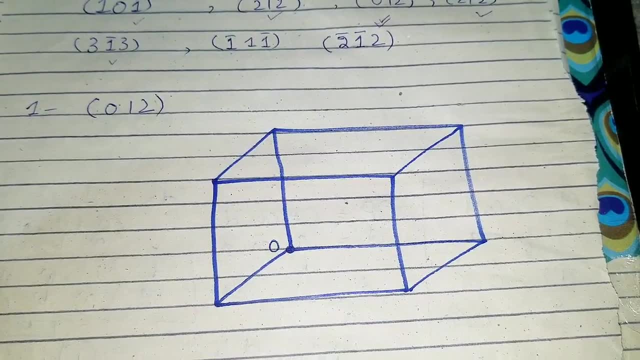 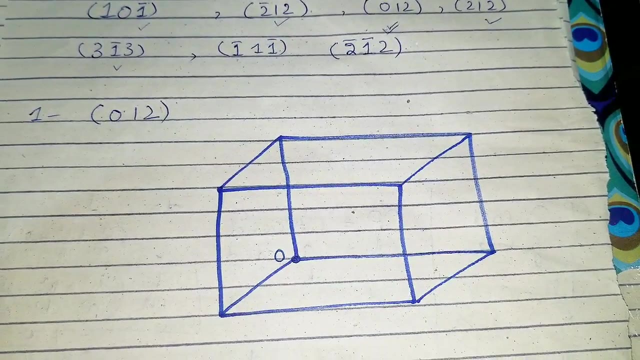 always selected such that the plane that we want to draw uh will lie in a single unit cell, okay. and if you do not uh shift our region, then the process of drawing a plane will become complicated as multiple unit cells will be required to draw the plane, okay. so we don't want to complicate the process and 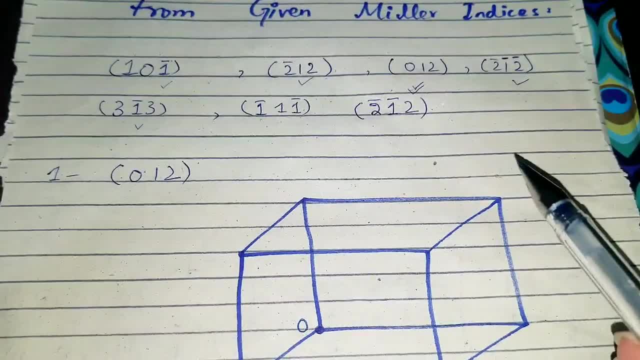 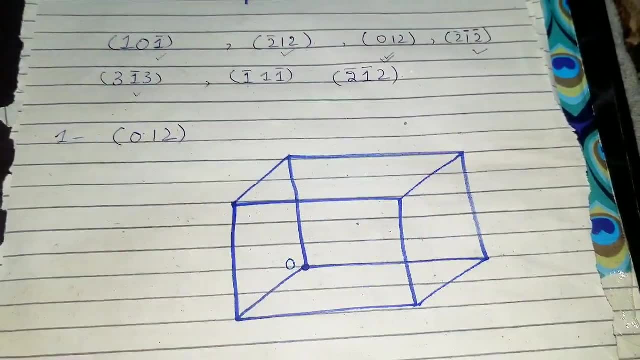 we want to draw the plane in a single unit cell and for that purpose, uh, you have to shift the region whenever the indices becomes negative. and i'll show the process, uh, step by step. okay, so let's do it for the all positive case, and for all positive case, this is the all positive. 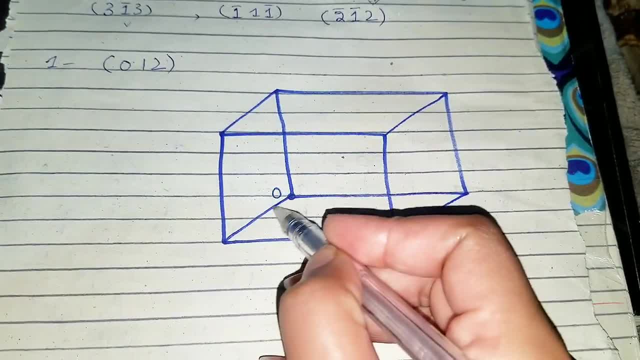 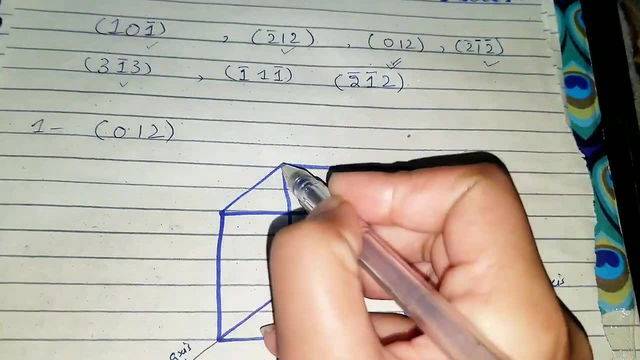 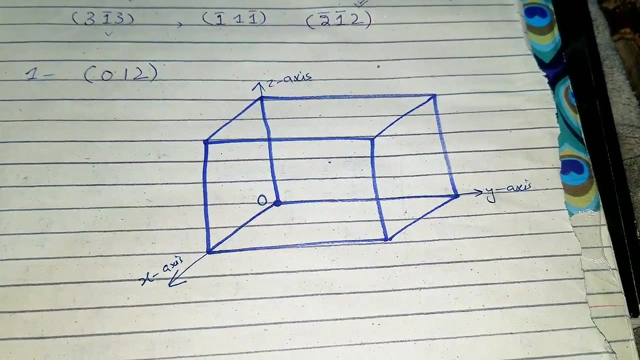 origin. i'll call it as all positive origin. so this is the region, and let us call this line as x-axis, okay, and this line as y-axis and this line as the z-axis. in drawing the planes and in finding out the miller indices for the planes also, uh, the axis lines are very important, okay, because 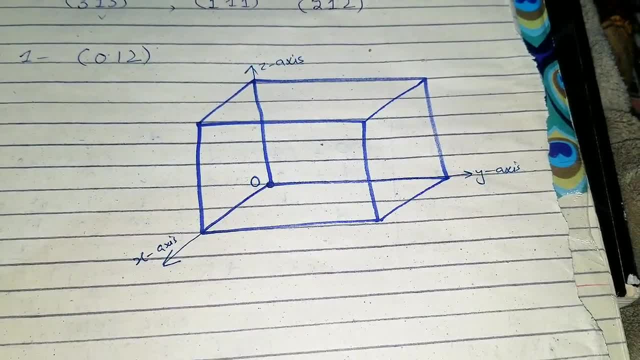 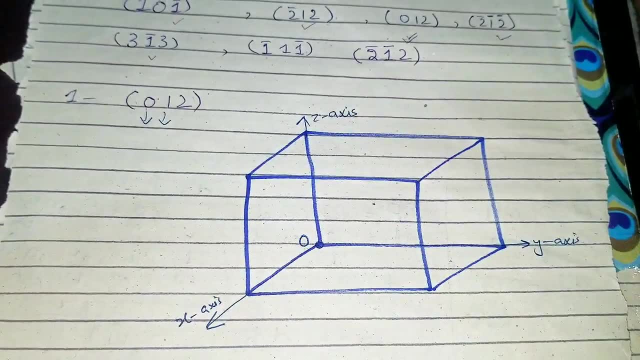 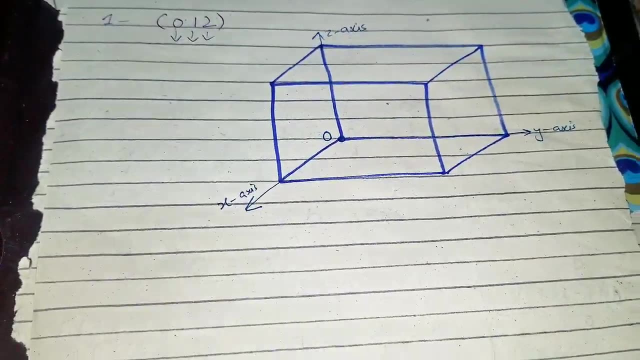 we are interested in intercepts, and intercepts are the point where the plane cuts the axis line. okay, so this will give us the x-intercept, this will correspondingly help us to find out the y-intercept, and this one will give us the z-intercept. so what we have to do is to find out the intercept and to 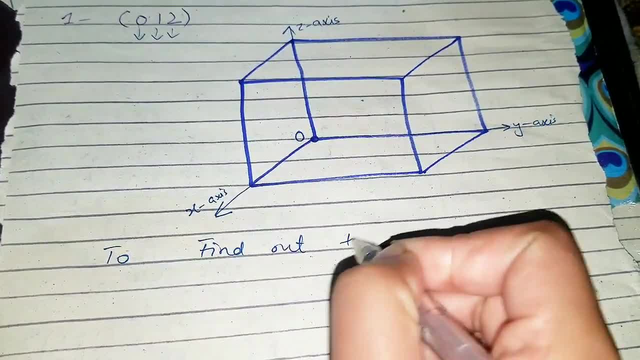 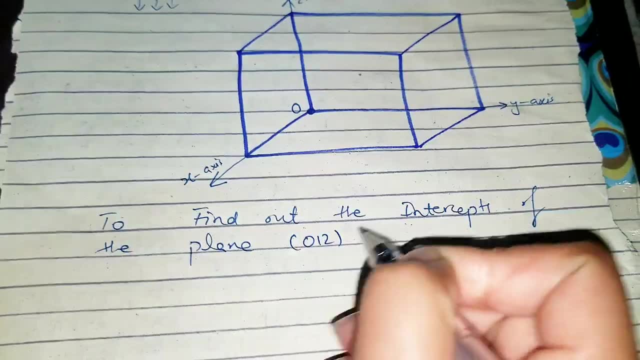 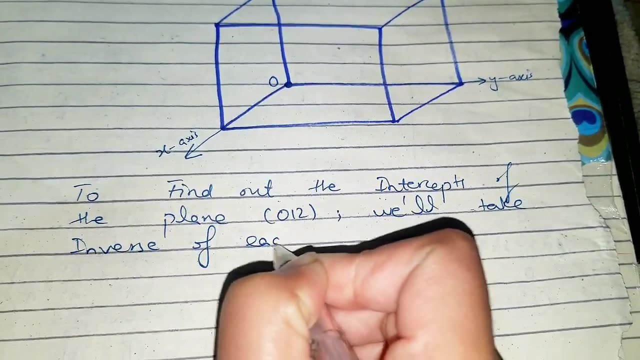 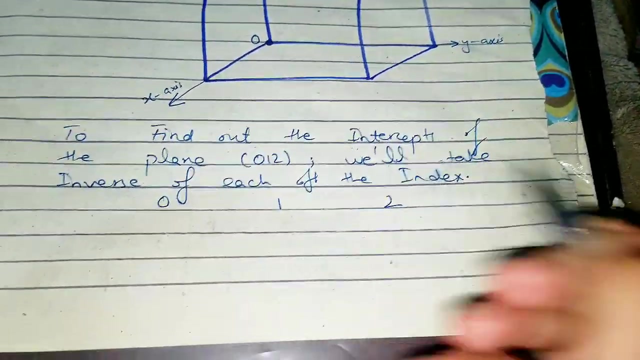 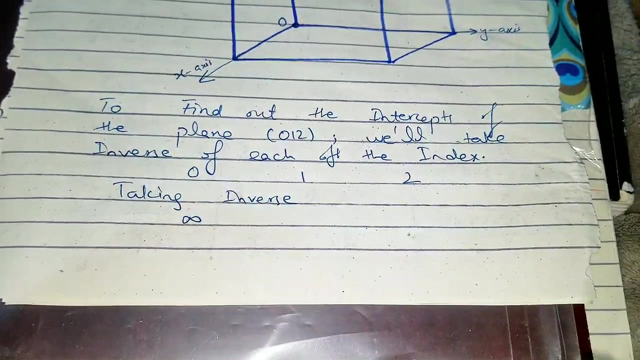 find out the intercept, to find out the intercepts of the plane, zero, one, two, we, we will take inverse of each of the index. okay, we'll take the inverse of each of the index. uh, the indices are 0, 1 and 2. okay, taking inverse will give us an uh intercept. so taking inverse of 0 will give us infinity. 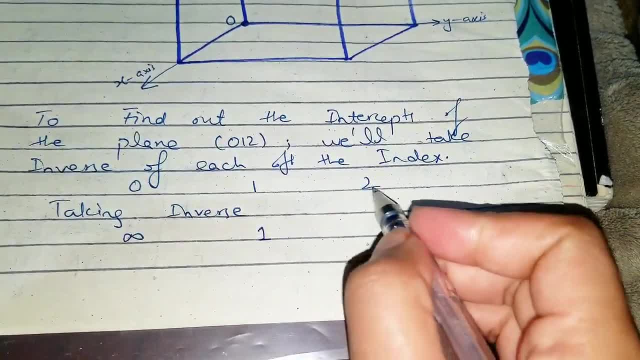 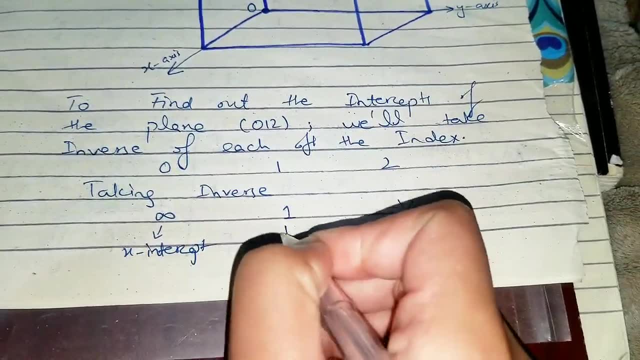 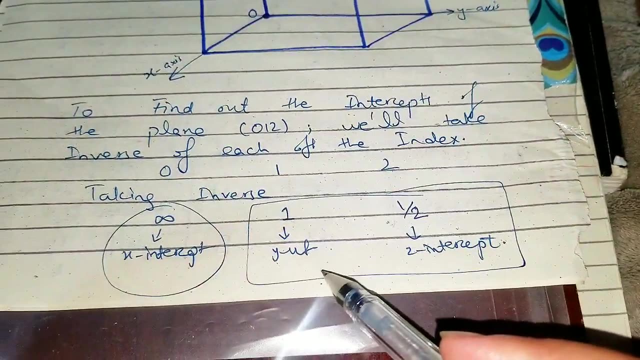 taking inverse of 1 will give us 1 again, and taking inverse of 2 will give us 1 by 2. all right, so this is the x-intercept, and this is y-intercept and this is the z-intercept. okay, so first of all, we'll focus on the intercepts which are not infinity. okay, the infinity cases are: 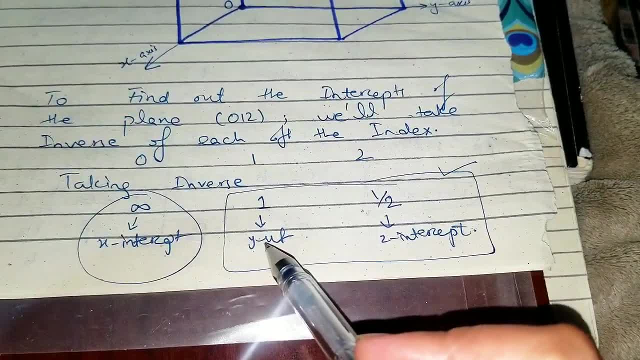 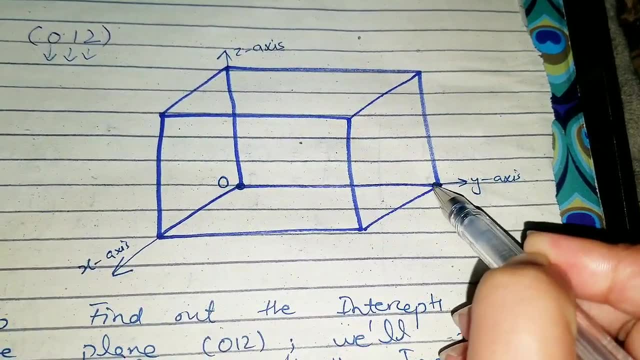 uh considered at the end: okay, at last. so, first of all, the y-intercept is one which means, uh, from origin to the other corner of the unit cell along the y direction, which is this one point. so this is the y-intercept, and let us uh make it prominent. okay, with some other ballpoint are making a very 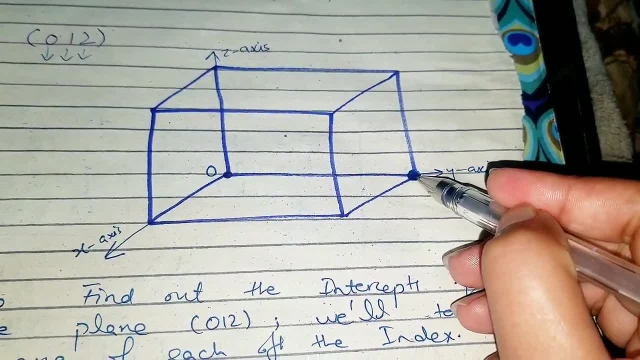 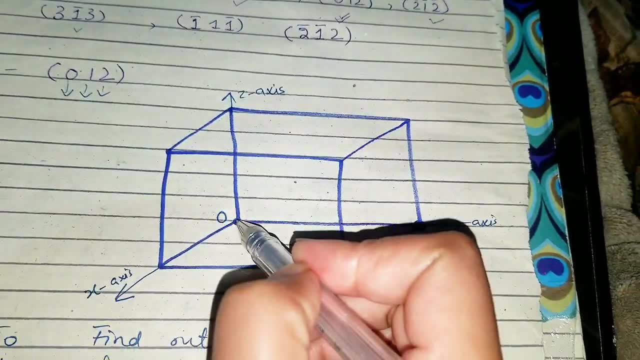 big dot so that it shows that it is one of the point on the plane. okay, this is the y-intercept. i have drawn that point now for the z-intercept and this is the z-intercept and this is the y-intercept. the other intercept is z-intercept, which is half so from origin again. okay, um, in drawing. 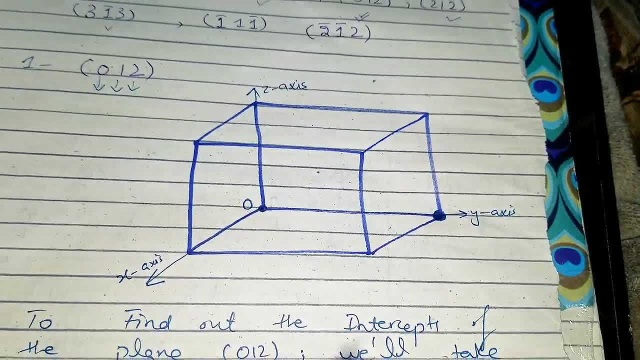 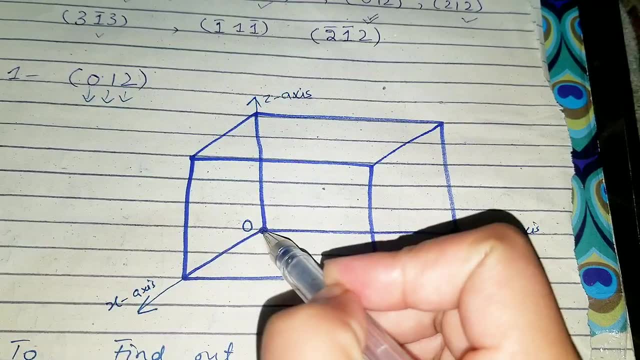 the intercepts, you always move, starting from origin, while in case of directions you move onwards from the point you left. okay, so, uh, from origin again. uh, half unit along the z-axis. this whole length from one corner to the other corner of the unit cell is one and half of it is about. 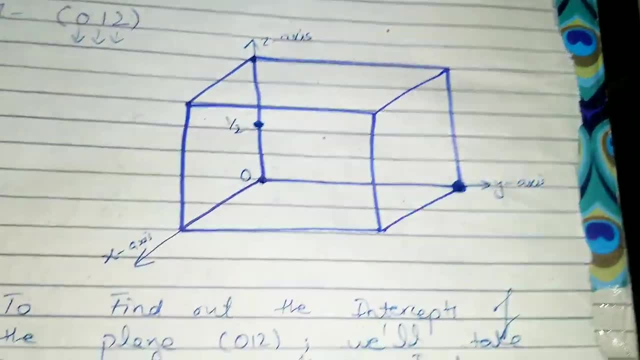 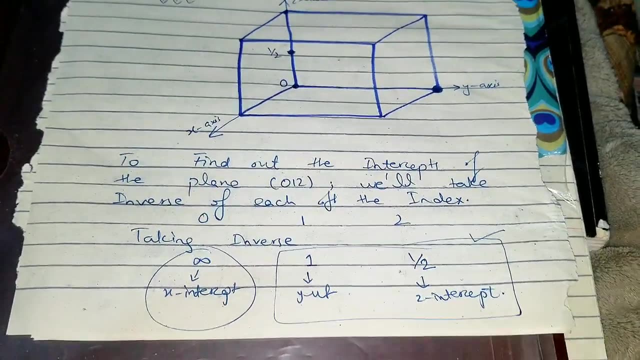 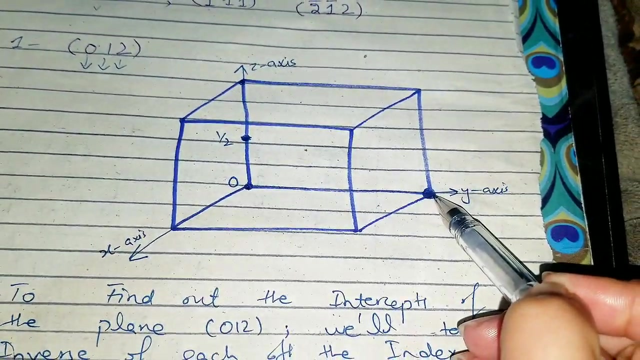 here. so this is the other point on the plane. all right now. uh, next thing is: x-intercept is infinity. so x-intercept is infinity. how will to deal with that is, we will, uh, draw a parallel line from each of these two points that we have found for the plane. okay, parallel lines from this. 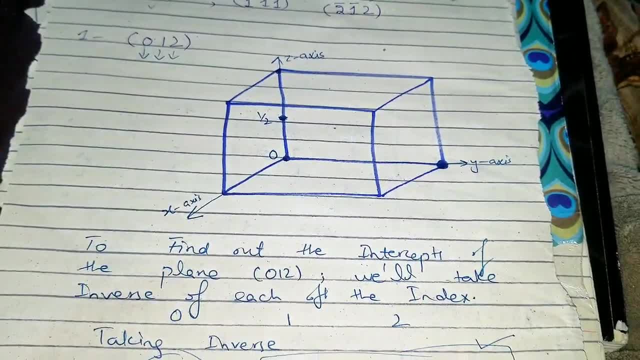 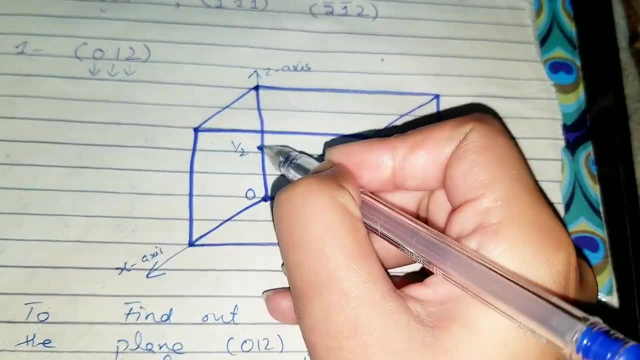 um, these points along the x direction? okay, parallel to x direction will draw parallel lines. uh, from this point. so let us draw the parallel lines. the direction is here, okay, so from this point, parallel to x-axis. is this point to the other corner of the unit cell? okay, you will stop. 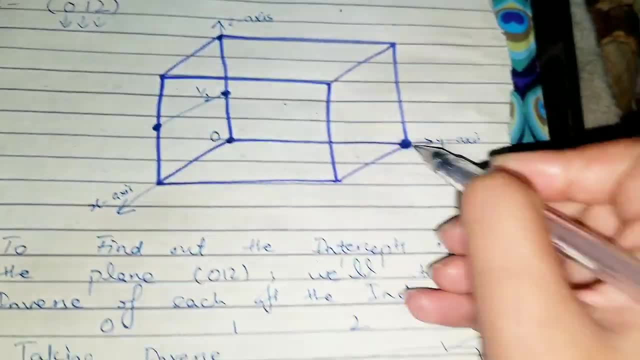 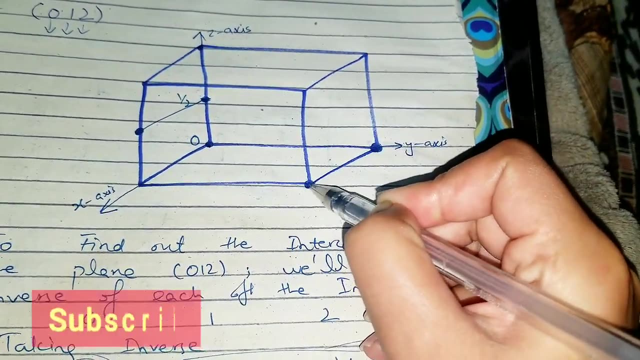 to the other corner of the unit cell, which is now this point. okay, and again, also from this point, we'll draw parallel line along the x direction, which is this direction, and up to there. okay, next one, we have to join these four points together to form a closed figure. 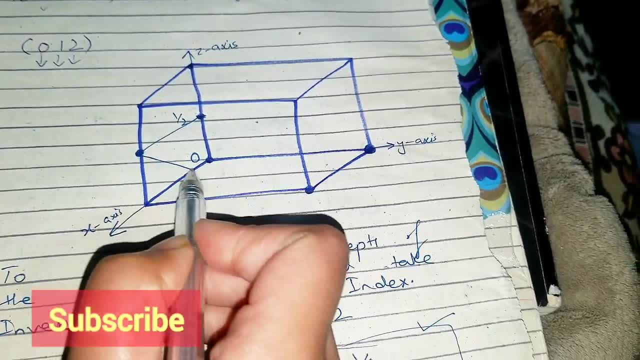 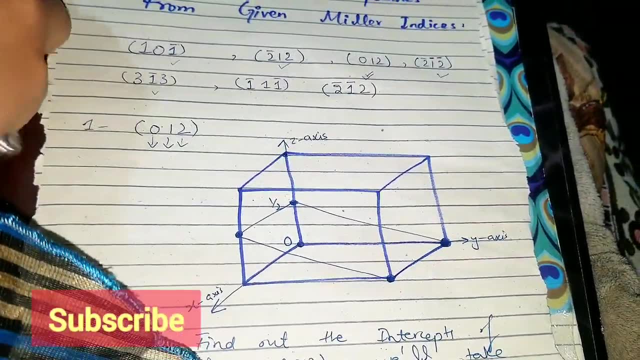 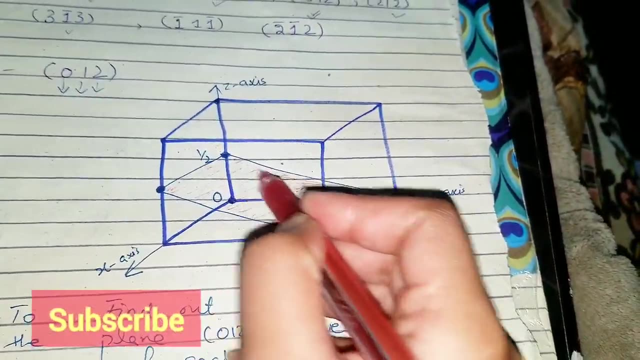 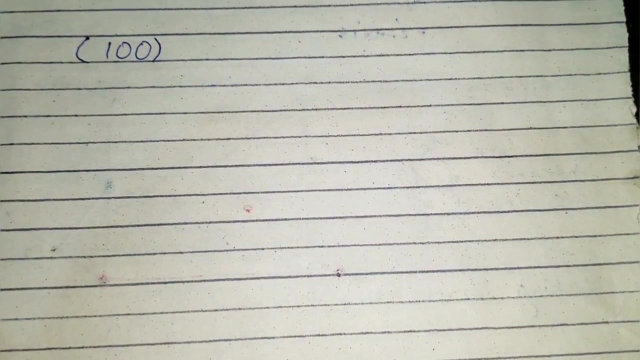 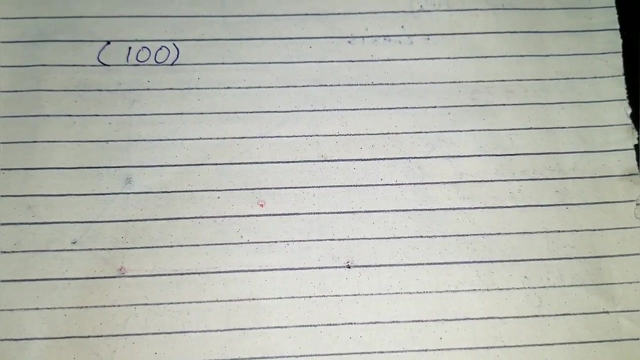 so we'll join these two points together in these two points together and okay, and this is the plane zero one, two. shared it like that, okay, so this is the plane zero one, two. all right, so this is example that i am going to show you people because, uh, sometimes students get confused when, uh, this one plane comes in, because if we take the 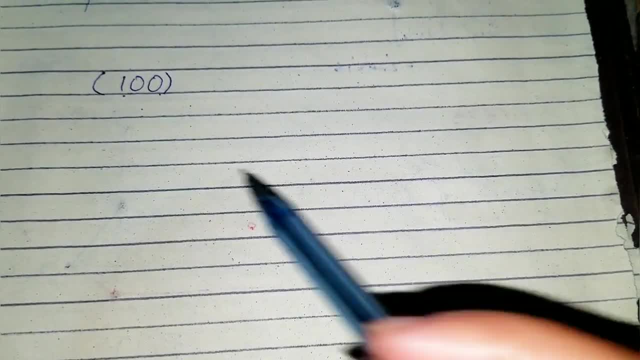 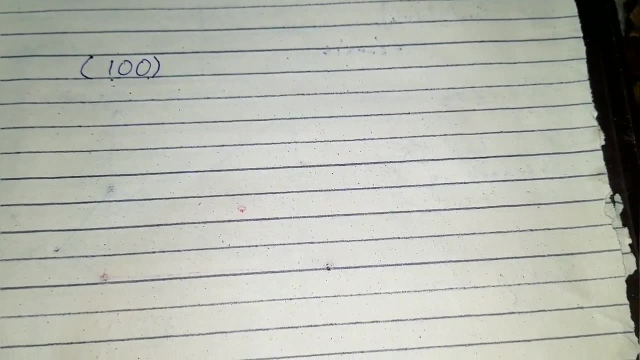 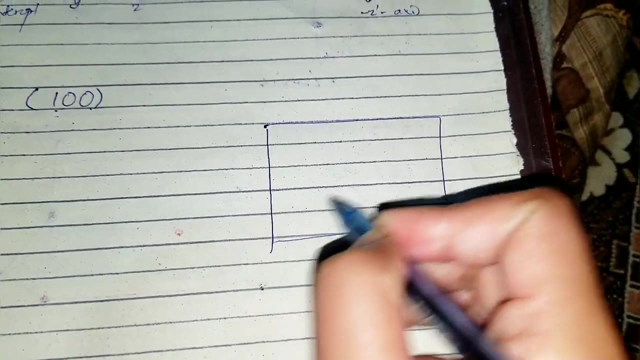 inverse of these three million. this is in order to get the intercepts for the plane. then, um, you get two infinities and one as one of the intercepts. so how you will draw this plane, okay, so, uh, we have a cube first. okay, we will first draw the cube. 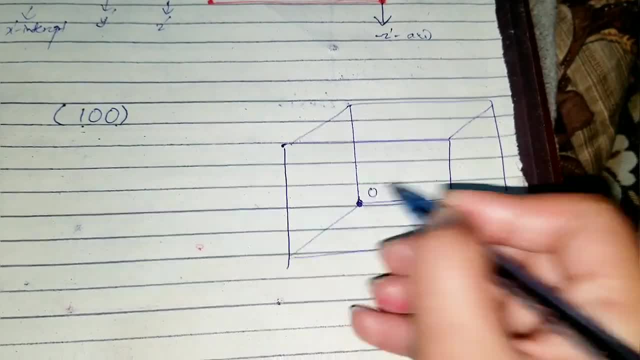 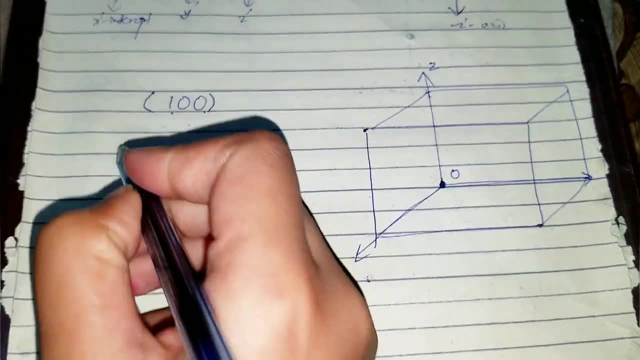 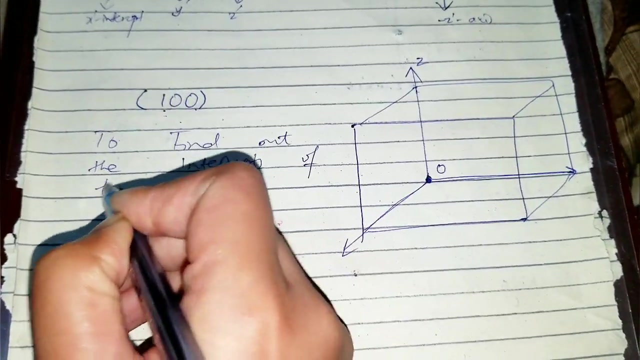 since all of the miller indices are positive. so we'll take this point as origin. okay, this is the x direction, this is the y direction and this is the z direction. all right, so to find out the intercepts of the plane, one, zero, zero, we'll take the inverse of each of the index. 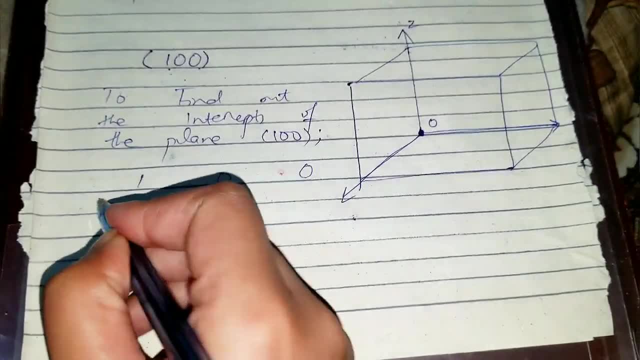 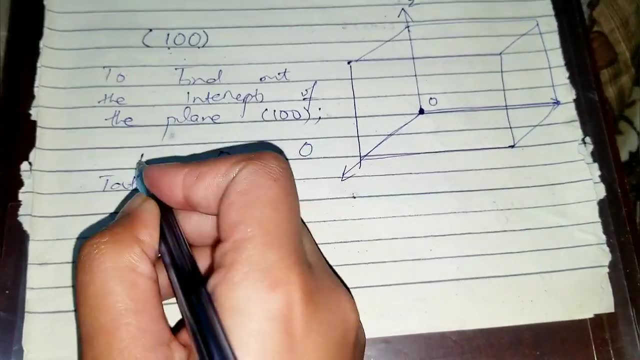 you'll write it yourself and these are the three uh indices. we'll write the operation that we are going to perform on these indices, that is, taking inverse, uh, taking inverse and inverse of one is one. inverse of zero is infinity. inverse of zero is infinity again. so this is the x. 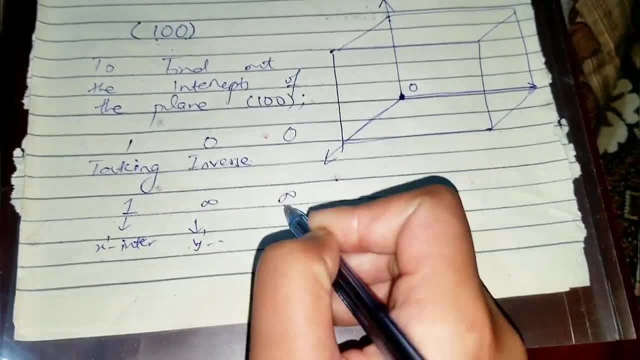 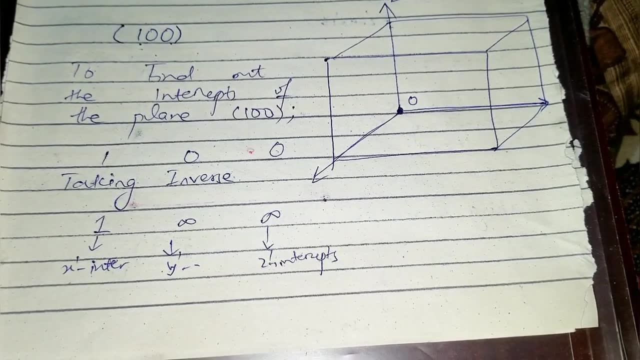 prime intercept, this is the y prime intercept and this is the z prime intercept. it's because when you are finding the miller indices of a plane, you take the inverse of the original intercepts um that are found for the plane. so in order to find out the intersection on the miller, 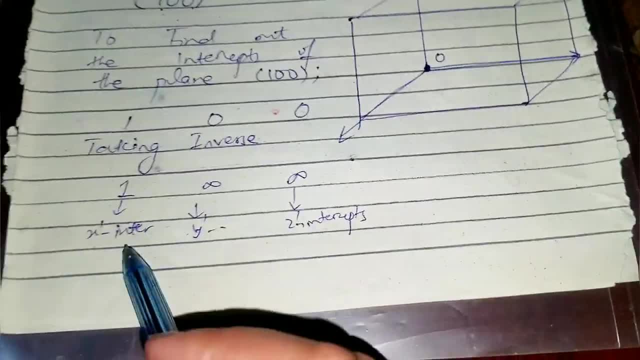 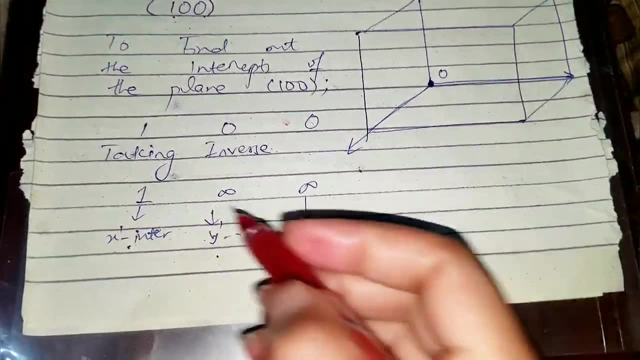 indices, you'll reverse the process, which is to take the inverse again. okay, so this is the x prime intercept. y prime is infinity and z prime is infinity again. and, uh, we deal with infinities at the end. first of all, we'll draw the um intercept, which is not infinity. okay, so that is x. 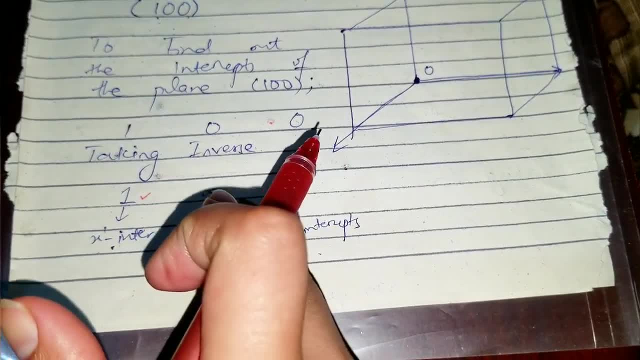 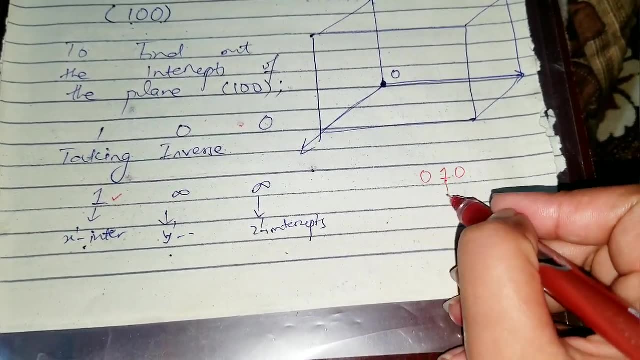 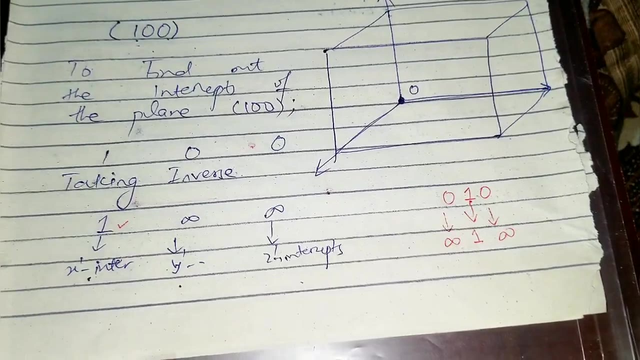 prime intercept. and if it would have been uh y prime intercept, like for that one case, then you will draw the y prime intercept first because, corresponding to that, you will get a non-infinity result, while for the other two you will get the infinity. so infinities are dealt at the end and we'll deal with the ones which are. 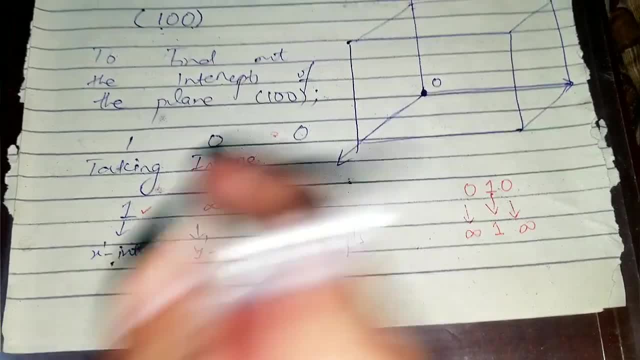 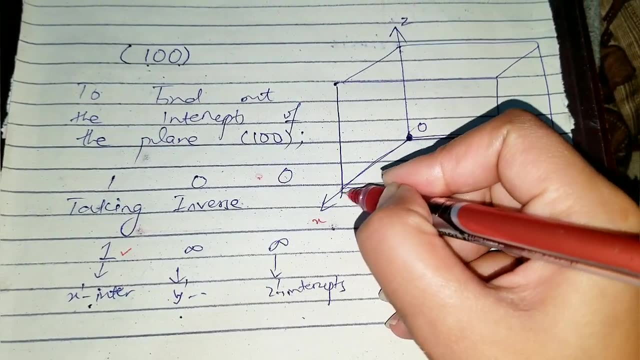 not infinity first. okay, so that's x prime intercept, which is one. so x prime intercept means from origin, one unit along the x direction, which means to the other corner of the unit cell, which is this point. okay, this is one of the point on the plane. now we have got this point and by using 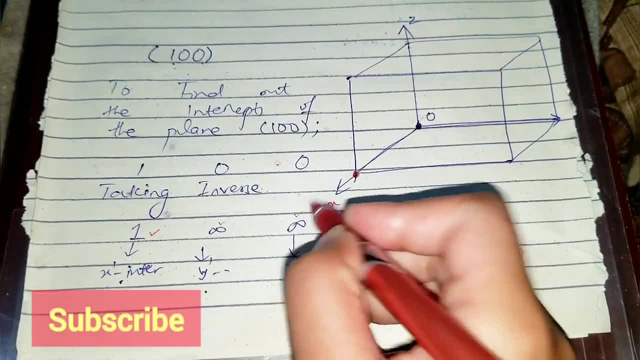 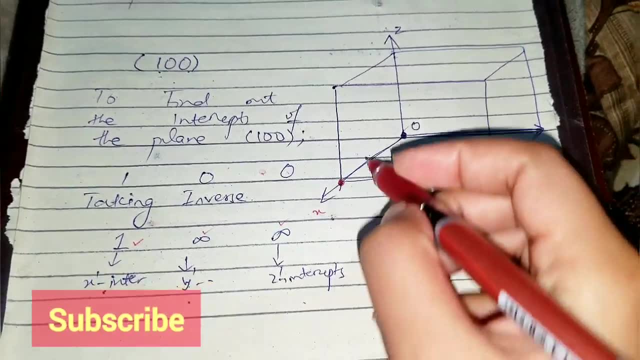 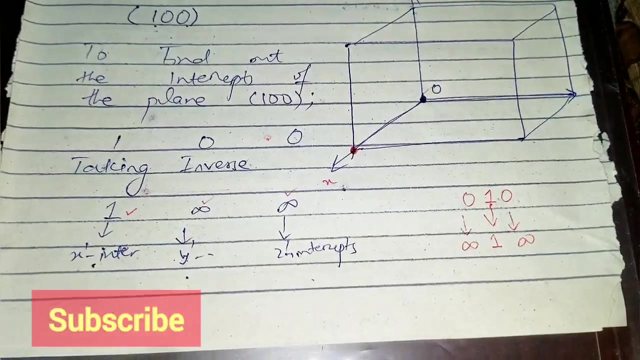 this point, we can draw the whole plane along with this information. now the y prime intercept is infinity, so what you have to do is to draw the parallel lines. um, from this point, okay, from this point, along the y direction, y positive y direction, okay. so from this point we'll draw. 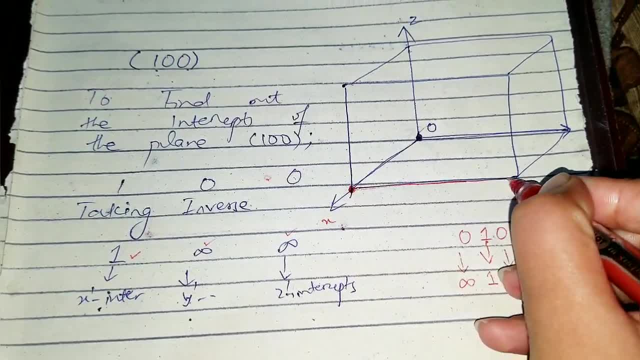 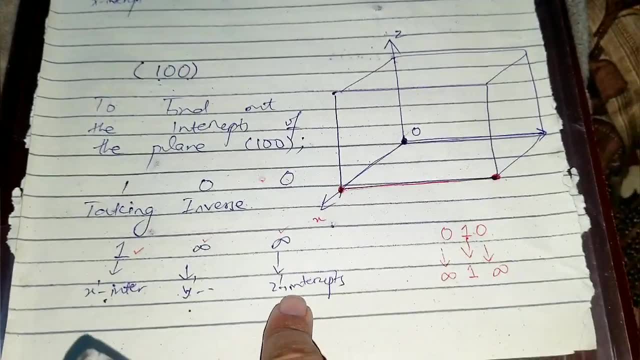 the parallel line along the y direction, which is this direction with the other corner of the unit cell up to the other corner of the unit cell. okay, now, this is another point on the plane. after that, since the z intercept is infinity, from these two points you will draw parallel lines along. 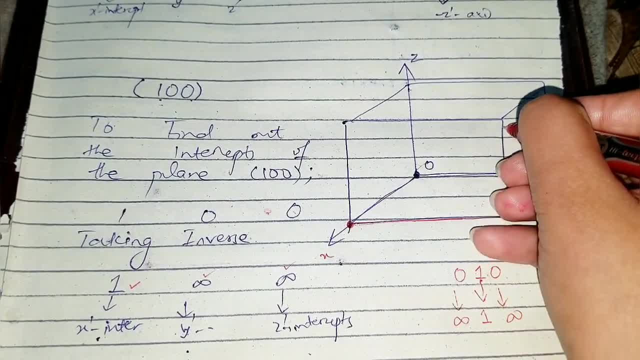 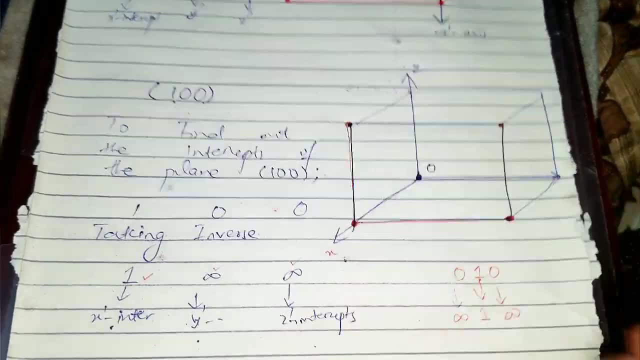 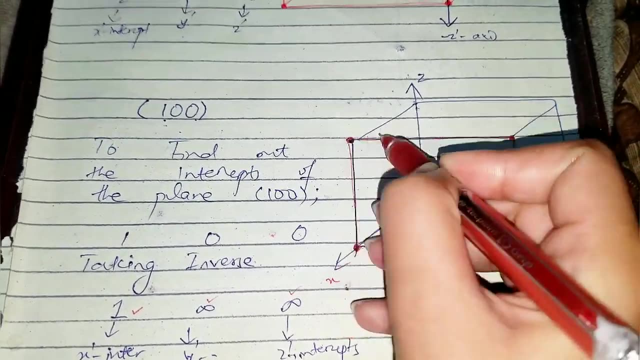 the positive z direction, which is like that, okay, ending without the corner of the unit cell, and also like that: okay, and we'll join these two lines, these two points together, in order to form a closed figure of a plane. and here we go, this is the plane one, zero, zero, all right, and this is the. 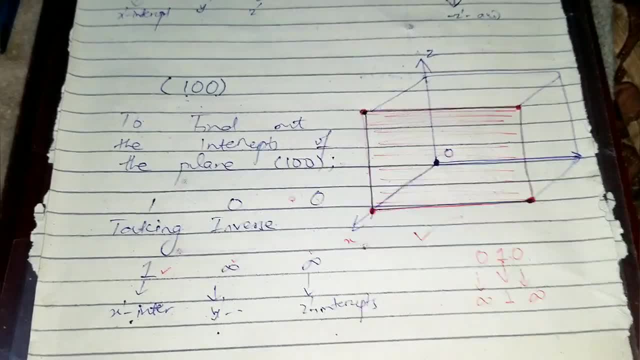 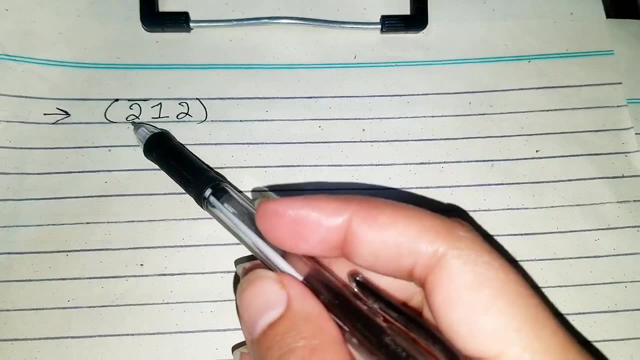 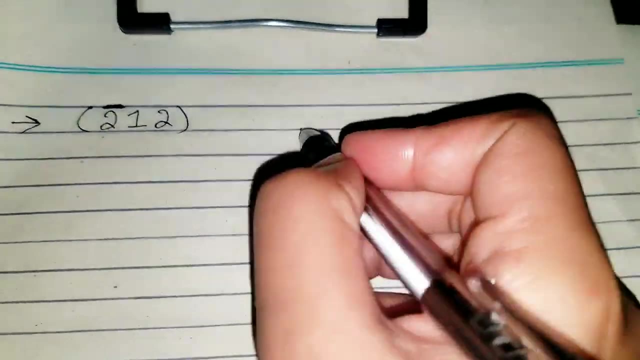 front wall of the cube. all right, and i hope you got the method. now we'll get to know the method for the negative miller indices problem. here the x index is negative. two bar one, two. okay, it's bar over two because it's black pencil, maybe it's not quite visible, but it's two bar one, two. these are the. 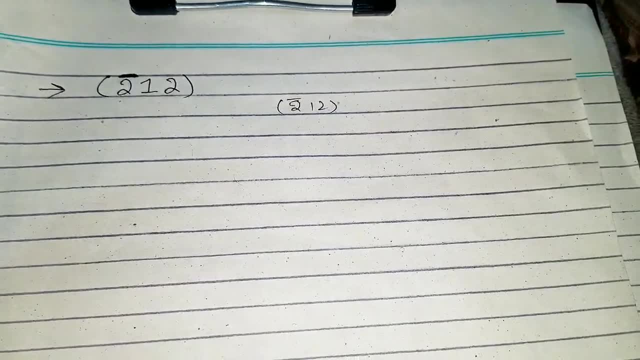 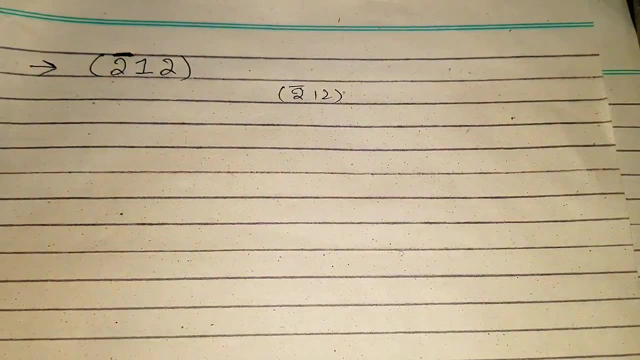 miller indices of the plane that we are going to draw and the x index is negative. so the origin shifting is required here. the rule is very simple and it will be applicable to all kind of planes you are drawing. okay, even if it is the indices of a direction. and if it is, if they are negative, then the rule for origin shifting, uh that. 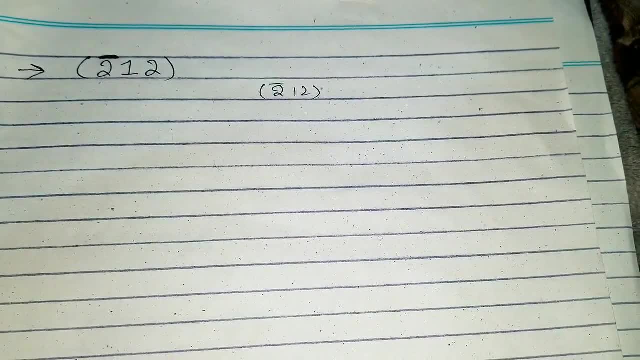 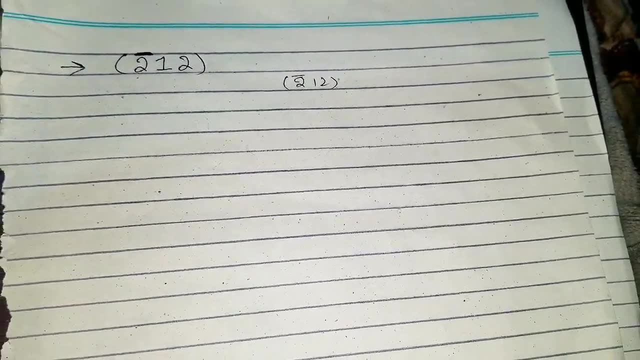 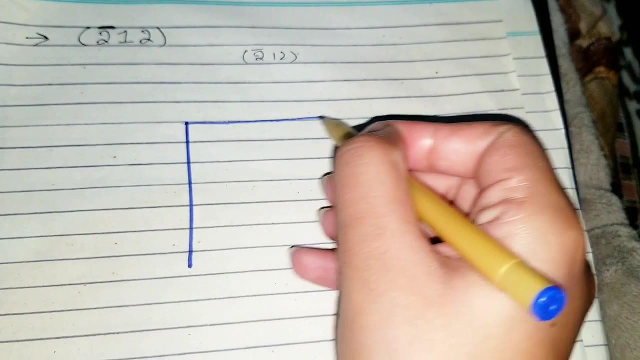 we use here- uh is used there too for origin shifting while drawing the directions. okay, i will display the rule step by step and you'll understand it by watching the problems. you know you cannot at first understand it completely, so let me first draw the cube while drawing the planes. 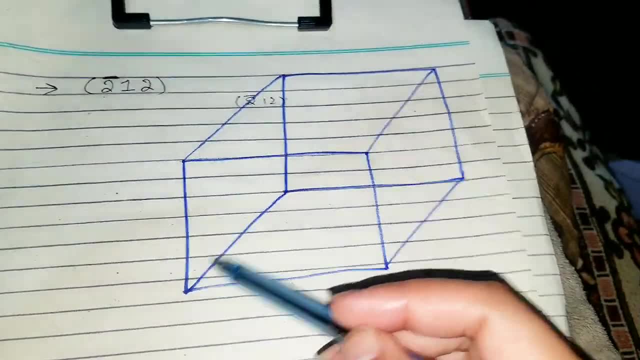 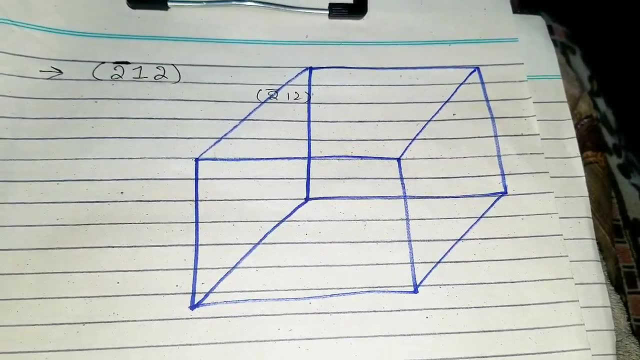 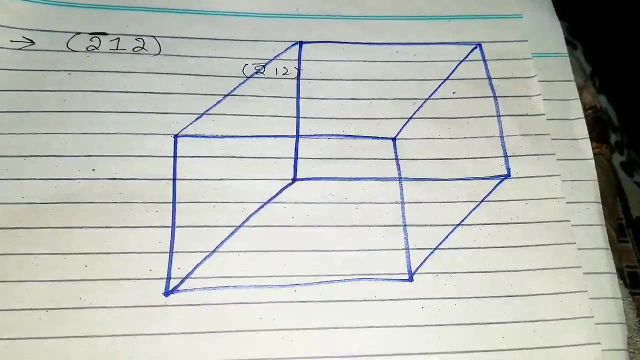 if you need to draw a line, then draw a line. yes, that is when it is happening first. and then you have to find a갖code measure to break the triangle down, okay, and then when you is to end up with an array of really nice двухazing size that is longer than one plane if you end up, 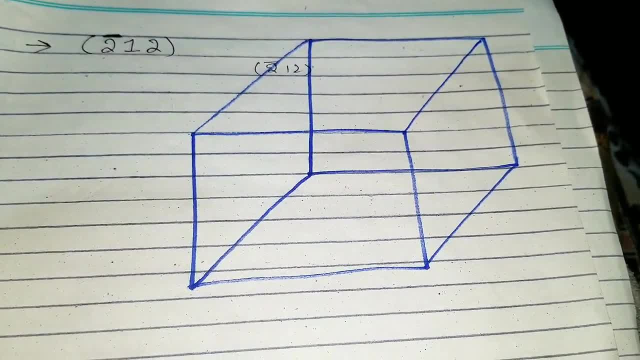 with a small one, then the !113 scale is going to be getting twice greater than the won of the million decim 2006. that's a simple thing to do, but also that's quite not important. that's cuz you need to keep a range like that. you put a short number below the size. 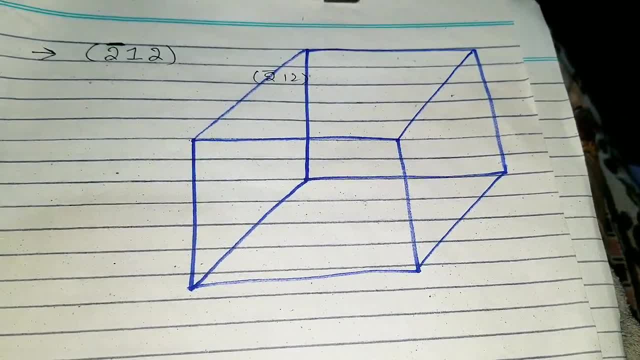 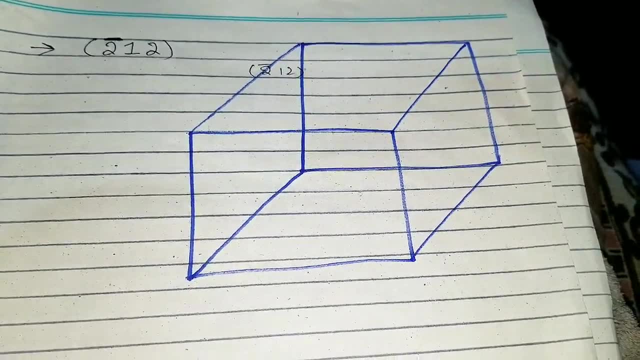 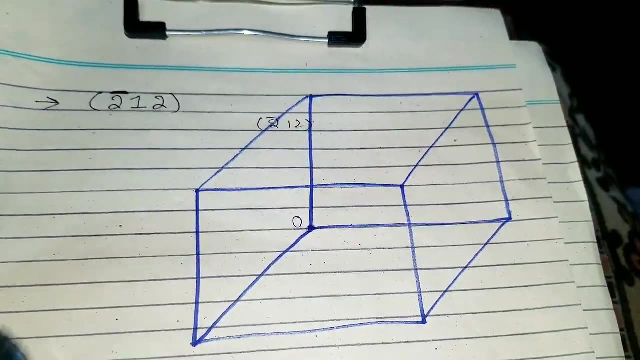 of the cube. the lengths are equal to each other or not. the issue doesn't arise there, but the issue will arise in case of the drawing of plane. okay, so yeah now. first of all, this was the all positive origin. let me call it as o. okay, and since the x index is negative, what you have to do is to shift. 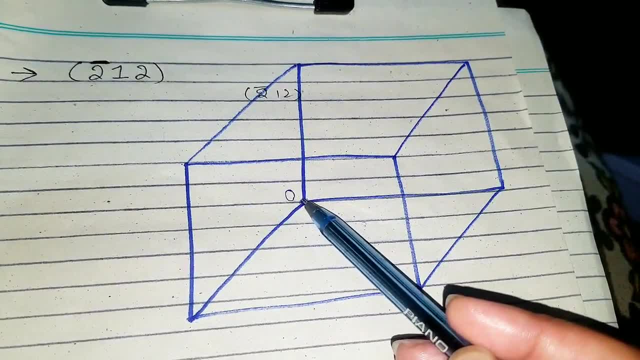 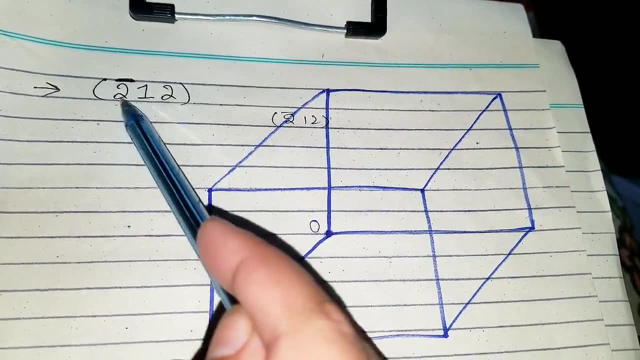 the origin by one unit along the x direction because the x index was negative. okay, whenever the x index is negative, regardless of this numerical value, okay, this numerical value doesn't hold anything, uh, in deciding the position of the origin. okay, if it has been seven bar one. 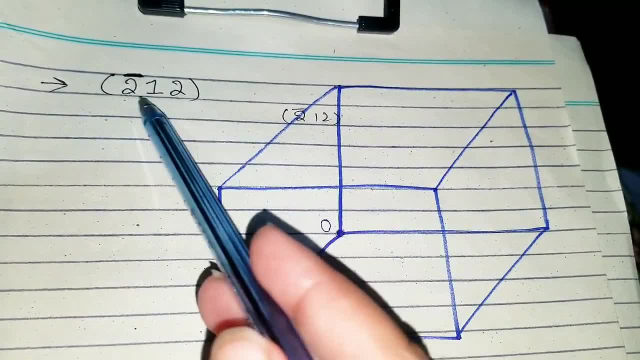 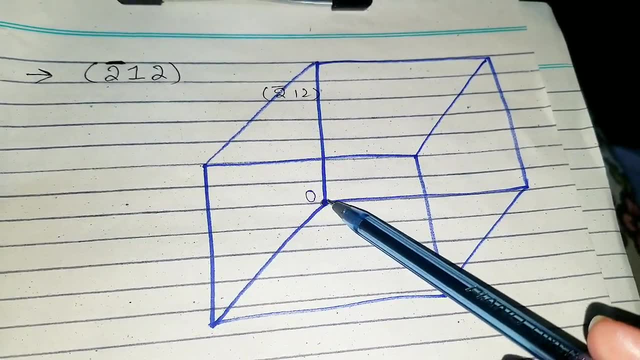 bar, or three bar, or two bar or whatever the value is, that doesn't matter, it's x index and it is negative. that matters only, okay. so whenever the index is negative, you have to shift the origin, starting from the all positive origin, uh to uh, uh, by one unit along that direction, which is: 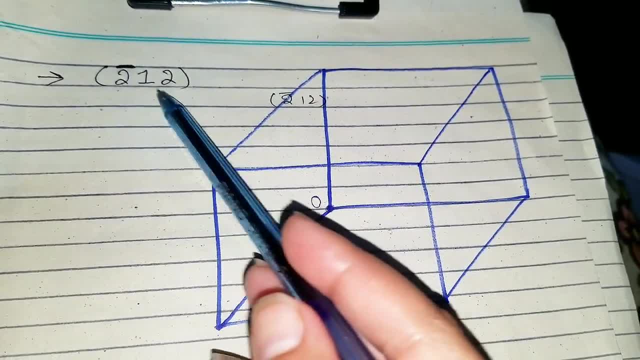 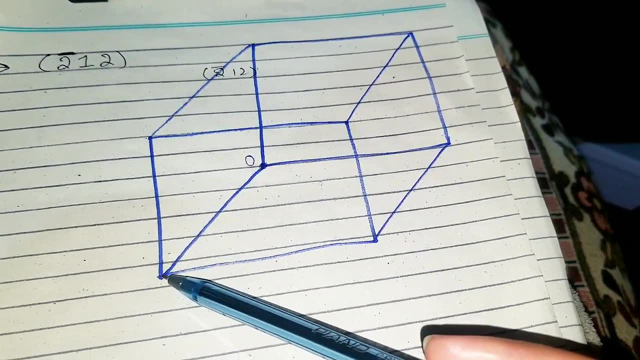 having a negative milli index. okay, if two of the index is indices are negative, what you have to do is starting from the origin. you will shift the origin by one unit along one direction. then from that point onwards, okay, continue. uh, from that point on that. from that point onwards, you have to shift the origin one more time along that. 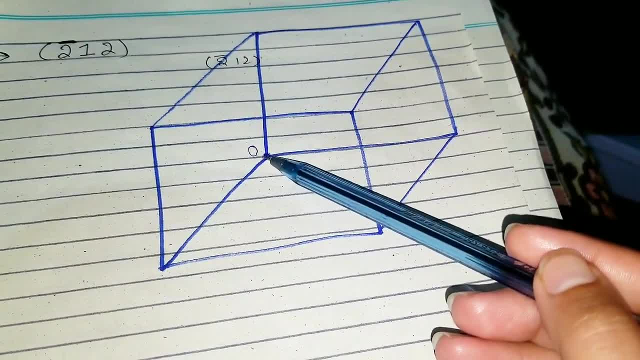 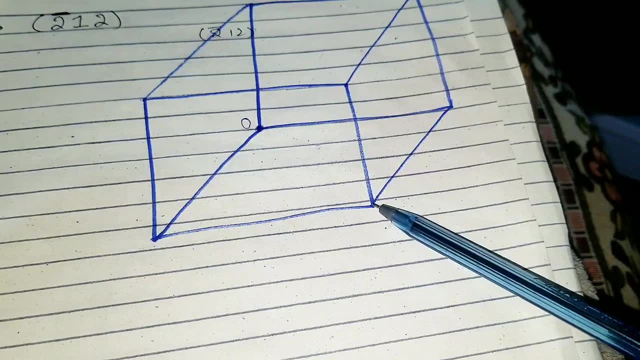 direction. for example, if x and y index would have been negative, then i will shift the origin from that point along the x direction there, then along the y direction, by one unit there, so that one point would have been the final origin. okay, if the y index and the x index, both of them would. 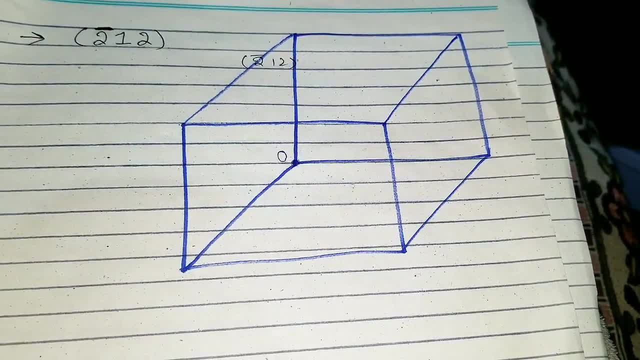 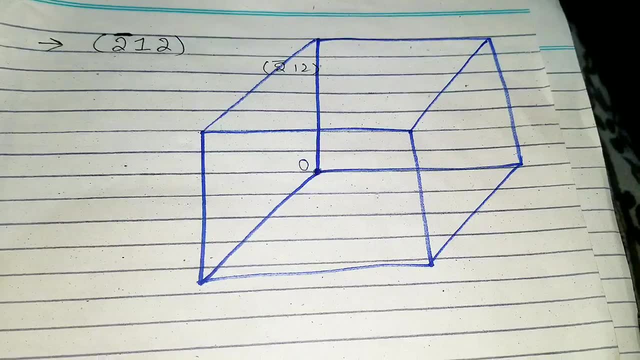 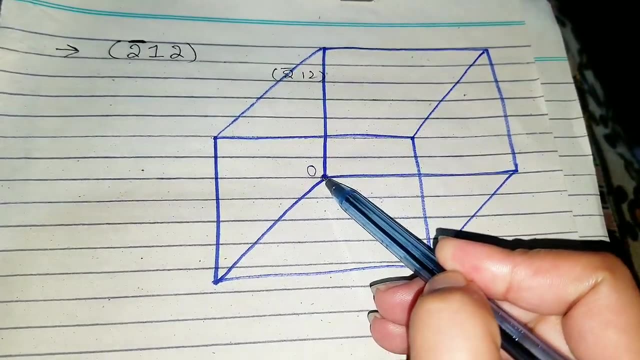 have been negative. so the process continues, uh, depending upon which one of the indices are. uh, which of the indices are negative? okay, so the process will be more clear to you when, uh, we solve the other problems. okay, so, first of all, the x index is negative, so i will shift the origin, starting from all positive. 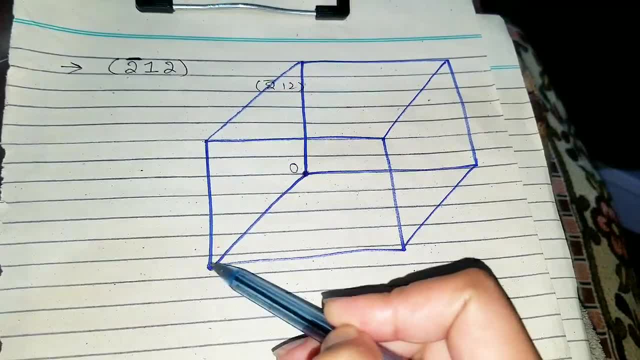 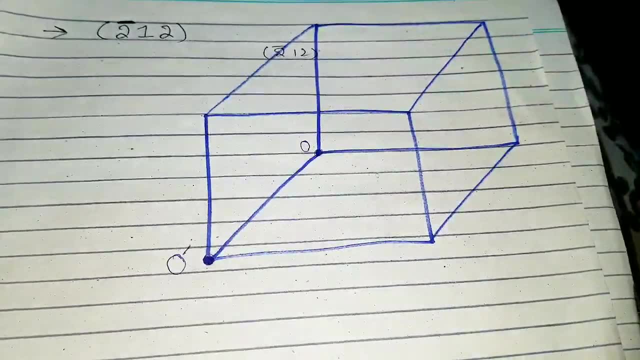 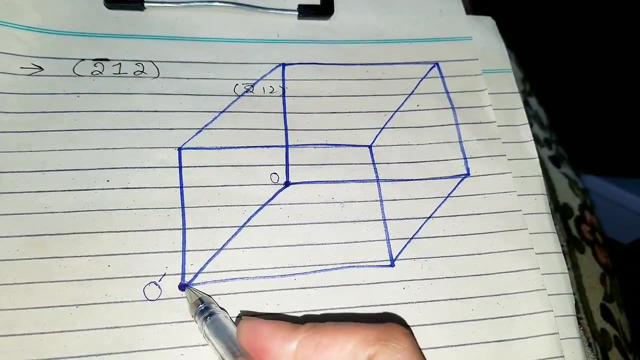 origin uh to uh by one unit along the x direction, which is this point. okay, since the other indices are positive. that is why no more shifting is required and this is the final origin that we will use to draw that uh plane. so let me um designate the axis lines, because axis lines are very important. we have to draw 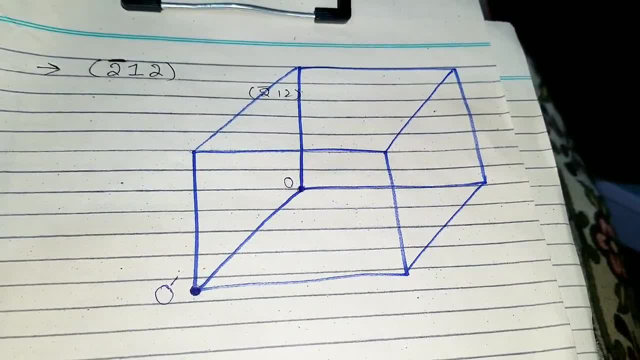 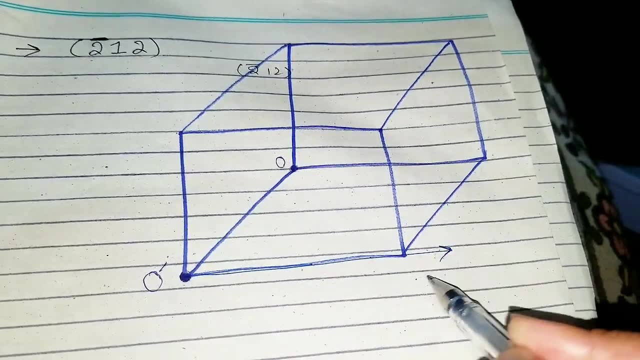 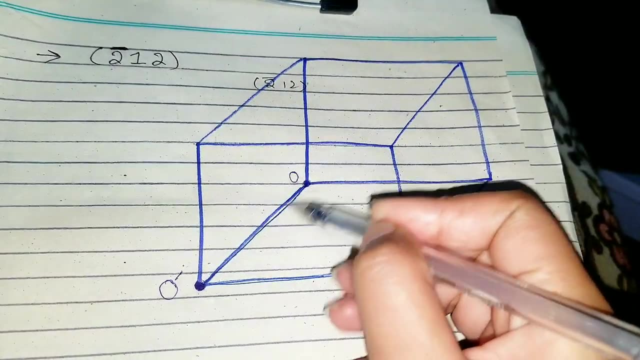 the intercepts. and intercepts are the points on the axis lines, not any other lines, but axis on axis line. so this one line joining, that is connecting the origin, is the positive y axis, y prime axis, since the origin is o prime and we'll use a primed and uh symbol. so this one is the 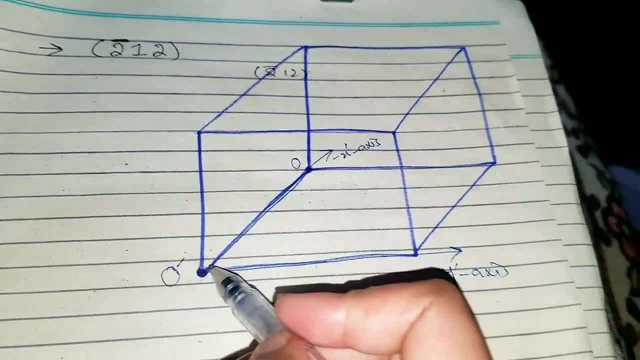 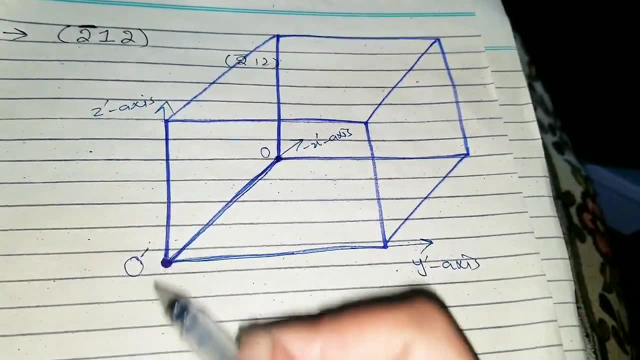 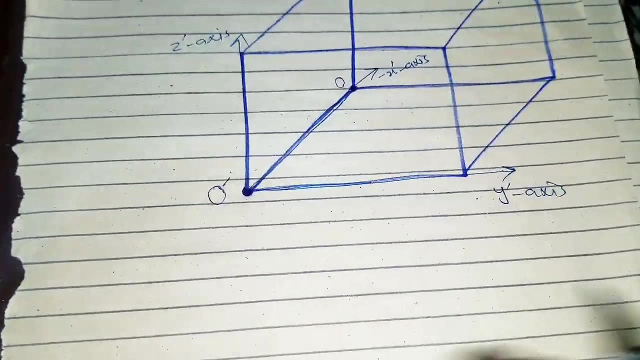 negative x prime axis. since the x index was negative, okay, and this is the positive z prime axis. okay, the lines that are connected to the origin are the axis lines and we have designated their names, all right. after, uh, deciding the position of origin, we need to find out the intercepts of the plane. now to find out the intercepts of the plane, 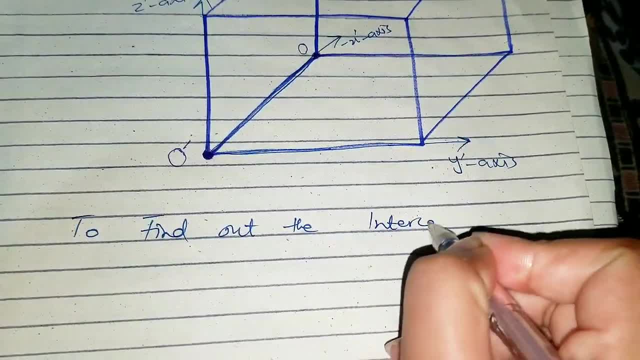 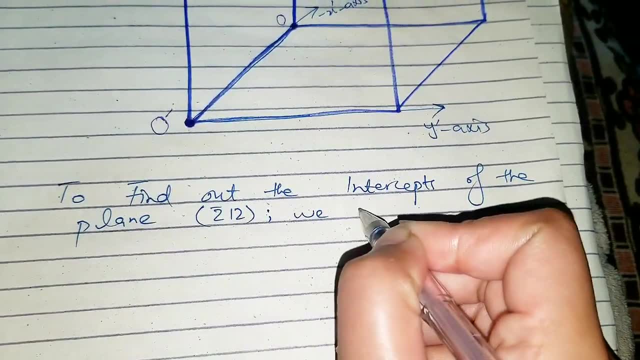 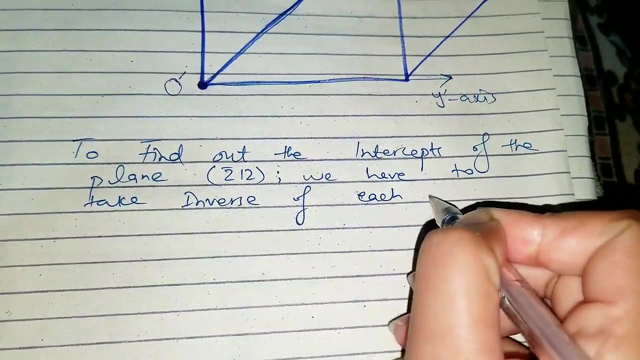 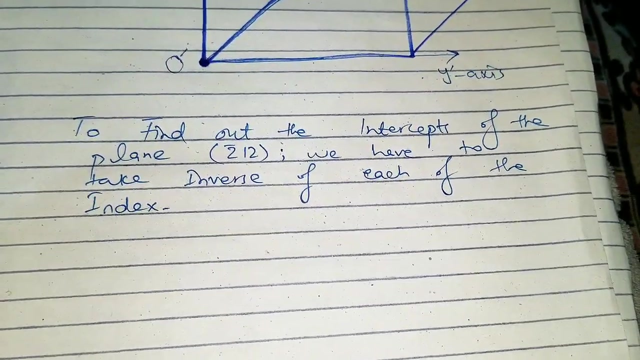 two bar one. two. we have to take inverse of each of the index, because in finding out the miller indices of the planes we take the inverse of original intercepts of the plane. okay, so to find out the plane from miller indices we have to do the reverse process. 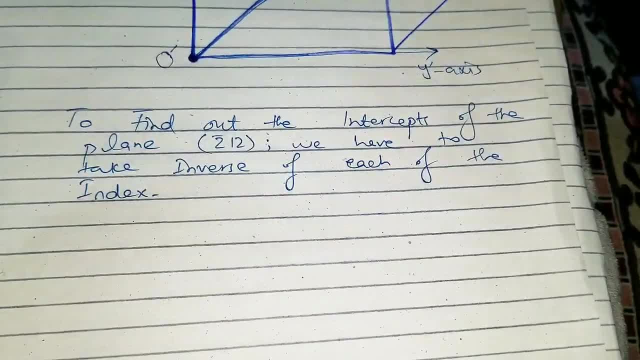 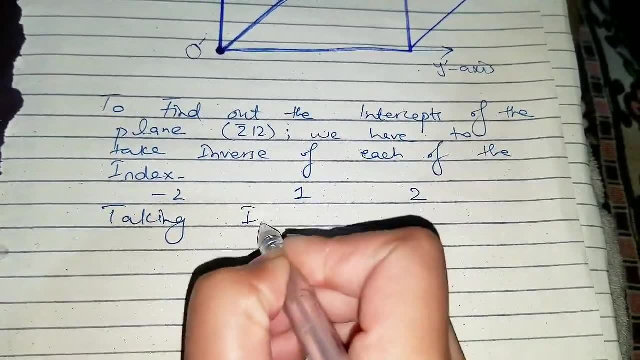 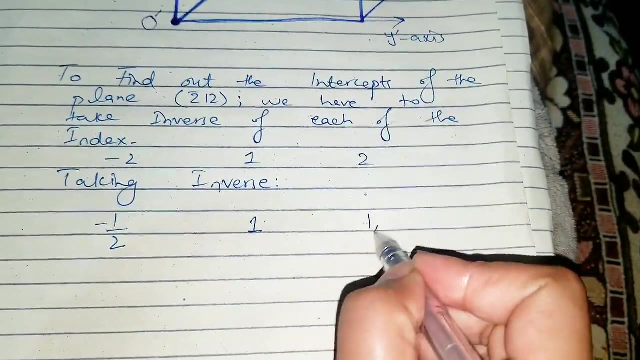 which is to take the inverse of, uh, the miller indices again to get the intercepts. so these are the intercepts: minus two, one and two. the operation to be performed is taking inverse and inverse of minus two is minus one by two. inverse of one is again one, inverse of two is one by two. okay, so these, these are the intercept, this. 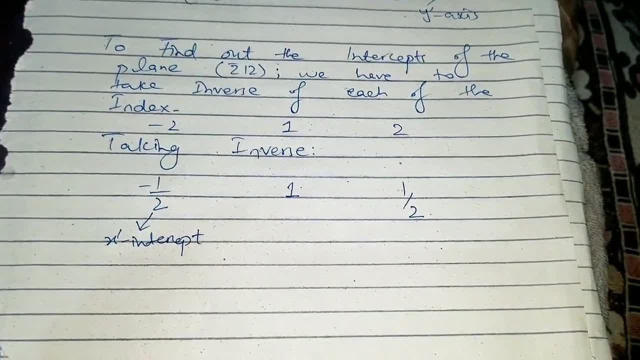 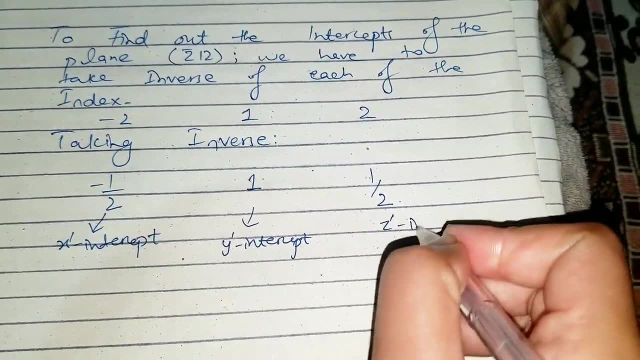 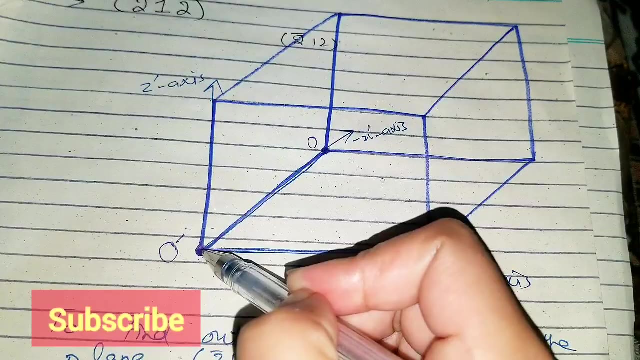 is x prime intercept because the origin that we will use to draw the plane is primed. that is why we are using primed uh names here. so this is the y prime intercept and this is the z prime intercept. all right, so the x prime intercept is minus one by two, which means from origin um along. 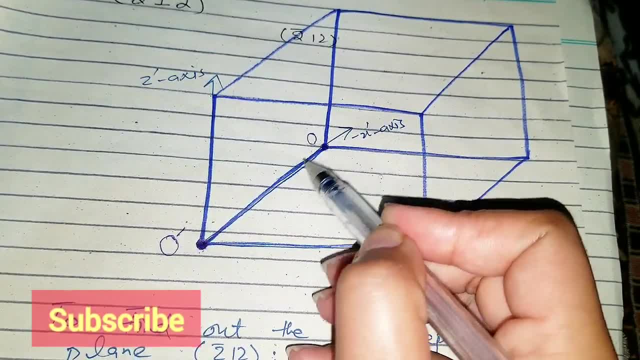 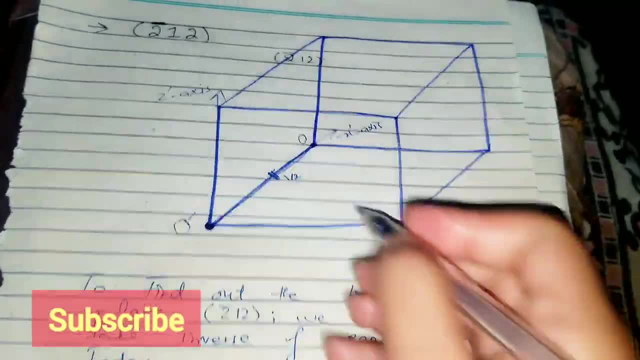 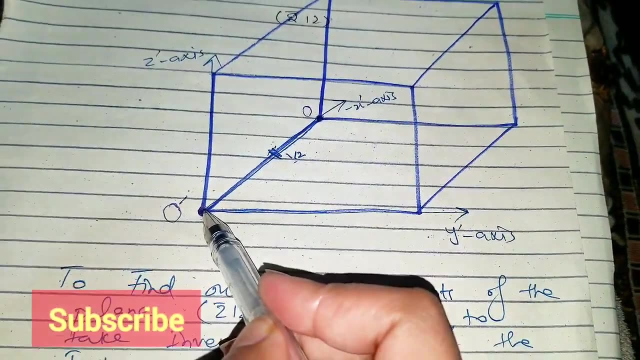 this direction. one means from one corner to the other corner of the unit cell. half of it is like there. okay, it's minus one by two here and one along y prime um direction. so from starting from a region, again, not from this point onwards, it's intercepts and they're always drawn on the axis lines from. 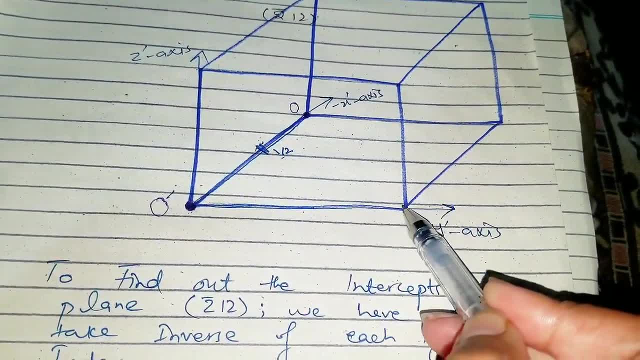 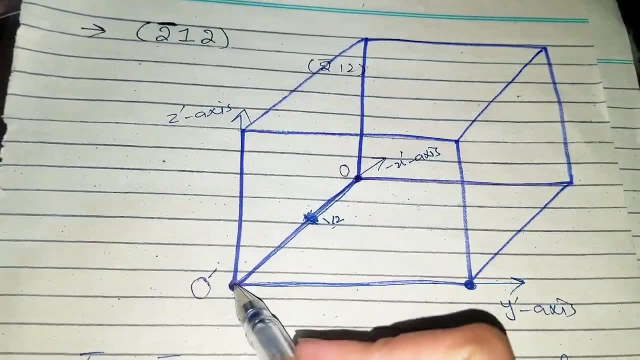 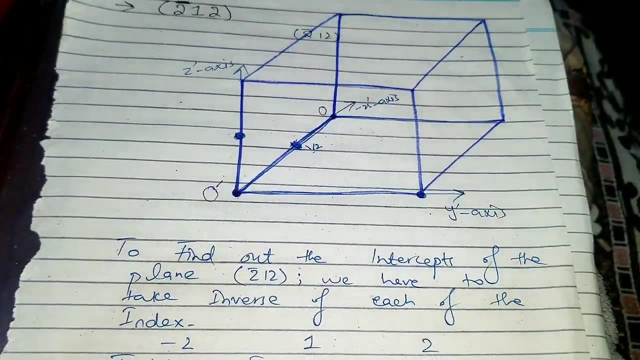 so from origin, one unit along the y direction, which is this point. so this is another point on the plane, okay, and the next one is the half unit along the z direction and starting from origin again, uh, here's somewhere like there, it's the point on origin. okay, now we'll join the three, three points. 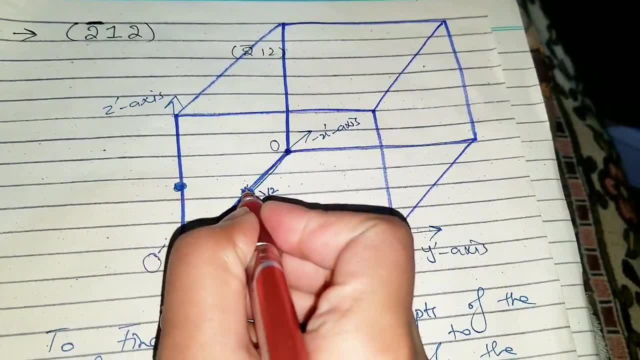 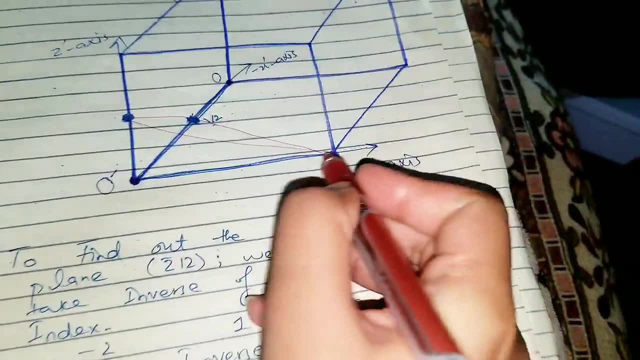 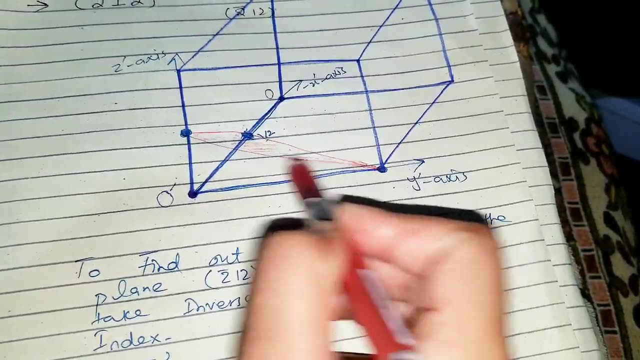 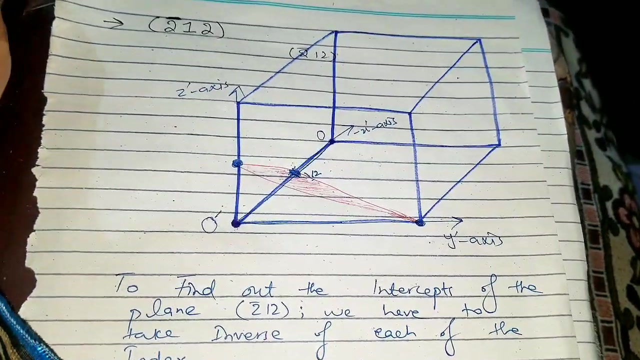 together to get the plane. okay, joining these two lines together by straight lines, um, yeah, something like that. okay, a triangular type of shape and shading it. this was the plane, okay, and the more accurate your cube shape is, the more a beautiful, uh, plane shape you will get. okay, so that is the plane. two by one, two. 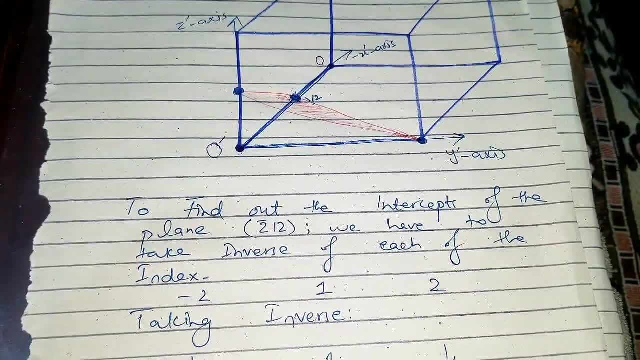 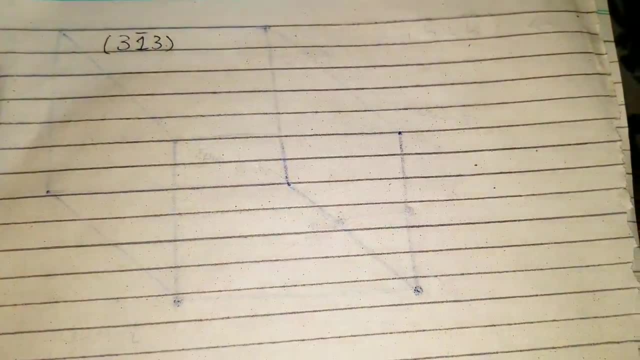 all right. so next problem is, uh, when the y index is negative and that one case is three, one bar three. okay, let us do that one now. so here's the next problem. okay, it's three, one bar three, the y index is negative, and let me draw a nice little cube. 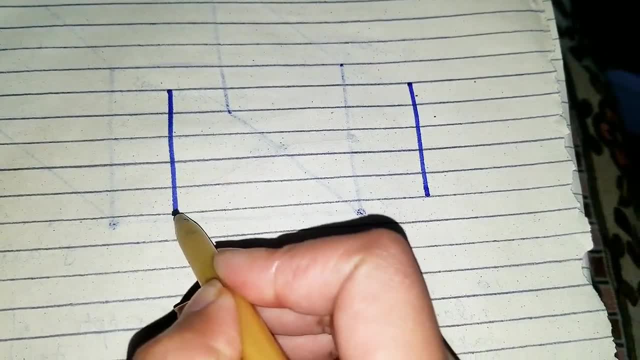 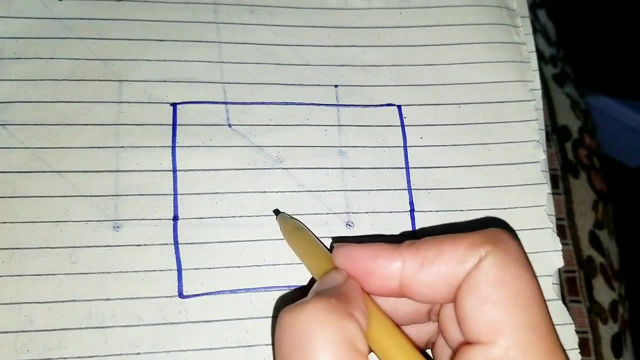 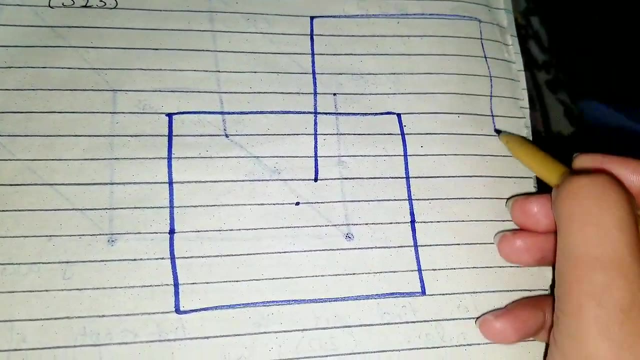 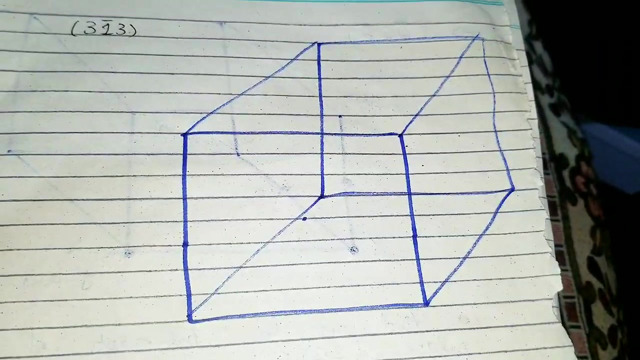 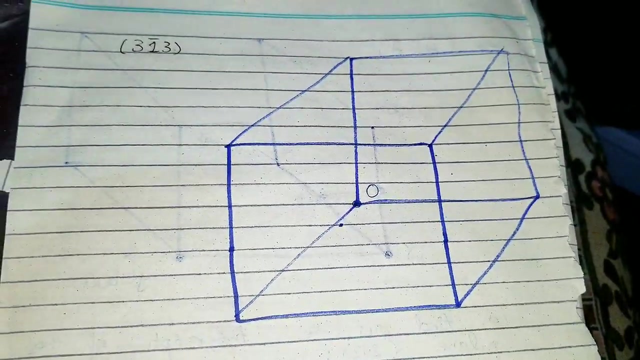 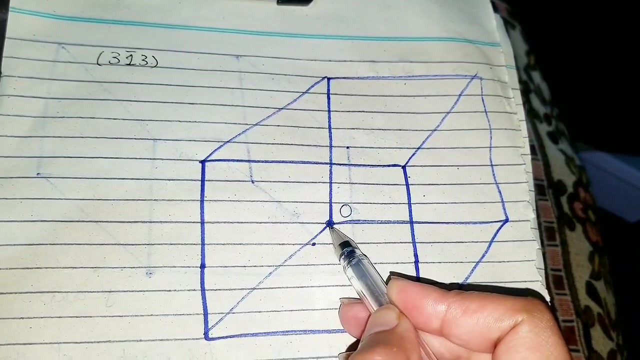 so end of column. okay, so the all positive origin is this one point, that's the all positive or region. now the y index is negative and you have to shift the origin from all positive point to the other corner of the unit cell along the y direction, since the 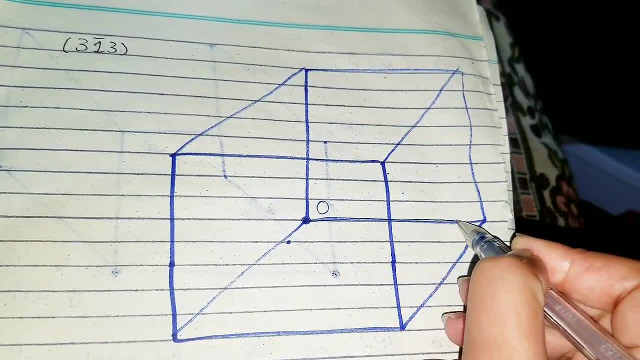 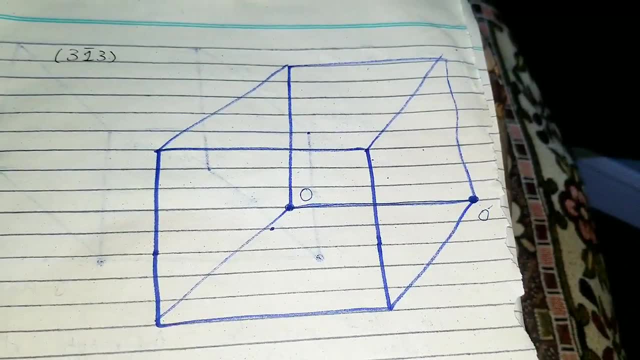 y index is negative, so we'll shift it along this direction to the other corner of the unit cell, which is this point. okay, so this is the new origin o prime that we will be using to draw the plane. okay, so this is a new region and this is one of the line connecting to the origin point. this is: 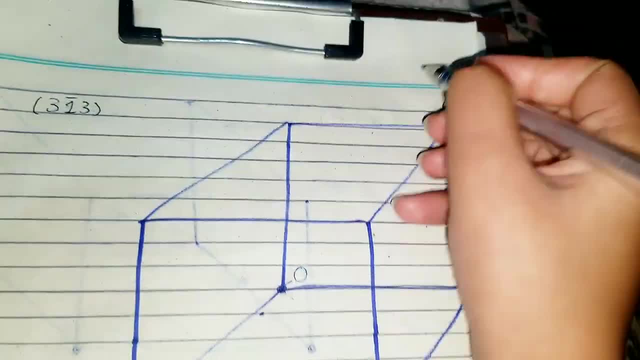 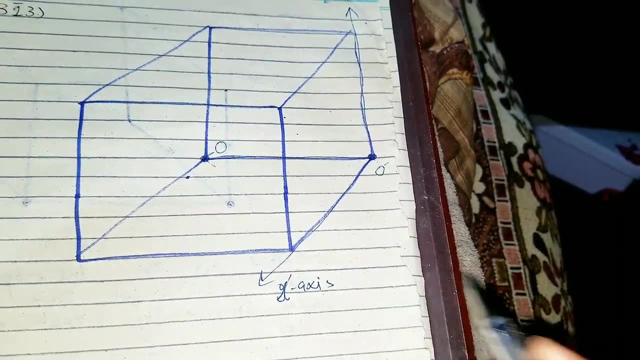 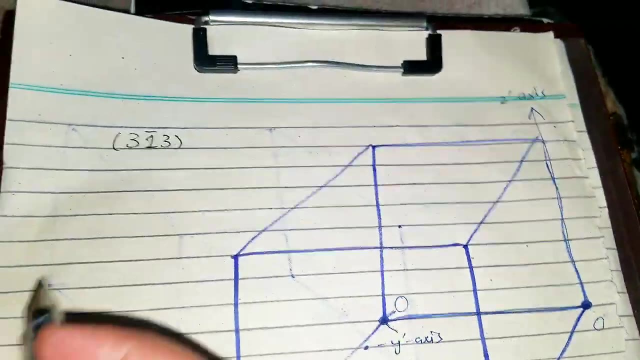 another line, and this is the third line. this is the z prime axis. positive z prime axis, this is positive y- sorry, x prime axis. this is positive x prime axis and this is negative y prime axis, since the y index was negative. okay, so now we'll take the inverse. okay, you have to write the same thing. 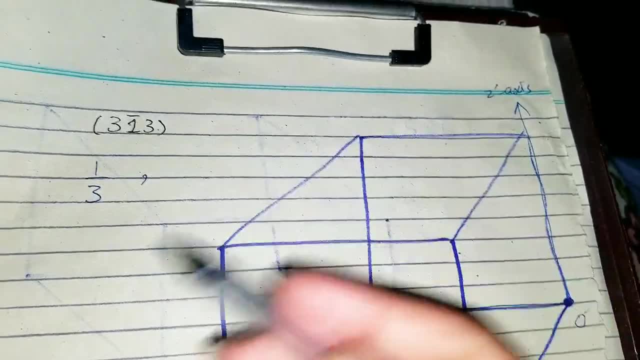 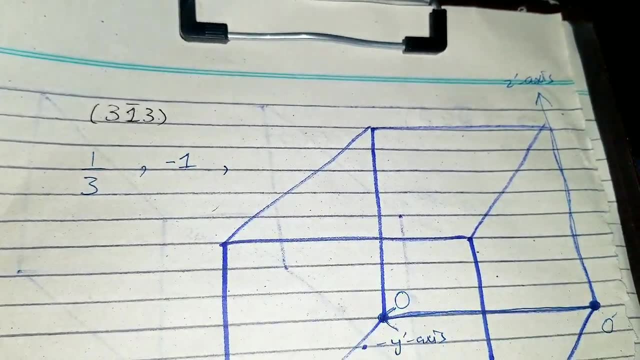 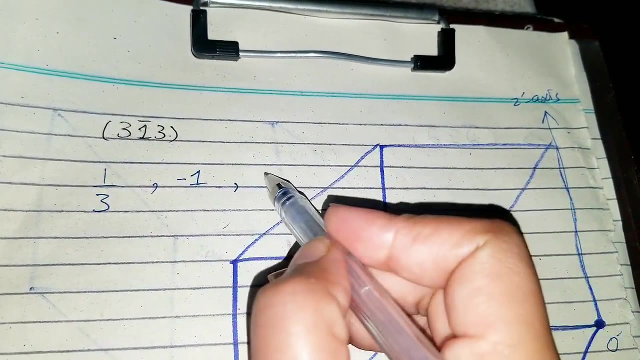 that i wrote for the previous problems, when you are like solving it for exam. so we'll take the inverse of the miller indices in order to find out the intercepts of the plane. so inverse of 3 is 1 by 3. inverse of minus 1 is again minus 1. inverse of 3 is 1 by 3. so this is the x prime intercept. this is y prime. 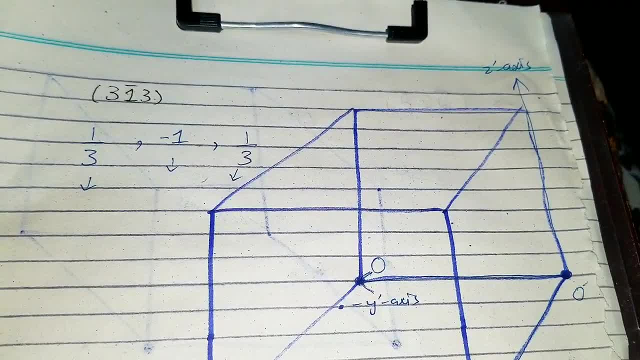 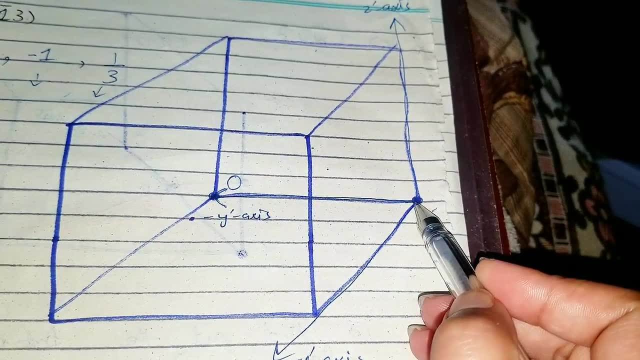 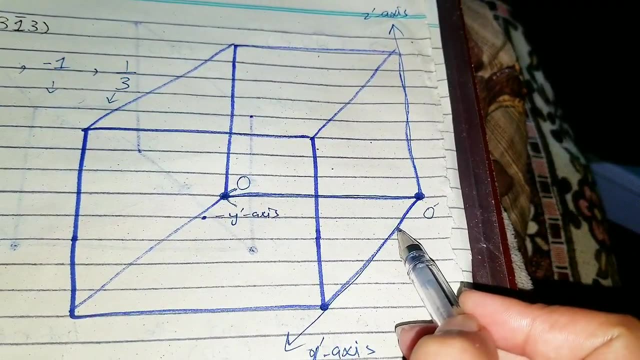 intercept and this is a z prime intercept. okay, so x prime intercept is 1 by 3. so from origin, new origin, 1 by 3 is the x intercept. so we'll divide this whole length. this whole length from one corner to the other corner of the unit cell is 1 and we'll divide it into 3. equal power to get. 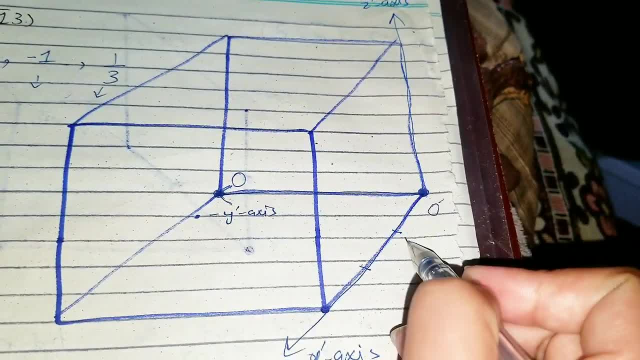 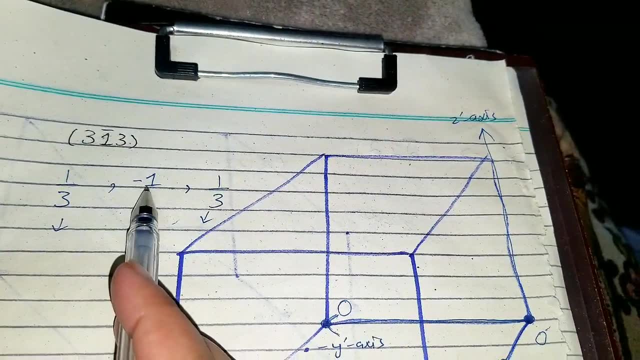 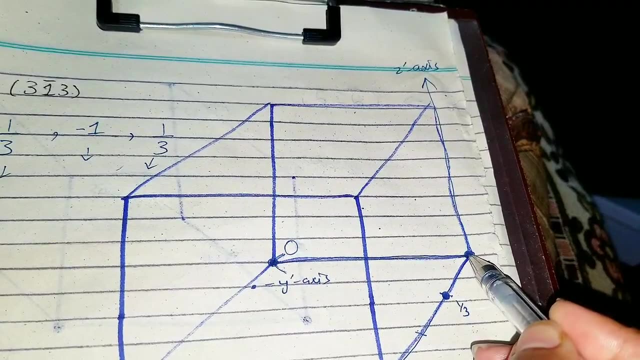 the one third power. so this is roughly that, okay, and this is the one third power. so this is one of the point on the plane, this one, okay. next is minus 1 intercept for the y direction. so from origin, new origin. okay, this is the new region, again starting from the origin, one unit along y direction, which 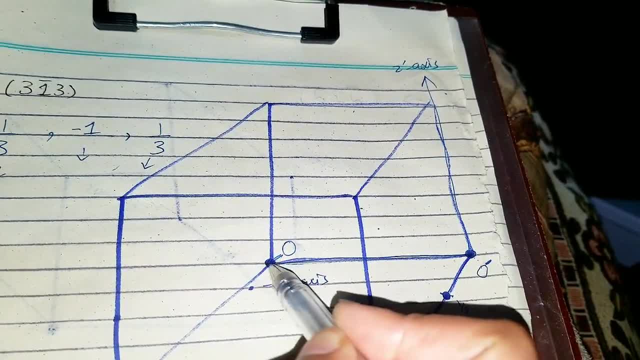 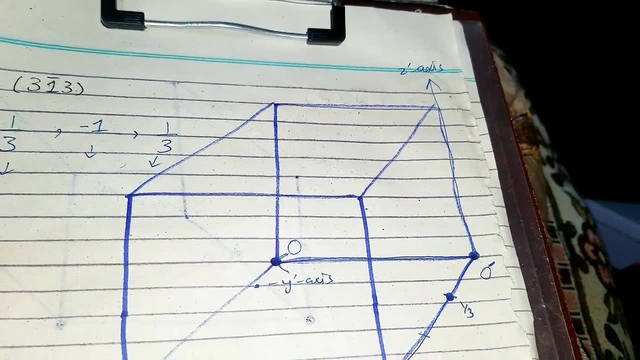 is this minus 1? okay, so this is the another point on the plane, this one point and these two points are the points on the plane. now the third one is 1 by 3 along the z direction. so this is the z direction, so this whole length from one corner to the other corner of the unit cell, starting from 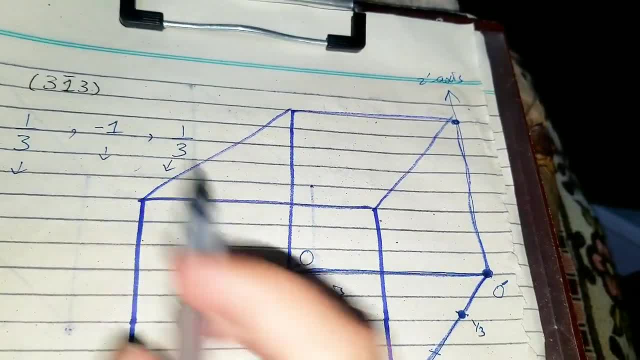 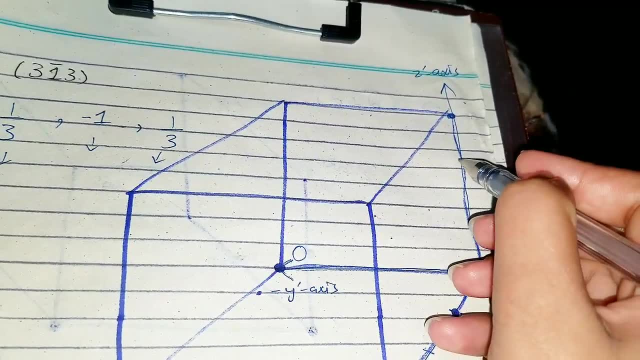 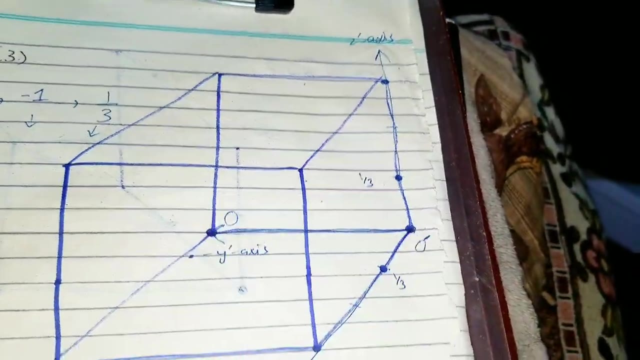 the origin. okay, uh, you always draw these points on the axis lines and they're always drawn starting from the region. okay, so, starting from origin, we'll divide this whole length into three equal parts. equal parts- and this is the point 1- by 3. okay, this one, this one and this one. these three are: 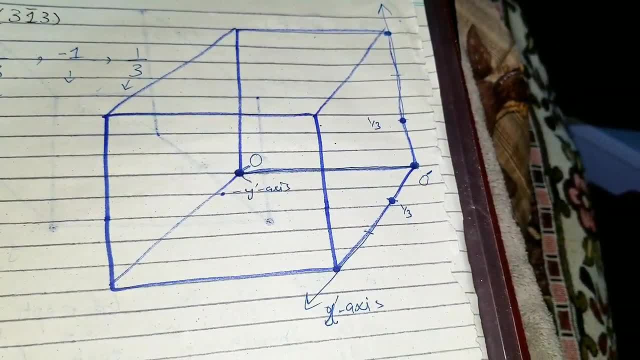 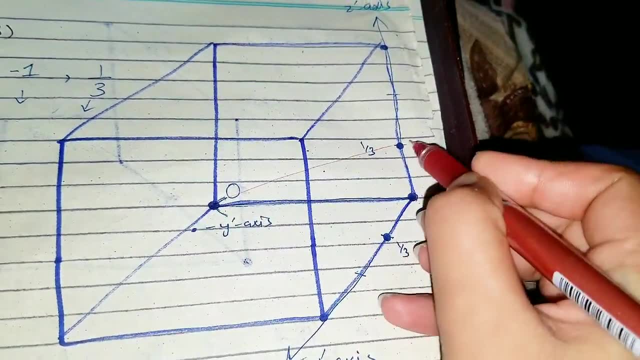 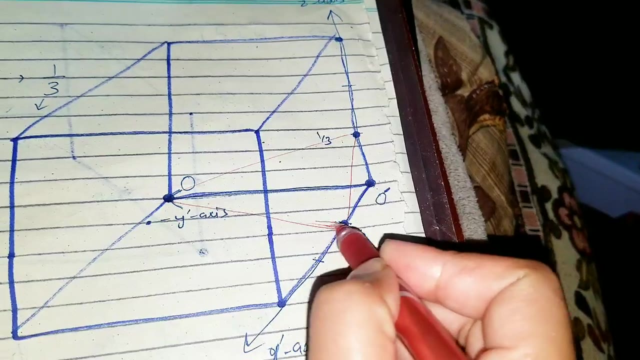 points are the points on the plane, and we will join these three points together in order to get the plane whose miller indices is 3, 1 bar 3. okay, so we'll join these three points together by straight lines and here we go. okay, it's on this one, we'll shade. uh it, okay with the same color. 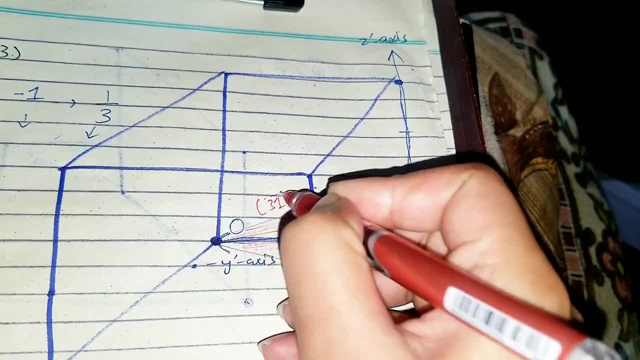 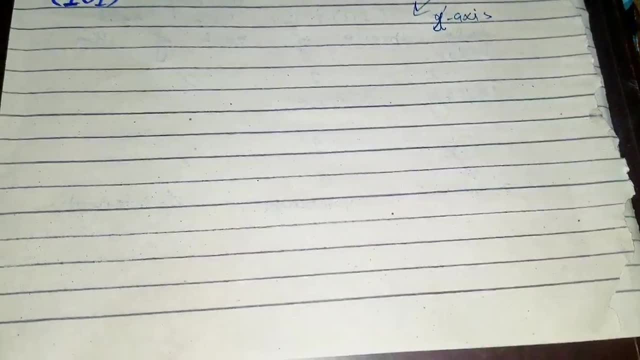 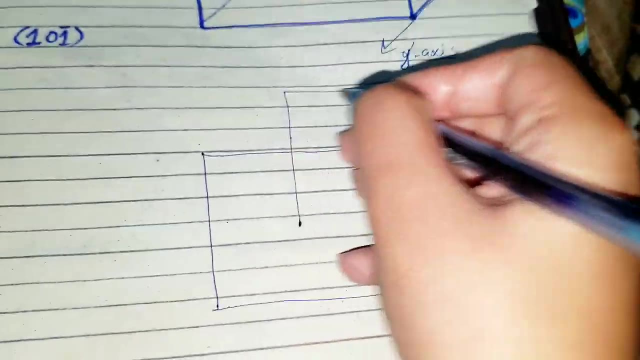 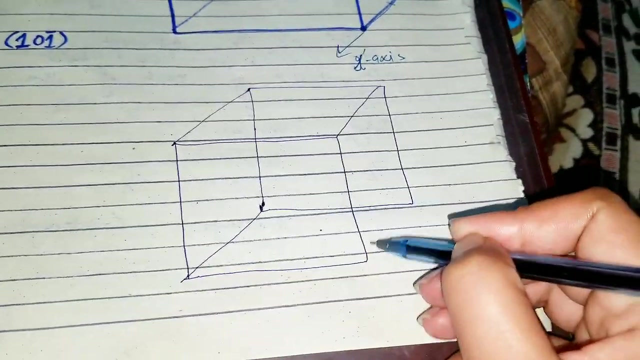 and, yeah, that's the plane. 3: 1 bar 3. okay, that's done. here's the next problem. here the z index is negative. okay, and uh, first of all, we'll draw the cube. okay, here's a small little cube, because all of the lengths are one. so that is why the small cube will surface. and this is the all positive. 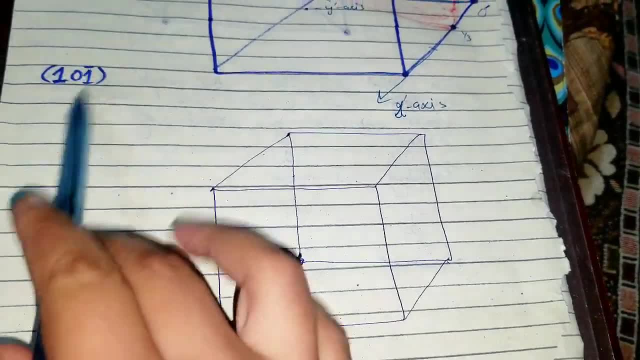 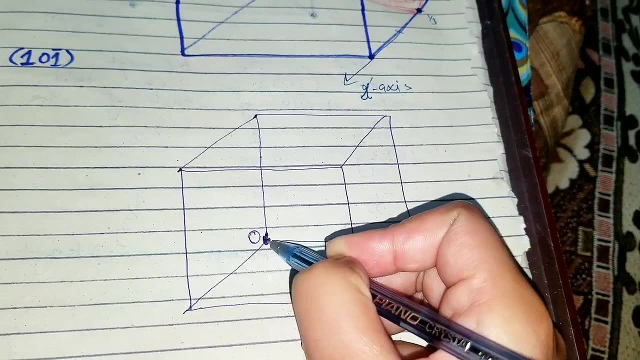 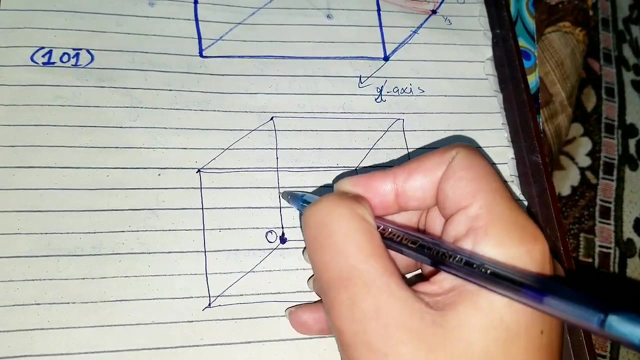 origin, okay, and you have to shift the origin because the z index is negative. and since the z index is negative, that is why we have to shift the origin from all positive point, uh, by one unit along the z direction. so this is all positive origin point and one unit means to the other corner of the unit cell along the z direction. 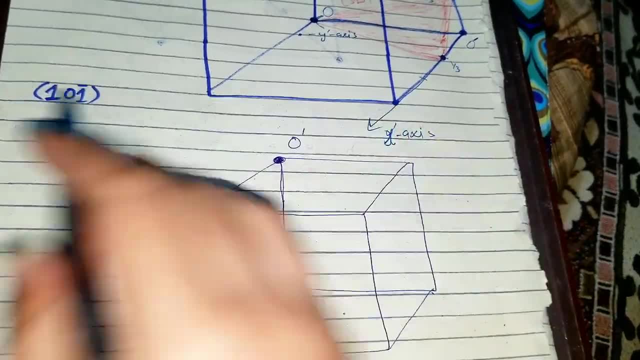 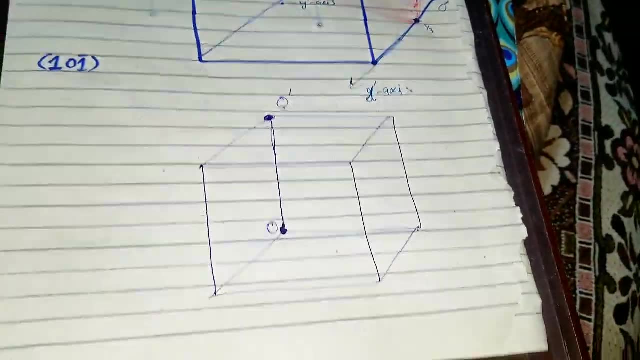 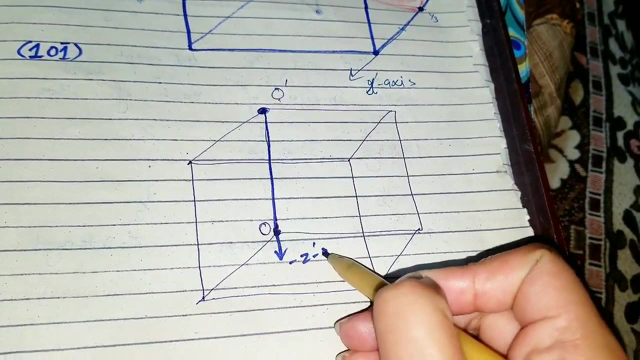 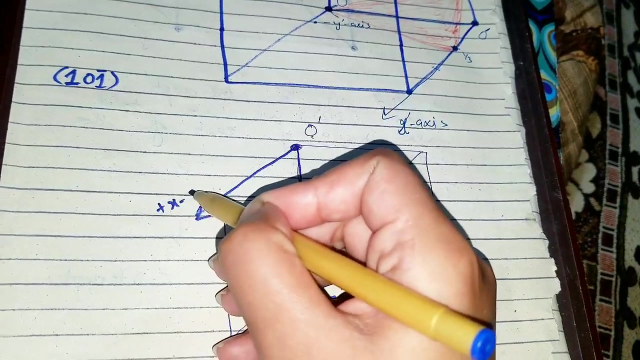 which is this point. so, since the other two indices are not negative, that is why this is the final origin- okay, and this origin will be used to draw the plane. um, okay, and the axis lines are: this one line is the negative z prime in axis- okay, since this index was negative. and this is the positive x prime axis: okay, since the origin is: 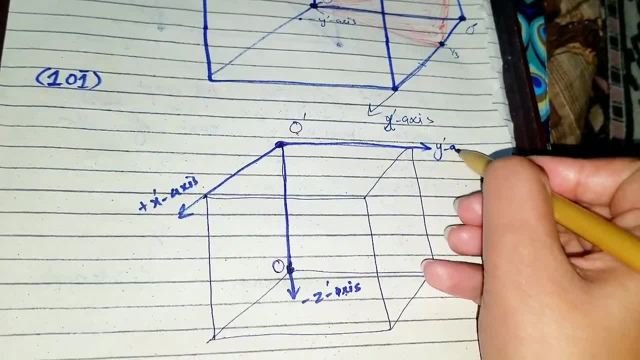 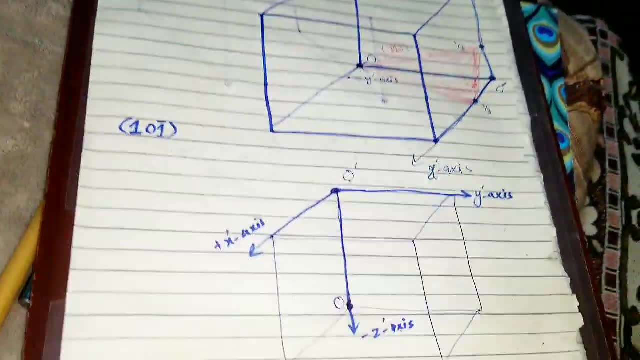 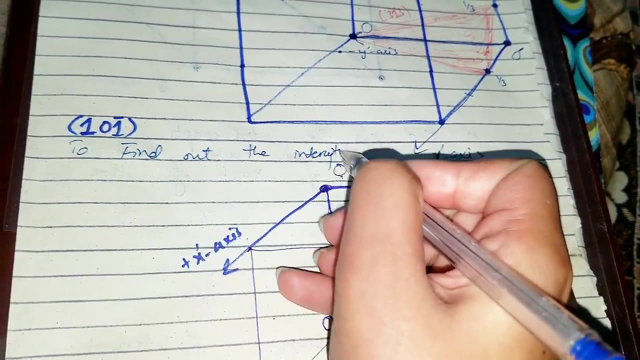 prime. that is why we are using primed word and this is the y prime axis, positive y prime axis. and uh, now we we need to find out the intercepts of the plane. so to find out the intercepts of the plane, plane one zero, one bar. 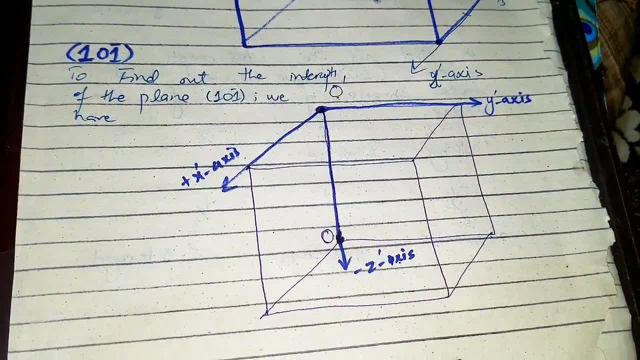 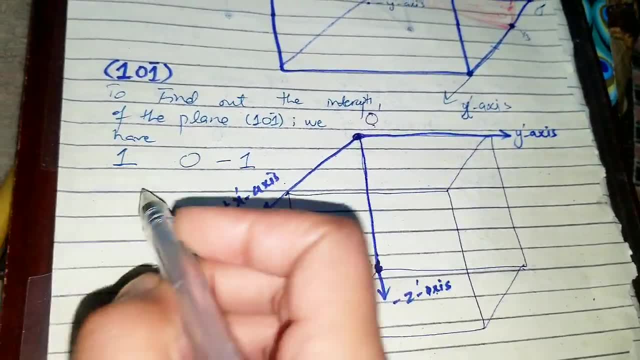 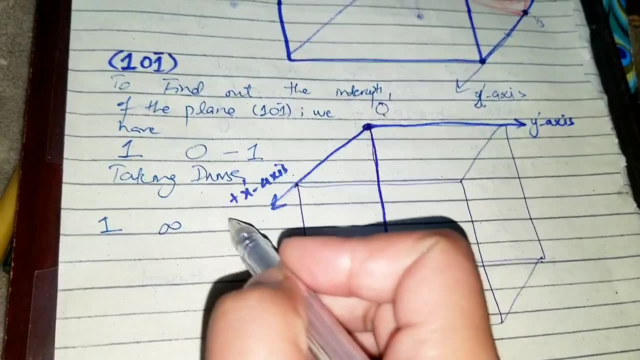 we have to take the inverse of each of the index, so you have to write it right there. okay, now we'll take the inverse of each of the index and these are the three indices: one, zero, minus one. so taking inverse: inverse of one is one, inverse of zero is infinity. inverse of minus one is minus one again. 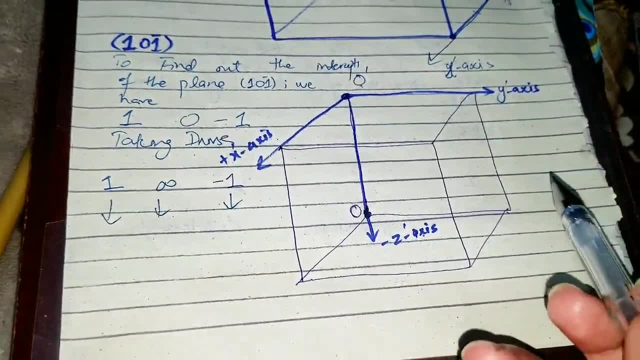 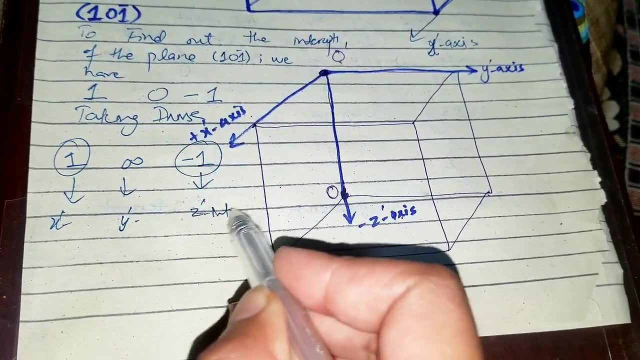 so, uh, we deal with the infinity intercept at the end, and first we'll consider the ones which are not infinity. this is the x prime intercept, this is y prime intercept and this is the z prime. okay, so x prime intercept is one. so, starting from the origin, from the new region, that, uh, 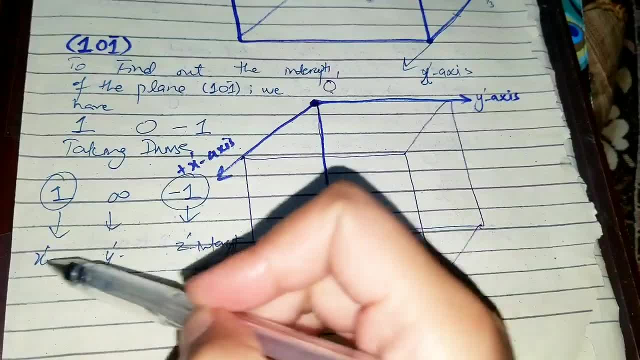 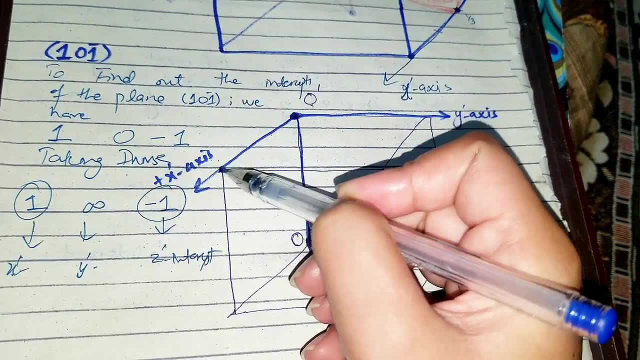 we have selected um one point, one unit along the x direction. okay, since x intercept is one, so the point one is to the other corner of the unit cell along the x direction, which is this point. so this is one of the point on the plane. all right, so the next is the z prime intercept, which is minus. 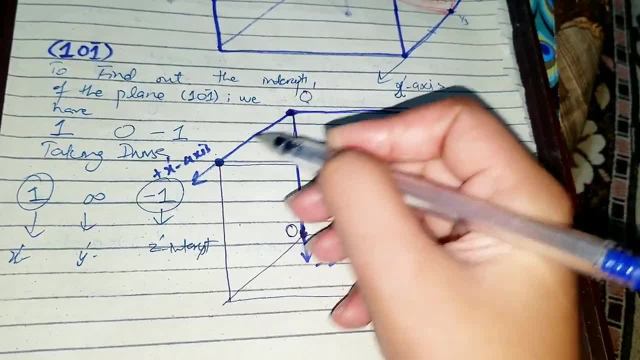 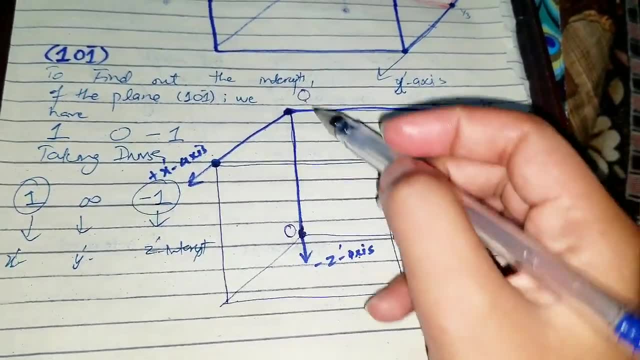 one. so starting from the origin again. okay, not from that point onward. starting from origin all again, because, uh, intercept is a point on the axis line. okay, that is starting from origin. you'll get that point. so it's minus one, which means to the other corner of the unit cell, along the negative. 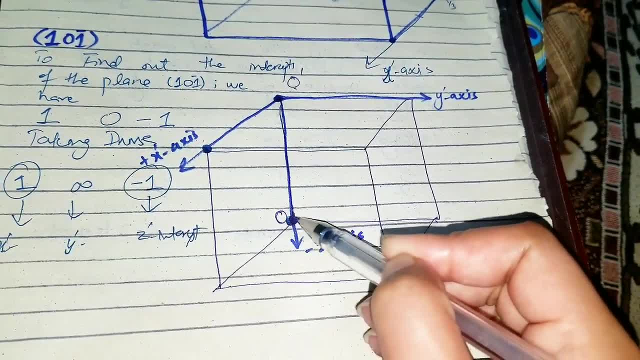 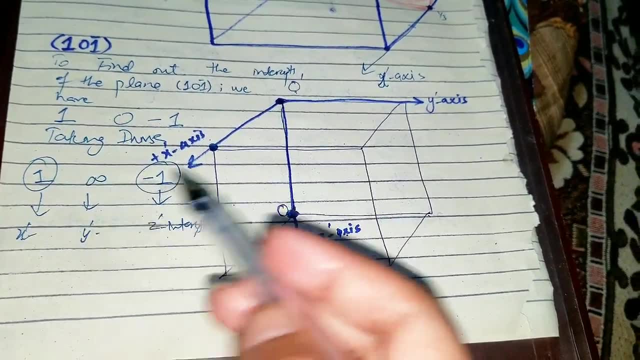 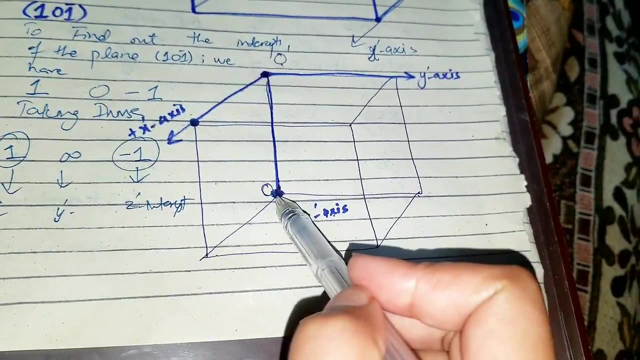 z direction, which is this point. okay, so this is another point on the plane, all right, since the y intercept is infinity, uh, so, uh, we'll deal with that by drawing a parallel line from each of these two points that we have got, okay for the plane. um, along the y direction. so from: 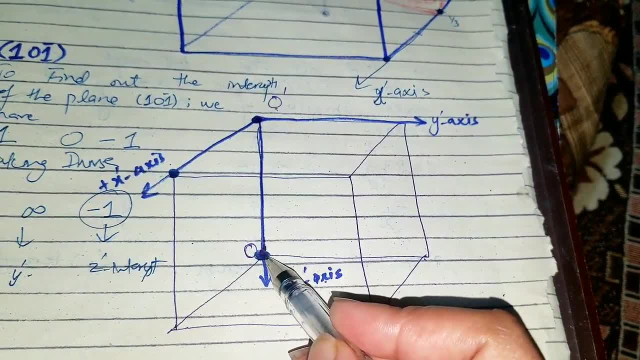 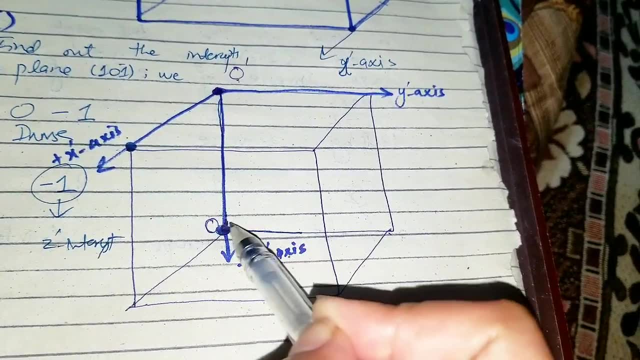 this point, we'll draw the parallel line along the y direction and this parallel line will end up to the other corner of the unit cell. okay, so this is the y direction and we'll draw a parallel line along the y direction, which is starting from this point that we have got, uh, from these intercepts. 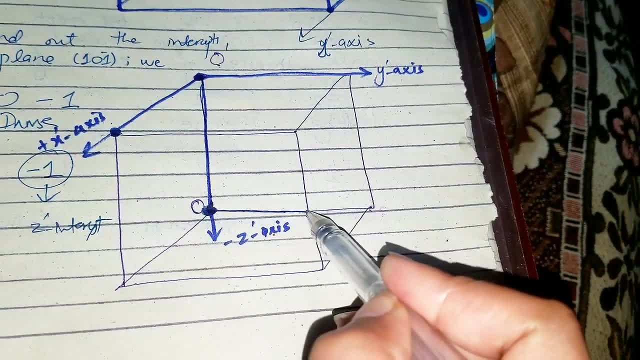 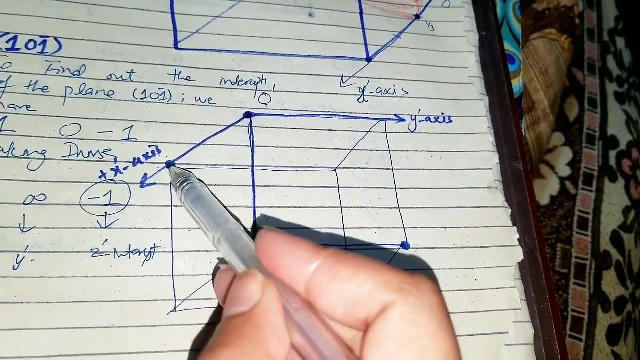 okay, these two intercept points, so parallel lines along the y direction, will stop to the other corner of the unit cell here. okay, this is another point on the plane now. okay, so this is another point on the plane and we'll draw parallel along parallel lines along the y direction, which is: 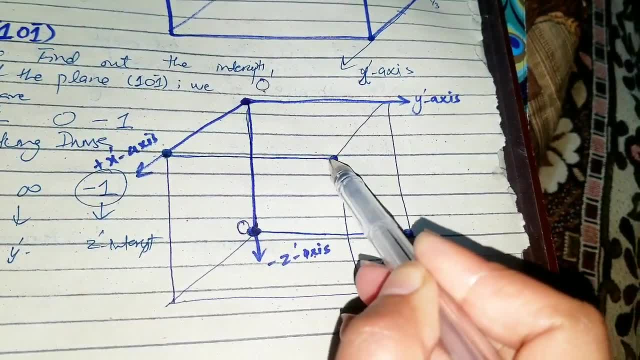 along this point and we'll draw a parallel line along the y direction and we'll draw a parallel line along the y direction, and we'll draw a parallel line along the y direction and we'll draw a parallel line along one pin, um, along this line, okay, and we'll end up at the other corner of the units, which is: 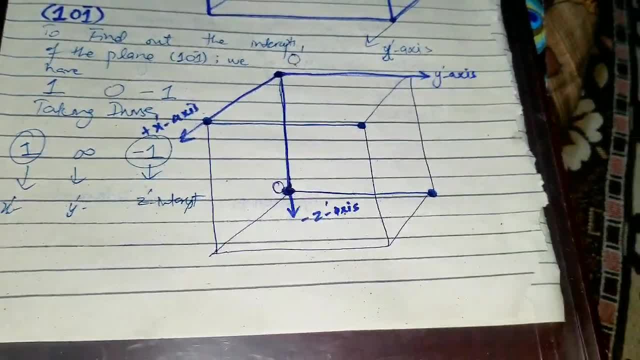 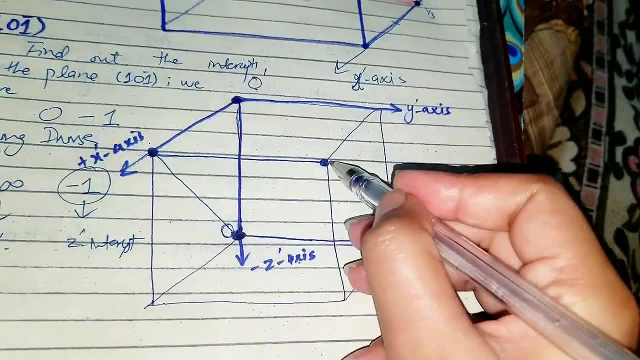 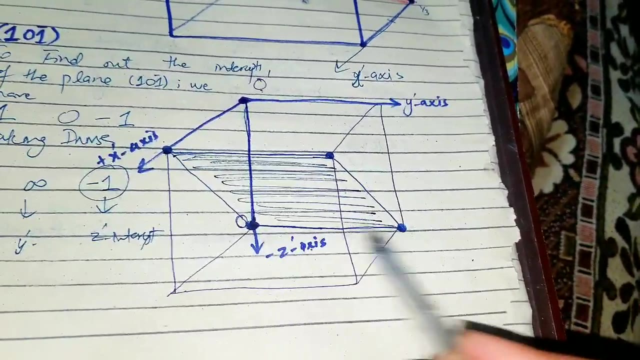 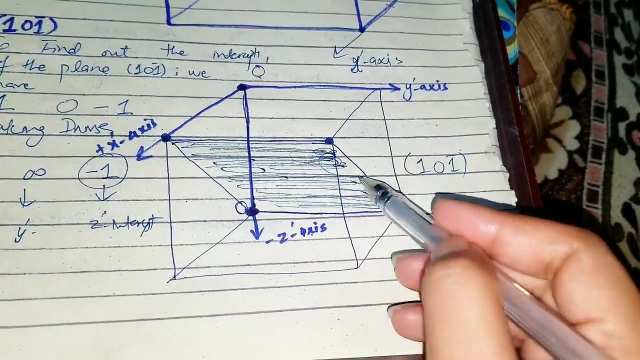 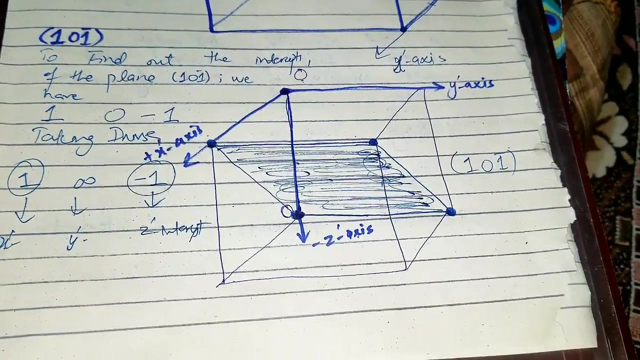 this point. now, these four points are the points of the plane and we will join these lines together, this line with this one. okay, and we'll shade these. this is the plane one zero one bar. all right, this is the plane one zero one bar. okay, this is done now, and now we'll do the case when two of the indices are negative. 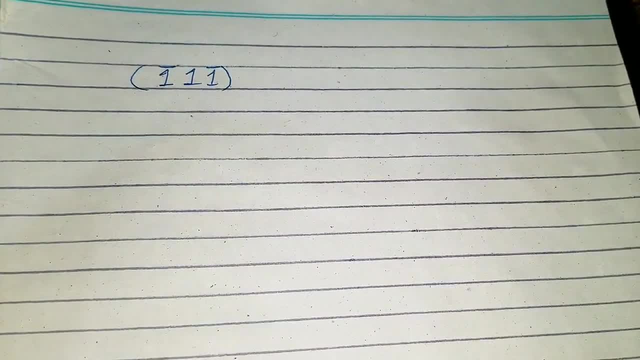 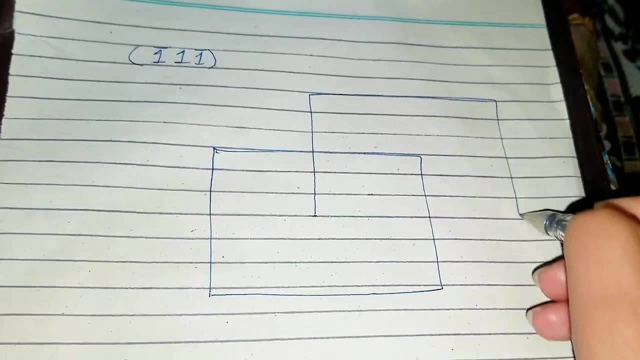 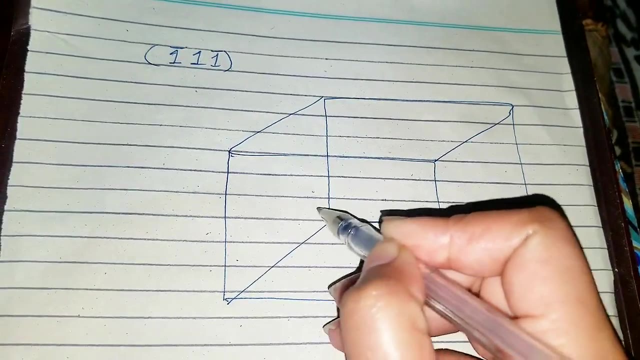 here comes the next problem. it's one bar, one one bar. x and z indices are negative. okay, so let me draw the cube first. it all starts with a all positive origin, which is this point. this is the all positive origin that cannot be used for drawing this plane. okay, we want to draw this plane. 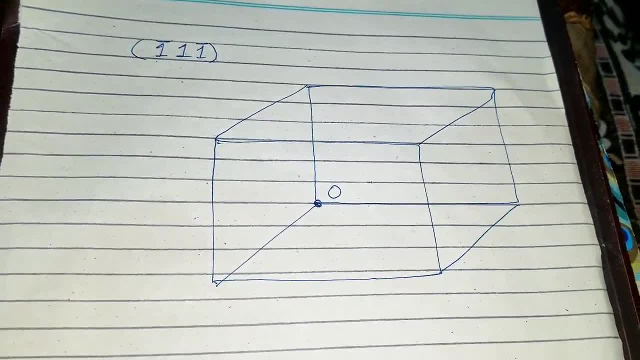 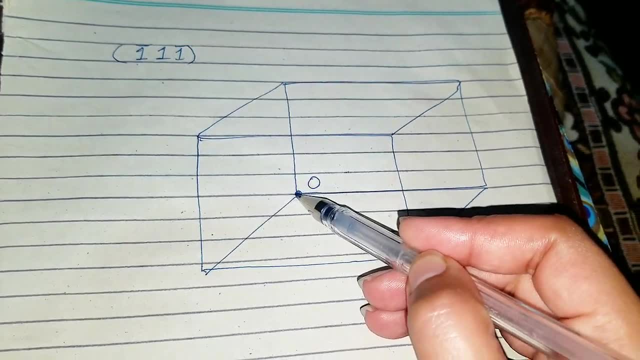 inside a single unit cell and for that purpose we have to shift the origin, and x index is negative. so first of all, starting from the all positive origin, we'll move one unit along the x direction, which is this point. okay, regardless of this numerical value it could have. 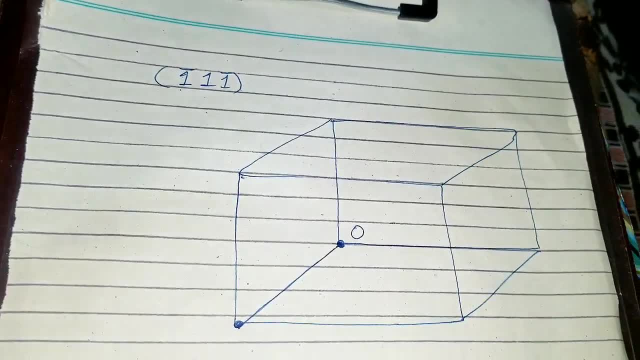 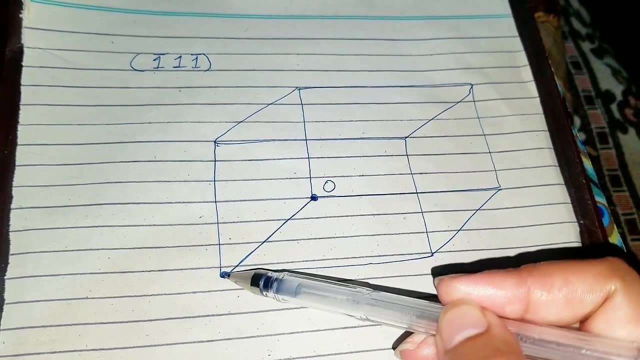 been two bar, three bar or whatever it is, we always move one unit along that direction which is having a negative value in this index. okay, so, from origin, one unit along the x direction, and this could not be the final origin point, because the z index is also. 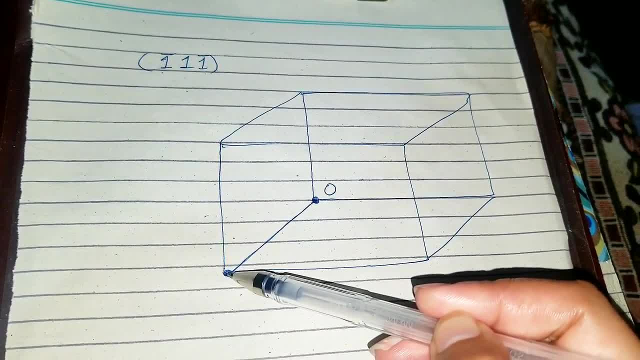 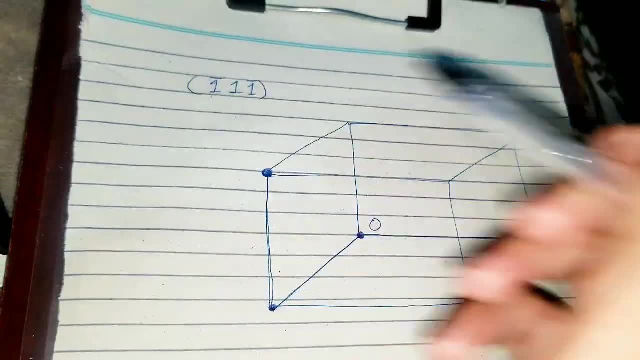 negative. so from this point onwards we have to shift the origin one unit along the z direction, since that one has the negative index. so that one point is the final origin, because the y index is positive and no more shifting is required along the y direction. so this is the final origin, okay. 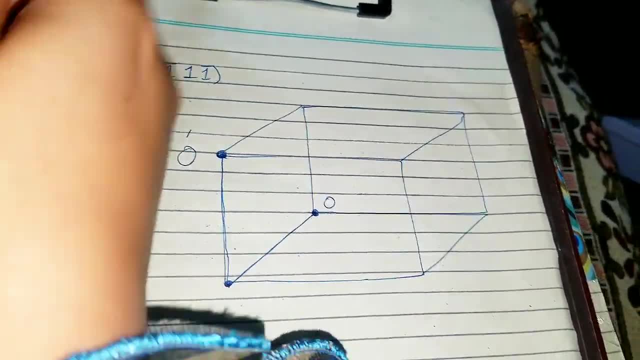 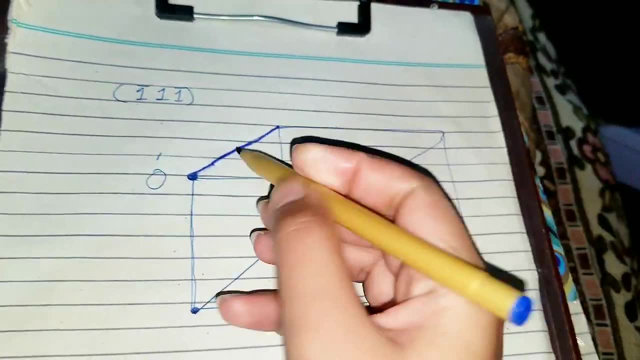 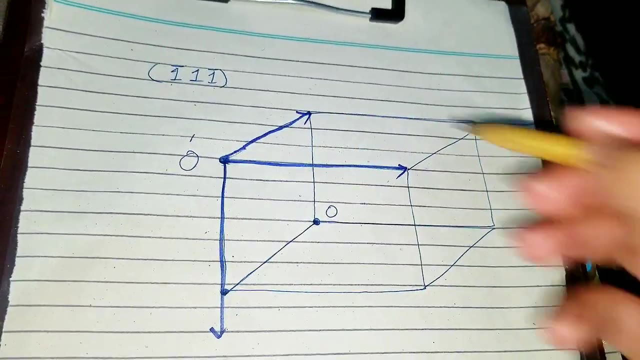 and this is a new region that will be used to draw this plane. and let us now draw the parallel, draw the axis lines and they are the three lines that are joining this point. and these are the three lines, okay, and these lines joining- uh, that origin point is- are the axis lines. so this one line is the negative x prime. 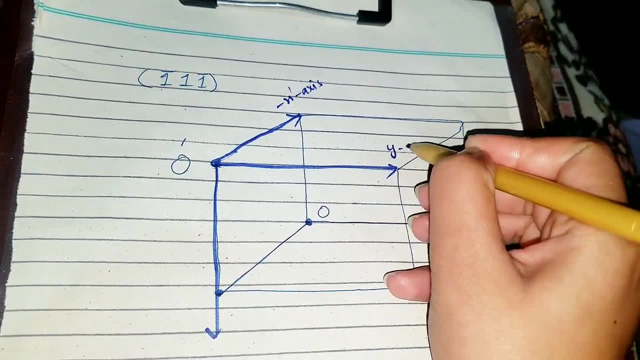 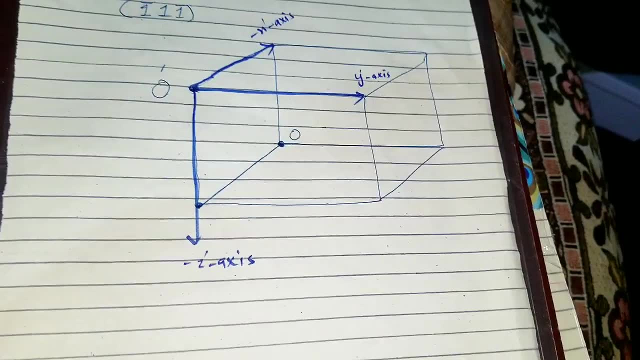 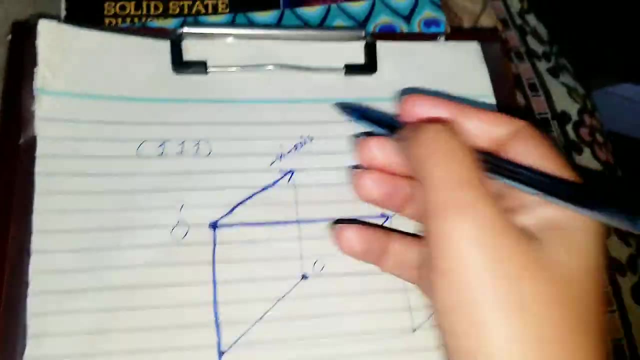 axis. okay, this one line is positive y axis, y prime axis, and this one line downward is z prime axis. okay, so negative z prime axis. now, next, what we have to do is to draw the intercepts and to find out the intercepts and to find out the intercepts. to find out intercepts, you have to. 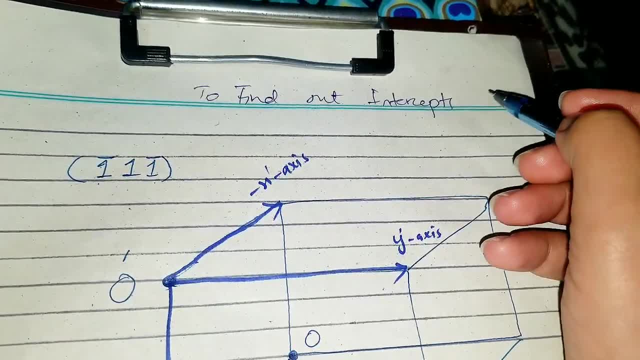 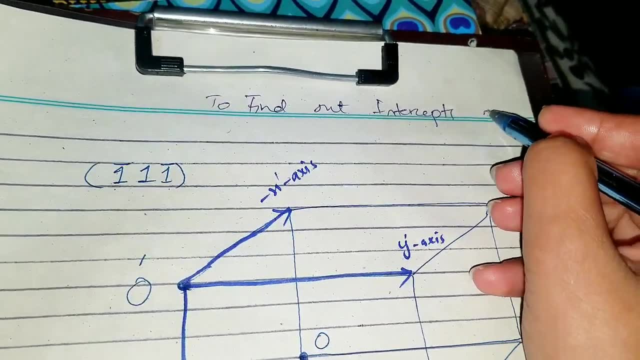 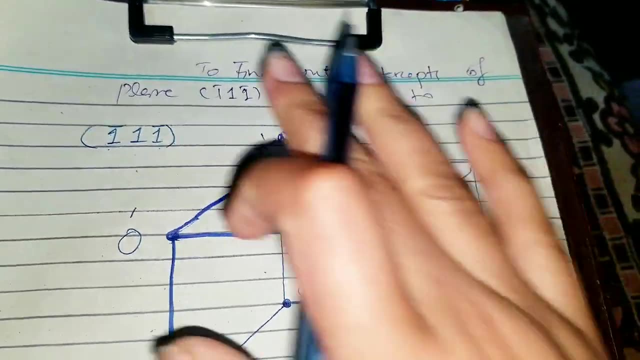 write this line either here or here. okay, i'm writing it here because, um, i have some vacant space right there and i want to make use of all the space now to find out the intercept of plane. one bar, one, one bar. we have to take the inverse of each of the index. you'll write it, okay. 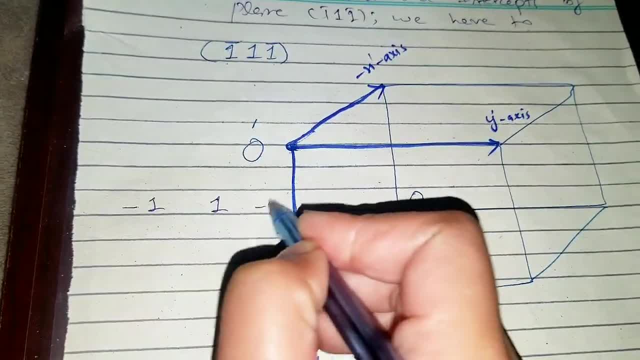 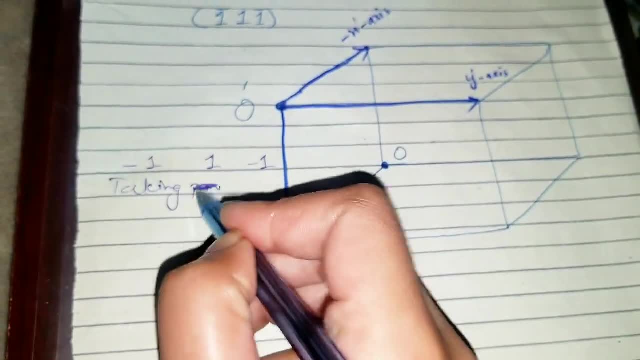 so after that, uh write these miller indices here, write the operation that you are going to process, that you are going to uh do. that is taking inverse. okay, we'll take the inverse of minus one, which is minus one. again, taking inverse of one, which is one. 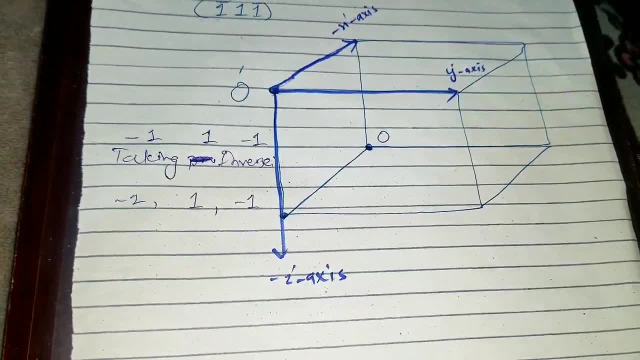 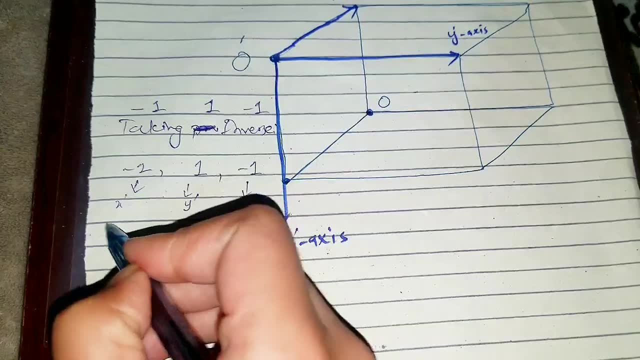 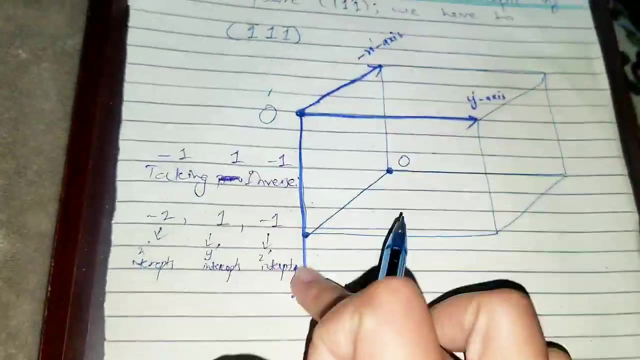 again, taking inverse of minus one, which is minus one again. okay, so this is x prime intercept, this is the y prime intercept and this is the z prime intercept. okay, these are the intercepts and they are drawn on the axis lines. okay, intercepts are the points on the axis lines and these are the. 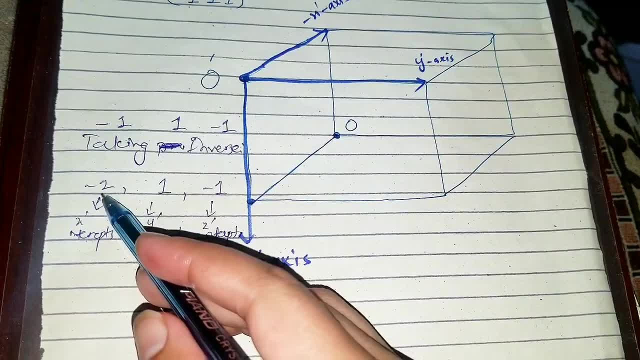 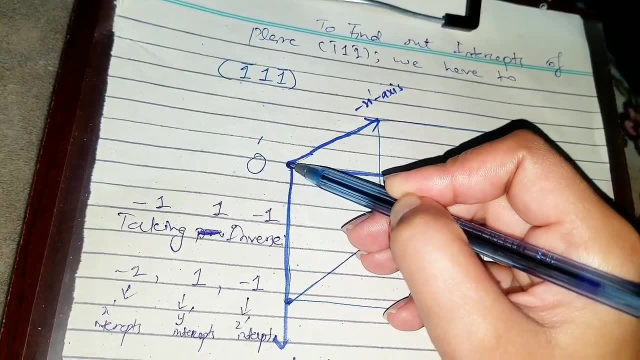 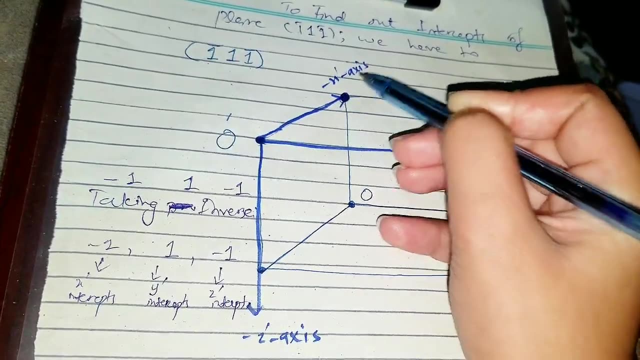 axis lines. okay, so x prime intercept is minus one. okay, so starting from this new region and x prime intercept is minus one, means to the other corner of the unit cell along the negative x direction, which is this, this point, this one pretty little point. now, next intercept is y prime. 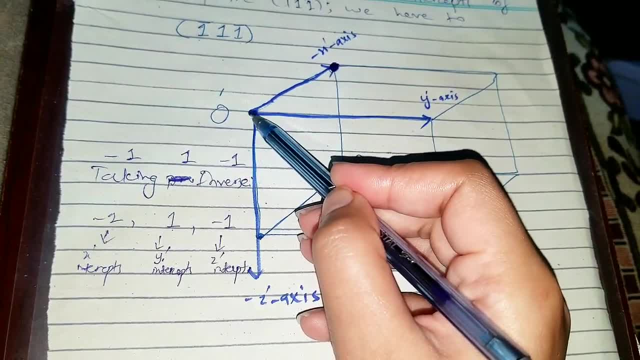 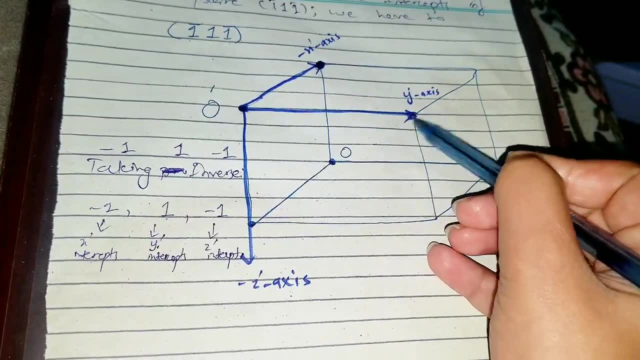 intercept starting from origin again, okay, all over again- and along y prime direction, to the other corner of the unit cell, which is this point, another point on the plane, and starting from origin again. z intercept is minus one, which means to the other corner of the unit cell, along the 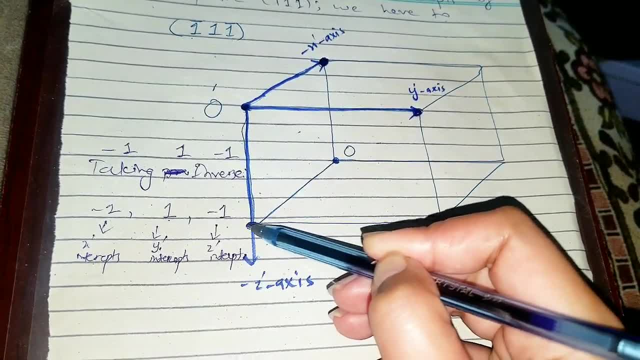 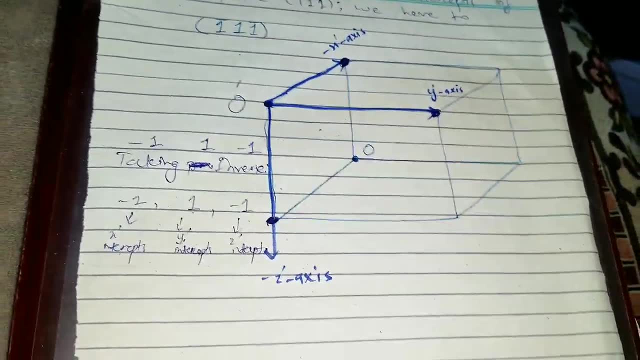 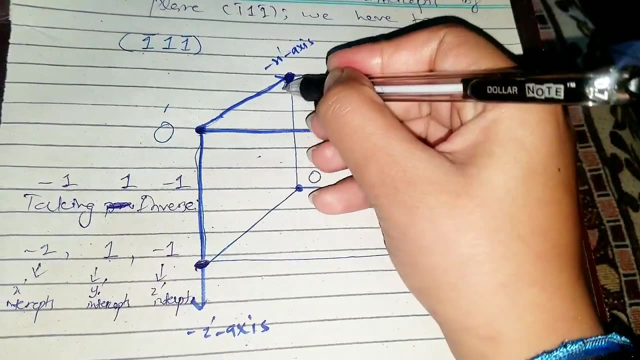 x direction, negative y, negative z direction, and this is this one, negative z, prime direction. and this is another point on the plane, this one, this one and this one. these are the three points on the plane. now we'll join these three lines. oh sorry, these three points together, like that. 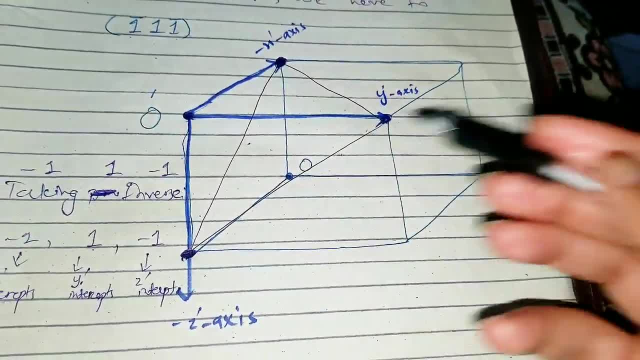 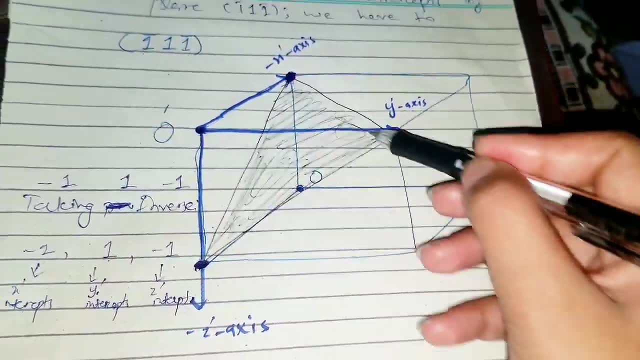 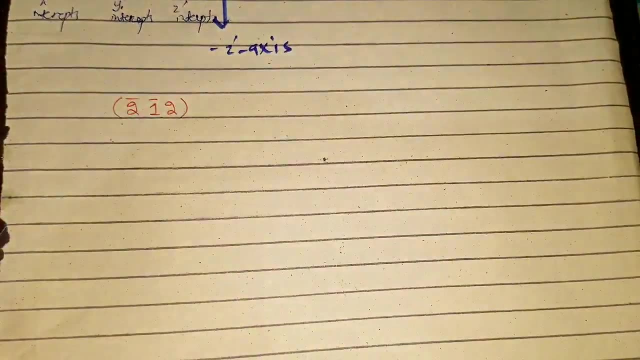 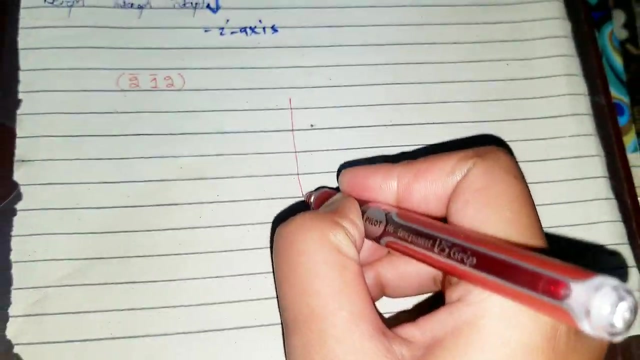 okay, and this pizza slice is our plane and if you want, then you can eat it also. all right, so this is done. here is the next problem. here, the two of the indices are negative, which are the x and the y index. so i will do that one problem also, and after that we'll do the all. 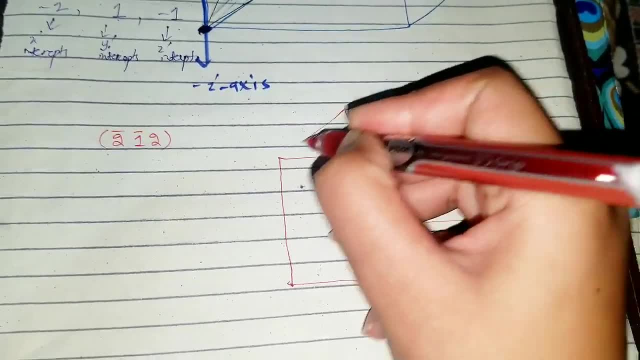 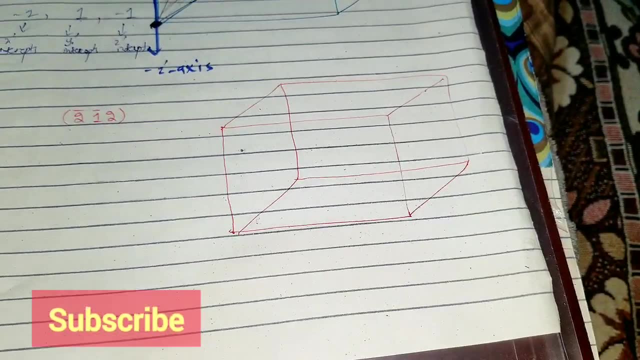 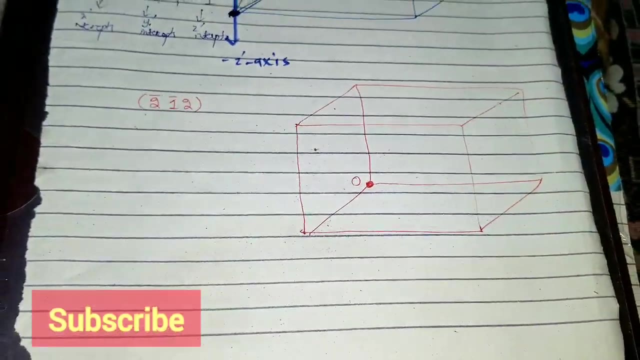 negative mla indices case. okay, so this is our cute little cube. okay, and i doubt that it will create a problem because it's very little. so, yeah, this is the region, all right, and uh, we have to shift the region. okay, the x index is negative and the y index is. 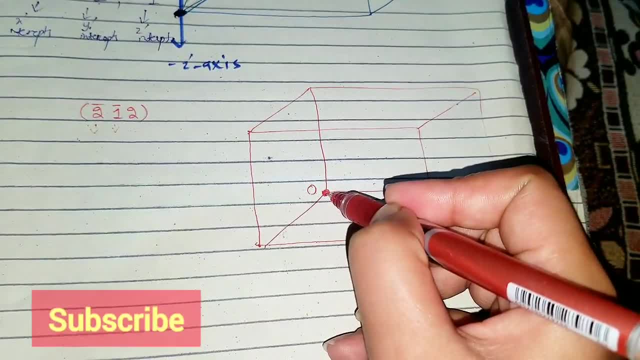 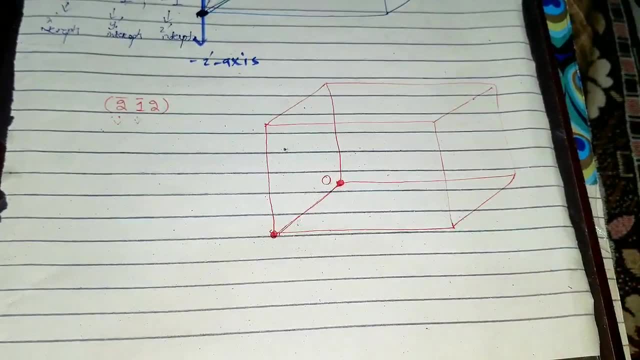 negative. so, starting from the all positive origin, we have to shift the region one unit along the x direction. six, since the x index was negative. okay, and that shifting is always done by one unit. okay, regardless of this numerical values, that is there. these numerical values doesn't. 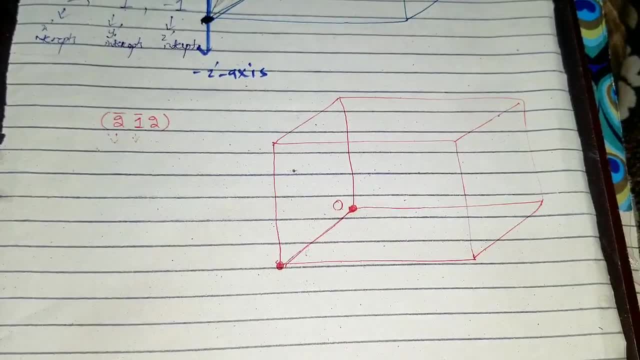 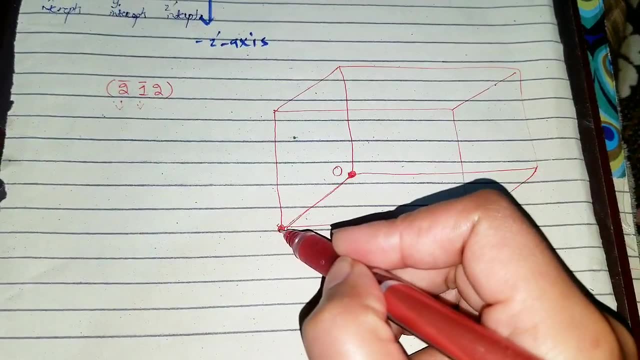 affect the position of origin that we select. okay, the shifting of region is always done by one unit. okay, regardless of this value, the negative nature only matters. so from this point to the other corner of the unit cell, along the x direction, we have shifted the origin. now, this is not the final origin point, because the y index is also negative. so we have. 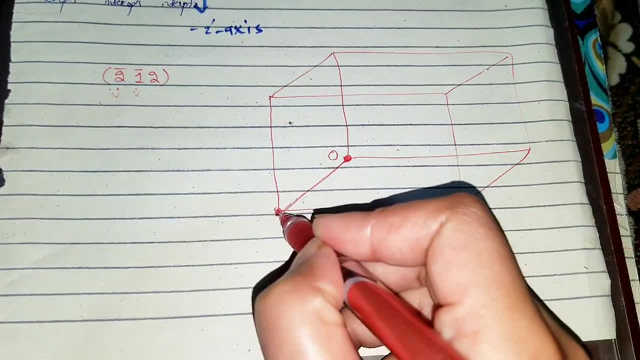 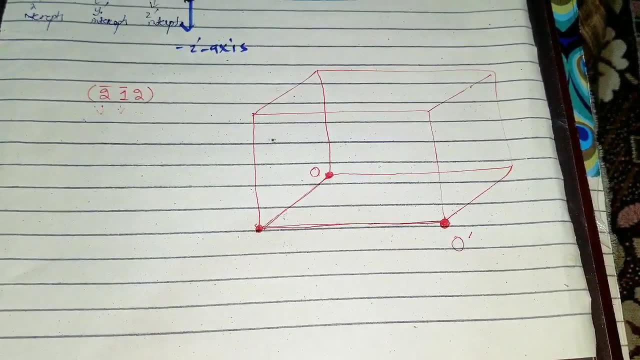 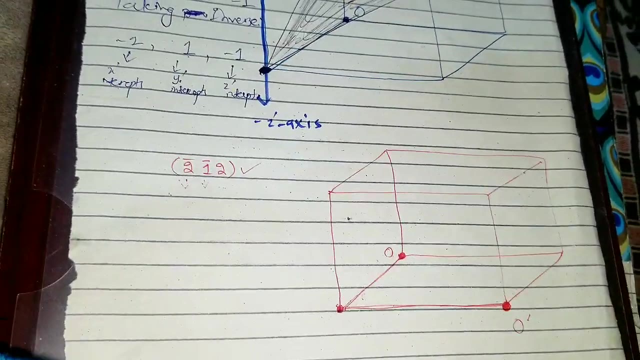 to shift our region, uh, onwards from this point uh, along the y direction, by one unit, which is this point. okay, so this is the final point, uh, final region o prime that we'll be using to draw this plane. okay, so this is the final origin, and let us draw the axis lines, because actually axis 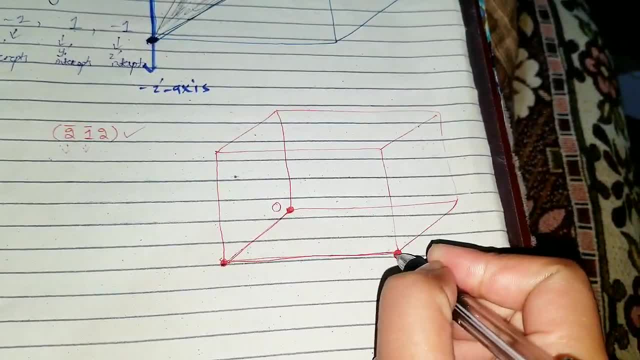 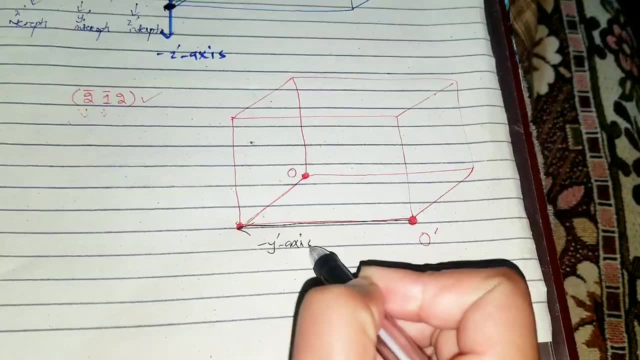 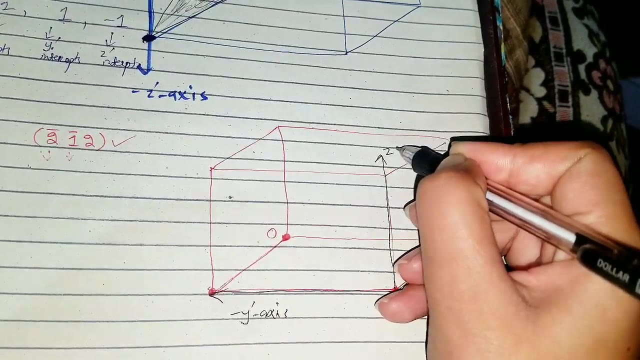 lines are very important in drawing the planes and because we are uh given with the intercepts and intercepts at the points on the axis lines. this is negative y prime axis. okay, this is the negative x prime axis and this is the positive z prime axis, since the z index was positive. so 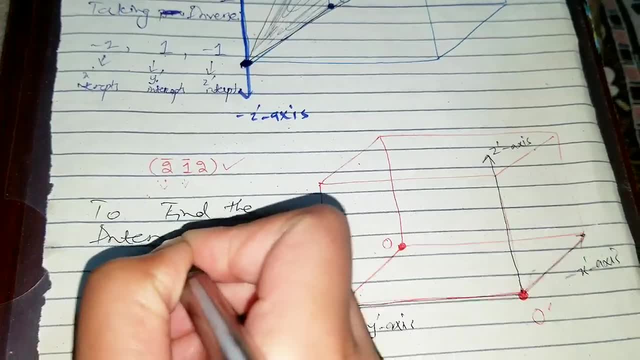 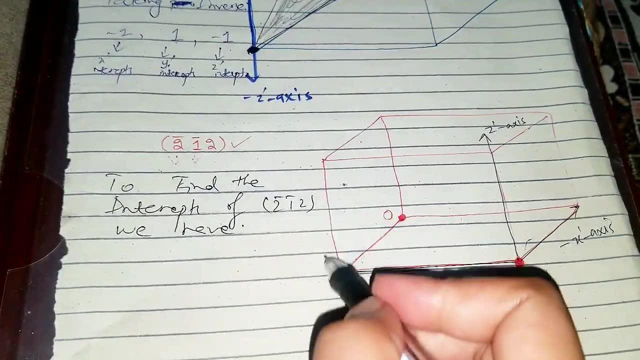 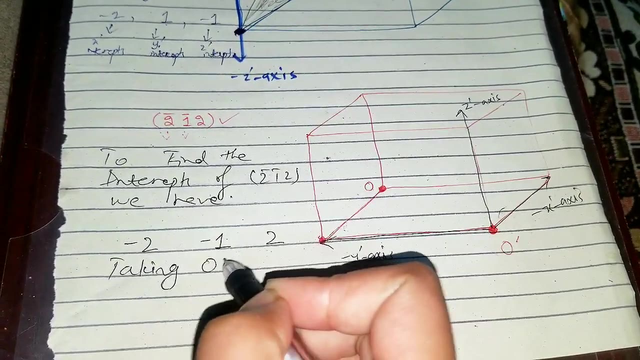 to find the intercepts of 2 bar 1 bar 2, we have to take the inverse of each of the index. you'll write it right there. and these are the three indices. write the operation that you are going to perform on them, which is taking inverse. taking inverse of minus 2 gives minus 1 by 2. 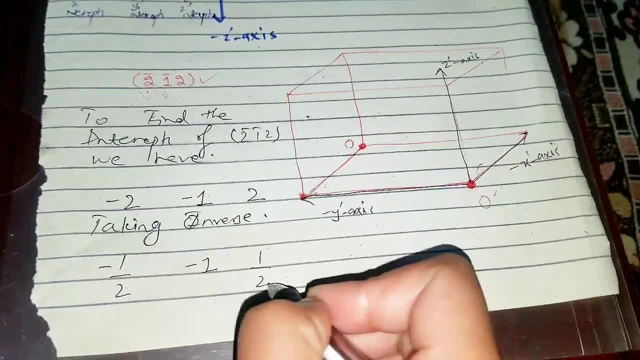 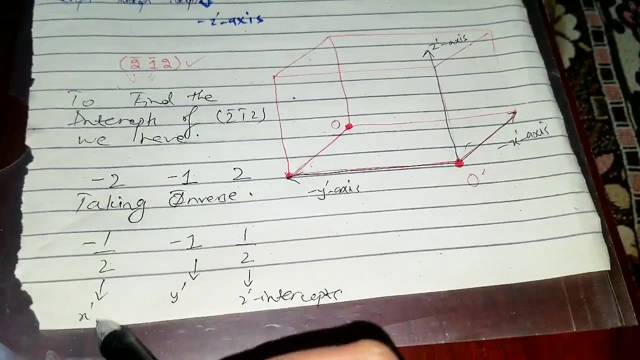 taking inverse of minus 1 gives minus 1. taking inverse of 2 gives 1 by 2. this is the x prime intercept, this is y prime intercept and this is the z prime intercept. these are the intercepts. so x prime intercept is minus 1 by 2. so this is the region, new region. 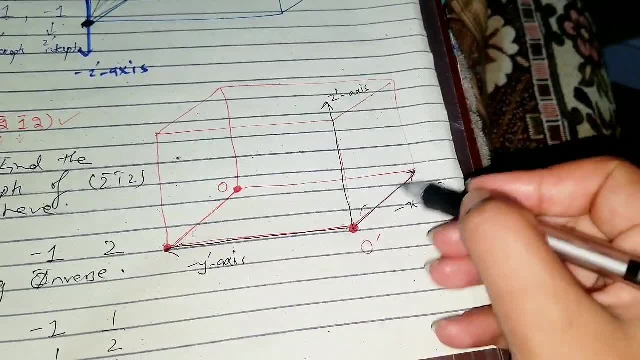 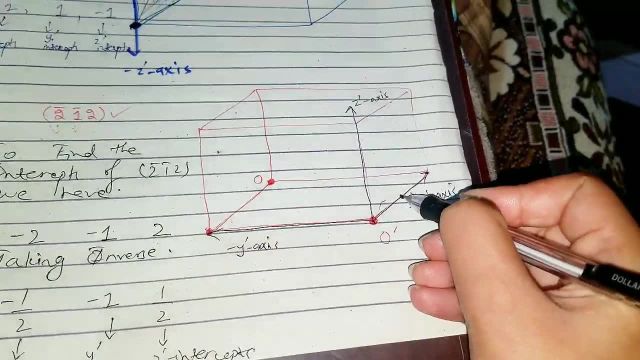 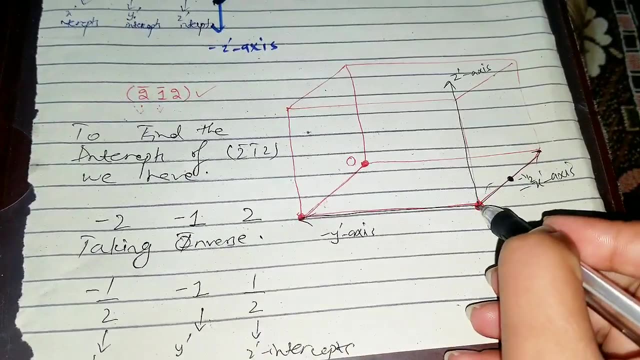 and minus 1 by 2 means this whole length is 1. okay, from one corner to the other corner is 1 and half of it is right there. okay, this is one of the point on the plane. next is y intercept, which is 1 here. okay, so minus 1 here. so from origin, one unit means to the other corner of 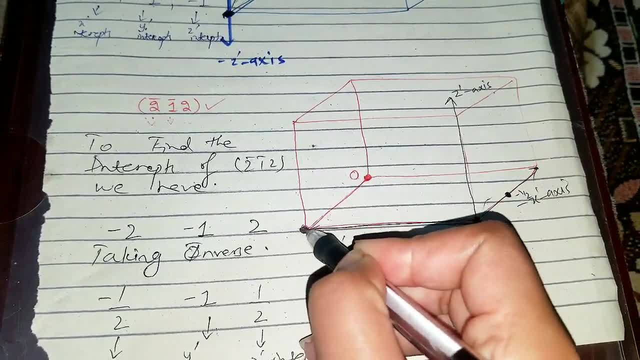 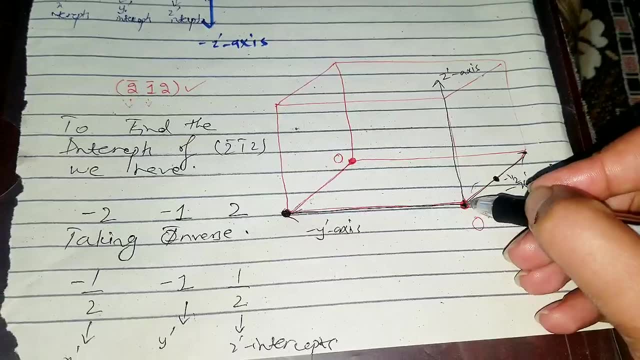 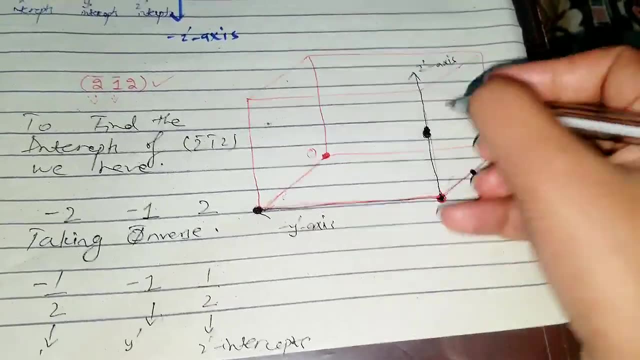 the unit cell along the negative y prime direction, which is this point, this is another point on the p lane- and um z intercept is z. prime intercept is 1 by 2, which means from origin, all over again. 1 by 2 unit, which means the half of it. uh, maybe right there, right there, okay. which is this? okay. 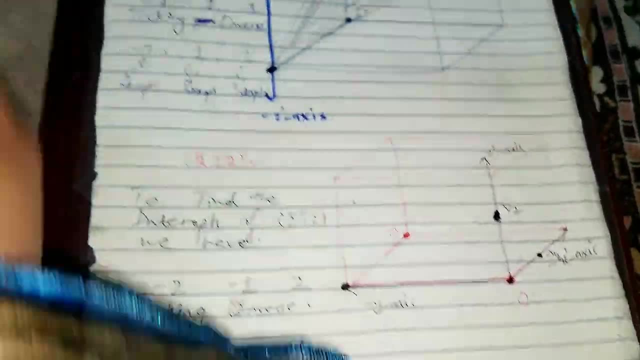 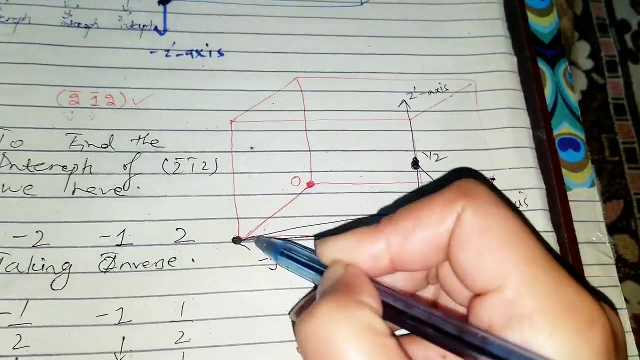 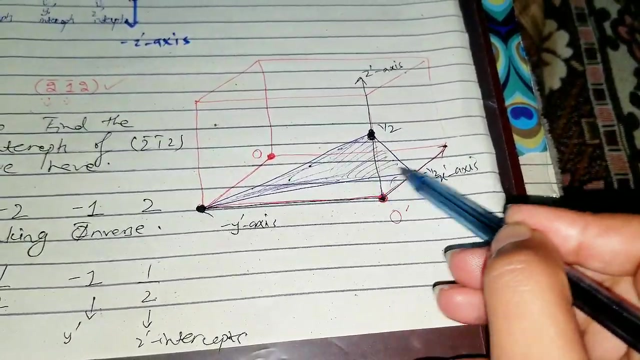 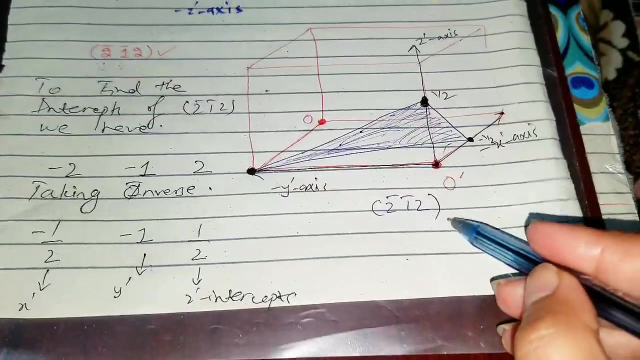 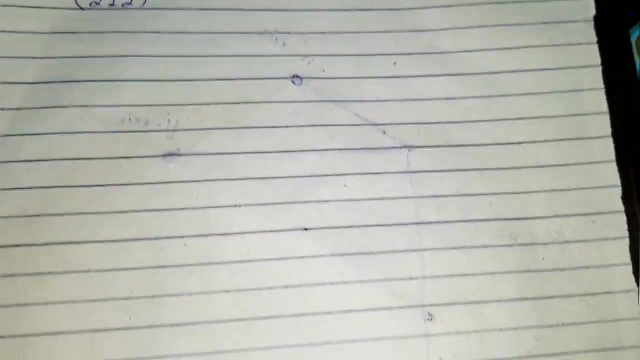 now we'll join these three lines together to get a cute little plane which is obtained like that. okay, so yeah, this is the plane. uh, two bar one bar two. okay, and yeah, this is done now. so here's the last problem that we are going to do. okay, so yeah, this is all negative case and let us draw the cube first. 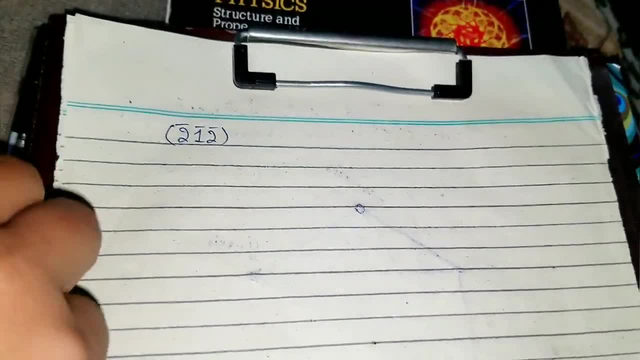 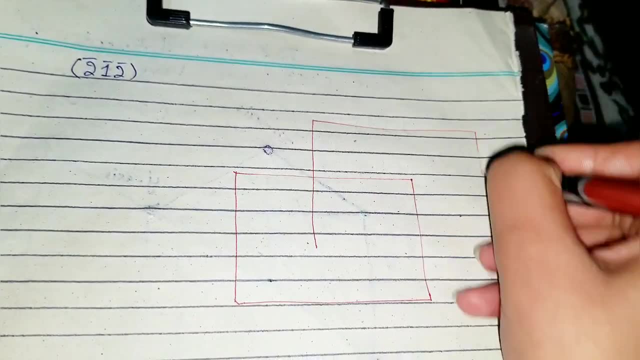 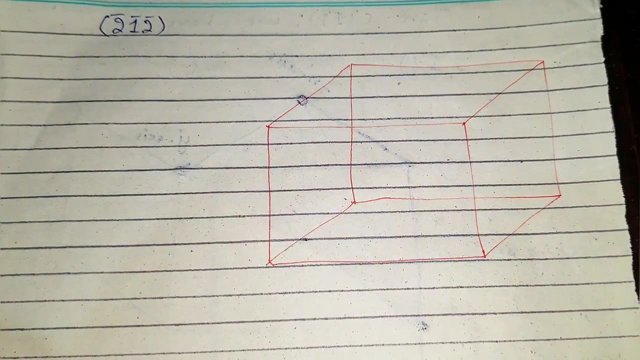 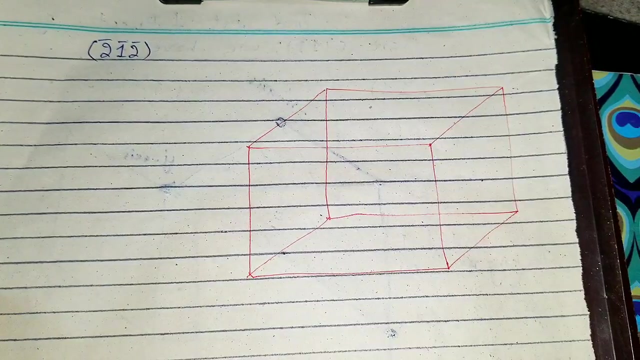 and then we'll shift the region. okay, so this is all negative case and let us draw the cube first and then we will shift the region. okay, so this is the cube and please cooperate uh with me with the background voices, because these are my family members and, uh, they like to speak when i, when i'm 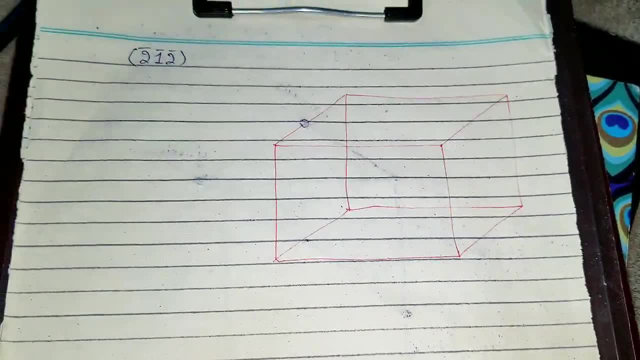 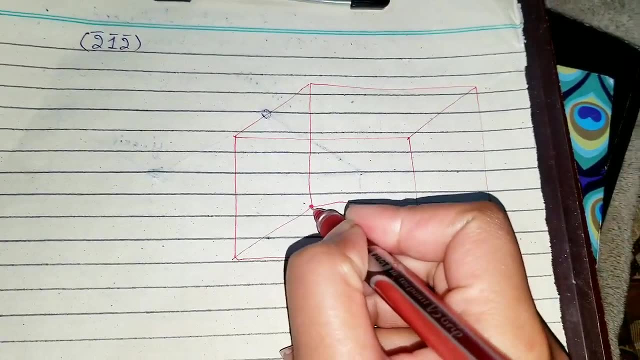 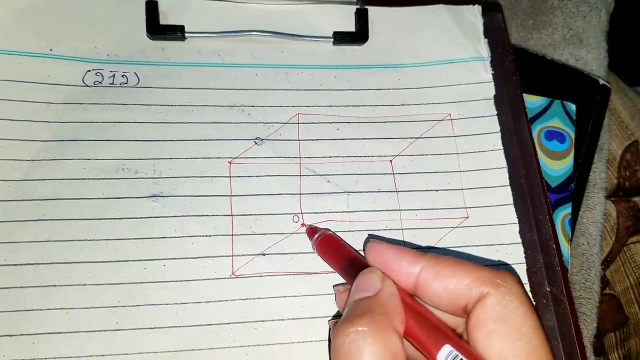 making video, you know. so i can't do anything of them. i have told them to stay silent, but they can't. okay, uh, yeah. so this is the all positive region. let us call it with o. okay, let us call it o. Now, since the x-index is negative, we have to shift the origin one unit along the x directions. 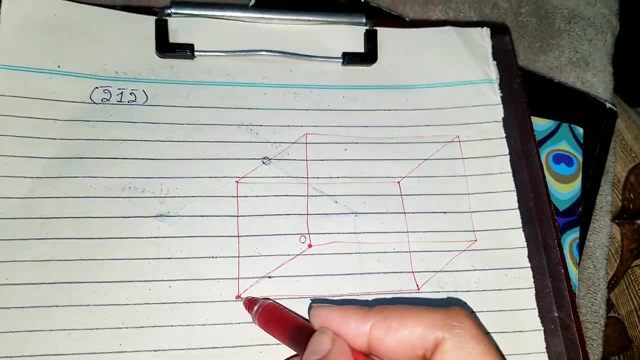 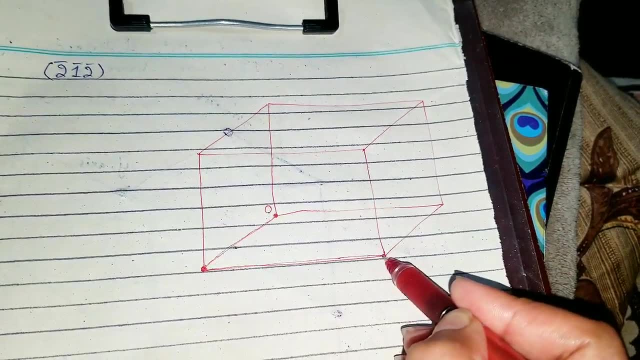 that is this one. now, this cannot be the final origin point, because the y-index is also negative. so from this point onwards we have to shift the origin along the positive y direction, which is this side, to the other corner of unit cell, since these the z-index is negative. 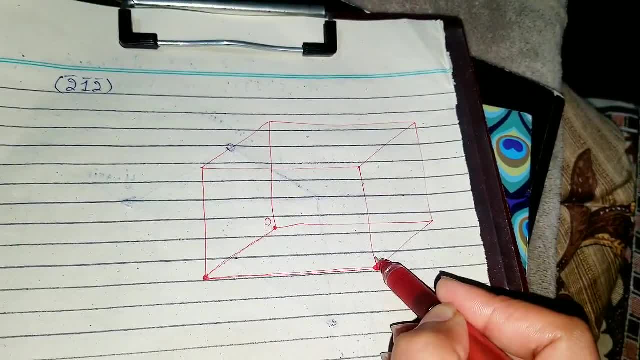 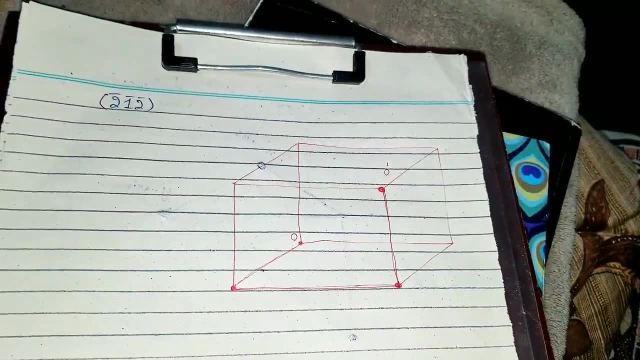 you have to shift the origin onwards from this point along the positive Z direction, which is this, to the other corner of the unit cell, which is this one point. so this is the final origin o prime. okay, and the axis lines are these three lines connecting the origin o prime. 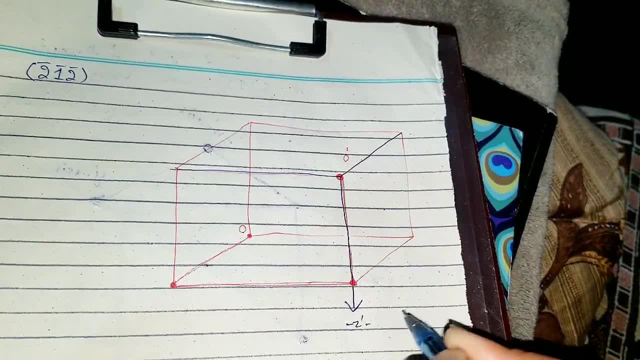 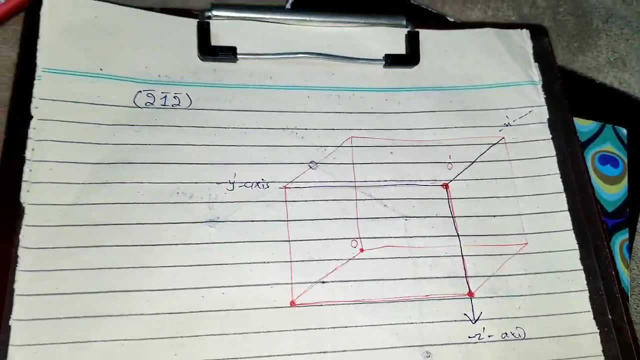 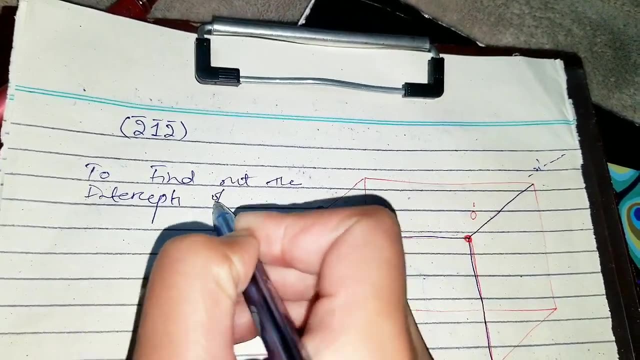 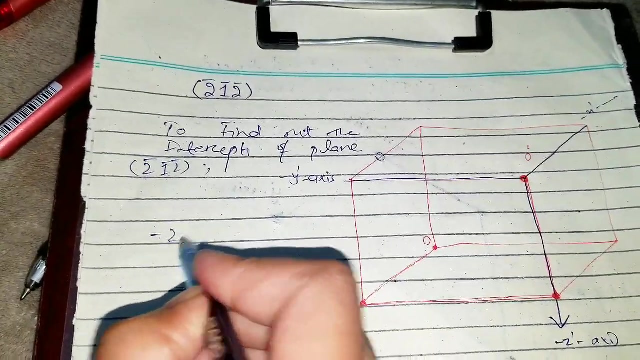 okay, this is negative z prime axis, this is negative x prime axis and this is the negative y prime axis. all right, so to find out the intercepts, the intercepts of p-line, 2 bar, 1 bar, 2 bar, we have to take the inverse of each of the intercepts, so it's minus 2, minus 1 and